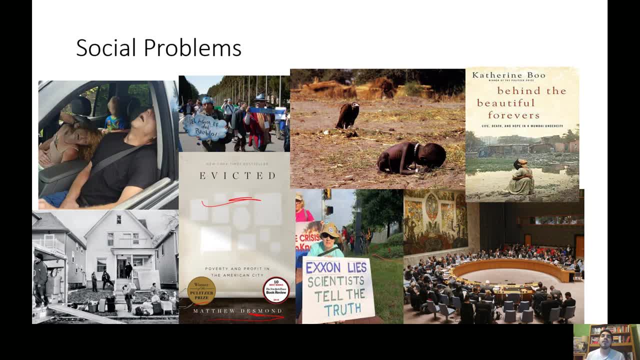 how to roll out material and pitch it to students and make it digestible and stuff like that. So hopefully my planning will allow us to touch these topics Specifically. the goal is to use microeconomics to better understand these sort of social problems and then use these social 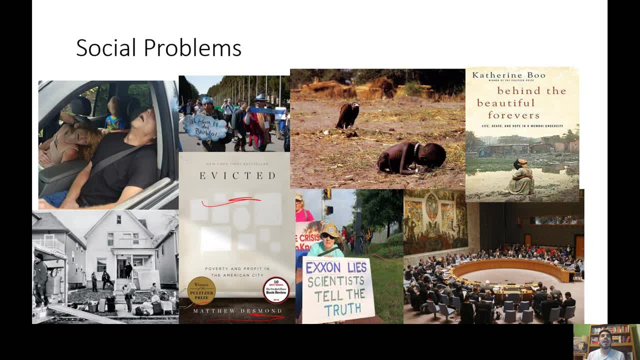 problems, to better understand microeconomics And also, hopefully by the end of it, to use microeconomics to come up with sort of solutions, or our own policy proposals, So to speak, to solve these sorts of problems. We also will be talking about poverty. We're going to be talking about the Washington. 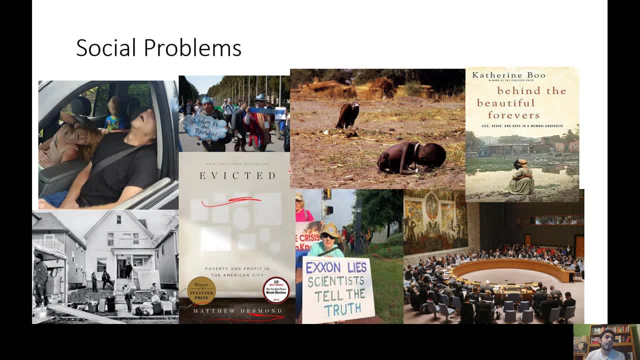 Consensus or the forced privatization of socialist economies and heavy government or economies that featured heavy government intervention and sort of the backlash and the backlash to it. We're obviously going to talk about extreme poverty. This is a really great book by Catherine Boo about Behind the Beautiful Forever. It's about a slum in India. 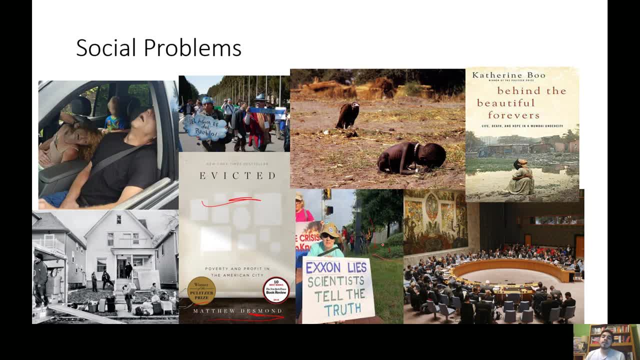 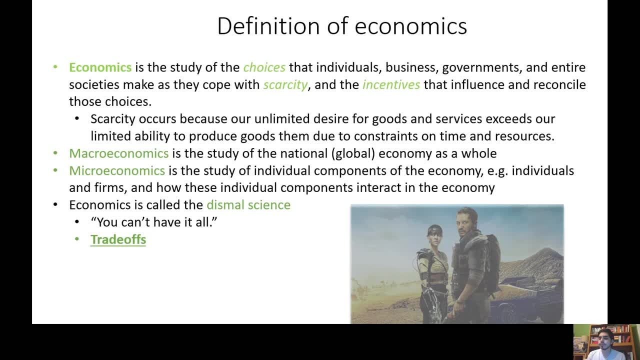 We're going to talk about climate change and we're also going to use economics to describe and explain the behavior of states and countries. So the reason why I presented you with that slide of what we're going to the breadth of the social phenomenon that we will be studying in economics- is because I know that there are a lot of 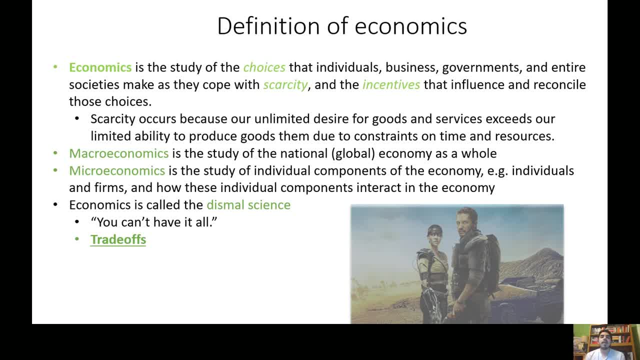 misconceptions about the study of economics. A lot of us think economics and we think financial literacy or dollar bills, and that's incorrect. Economics is the study of the choices that individuals, businesses, governments and entire societies make as they cope with scarcity. 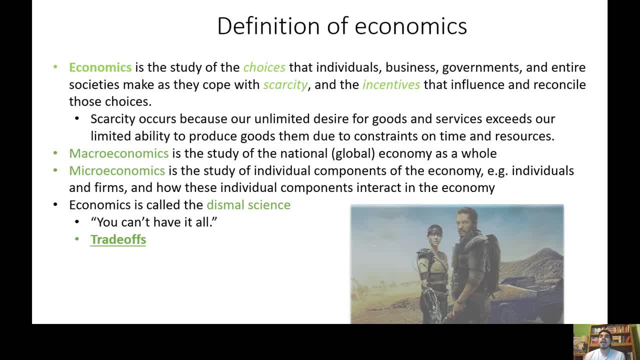 and the incentives that influence and reconcile those choices. So it's how individuals, businesses, governments wrestle with scarcity, wrestle with the fact that our unlimited desire for goods and services exceeds our limited ability to produce goods due to constraints on time and resources. There are two branches of economics. There is macroeconomics. 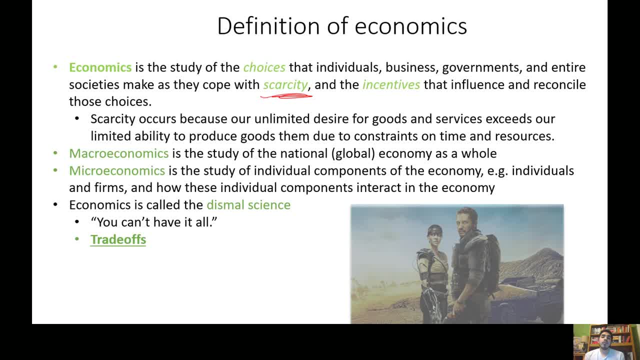 which is the study of the national global economy or the national or the global economy as a whole. So in macroeconomics oftentimes students wrestle with questions relating to unemployment and inflation, stuff that affects the macroeconomy and sort of the policy mechanisms that exist. 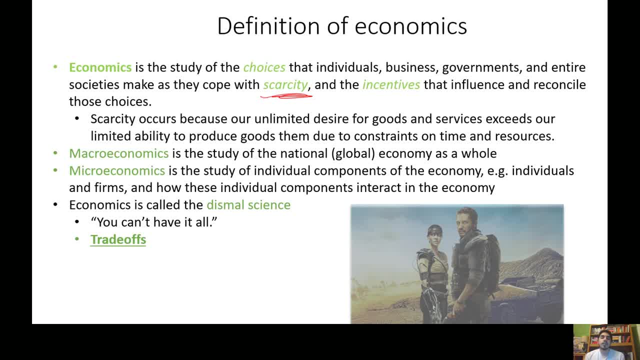 for the government to correct for bouts of low economic growth or even negative economic growth and so forth. Microeconomics, in contrast, is the study of individual components of the economy- uh, individuals, firms, um, and and governments- and how these individual components interact in the economy. 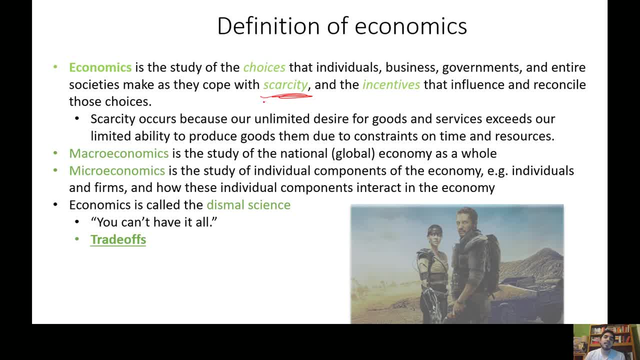 um, economics is called the dismal science, and this relates to this word, scarcity. it's called the dismal science because it tells you you can't have it all, given conditions of scarcity, given worlds of scarcity, and here's the kind of dramatic example of a world of scarce resources. 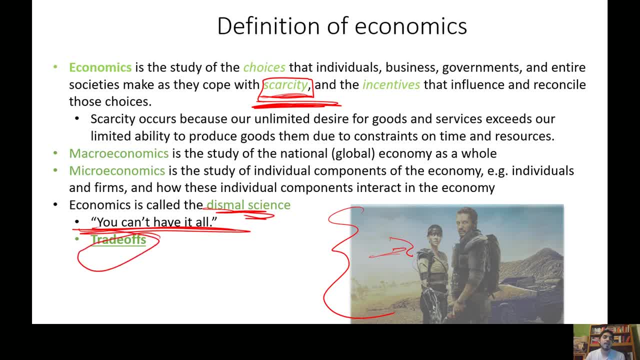 you can't have it all. there are trade-offs to be made, and that there's no such thing. this is a famous line. there's no such thing as a free lunch. no such thing. you're trading off something. you're giving away time. you're giving up something. 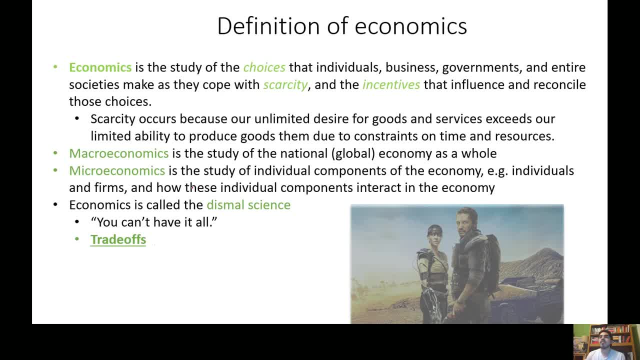 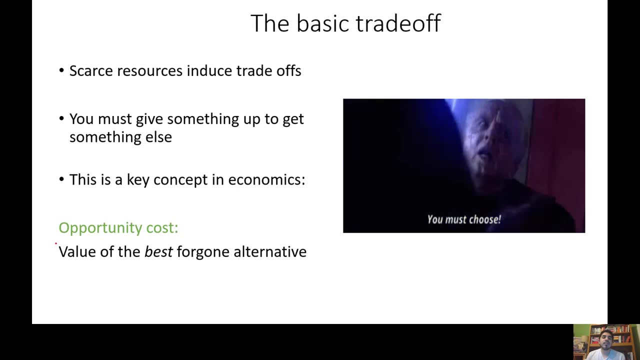 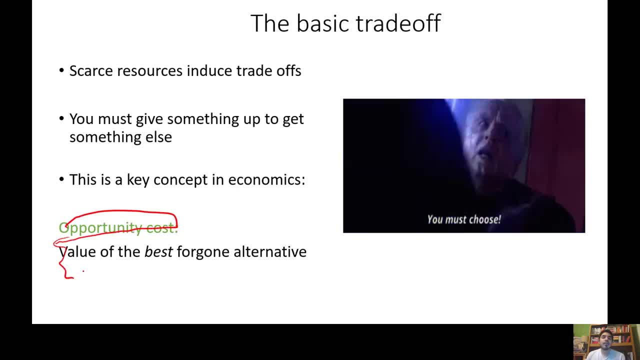 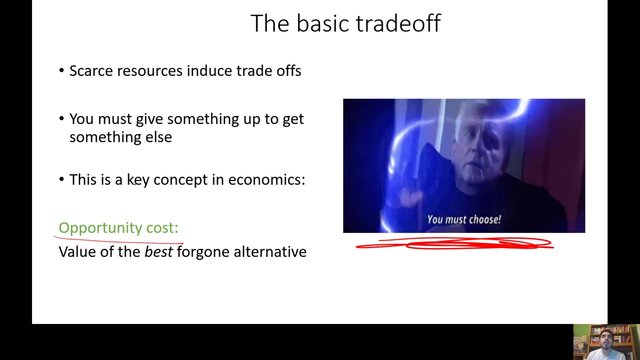 yes, at the beginning, um, but we really kind of to delve. we've delved deep into this. when we started um, drawing production possibilities, frontiers, and here's a picture of ember palpitating. you must choose, that's right. you might think of it as a 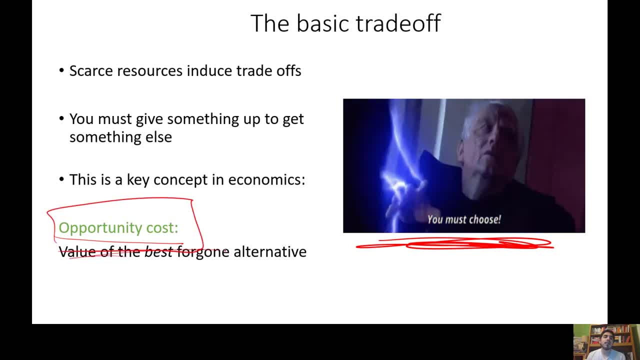 solution to all of your financial- your financial needs, but that's not the case. there are numbers on the Internet that deal with this issue. for example, there's a lot of money in the economy. you can't get a bunch of money immediately and you might not want to have that. 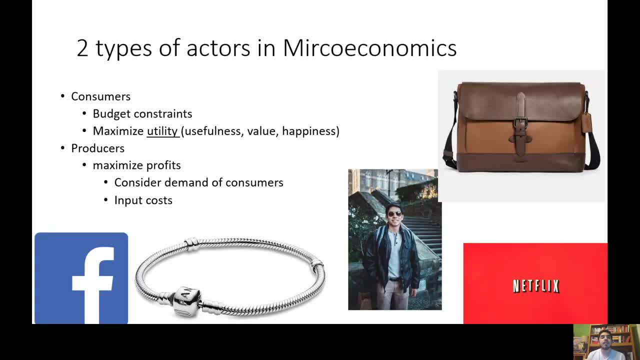 and have to do more and more ends, however, those numbers in the country, as you know, do you just want to buy a bunch of money, in which case you could buy, So we'll talk more about that when we get into production possibilities, frontiers. 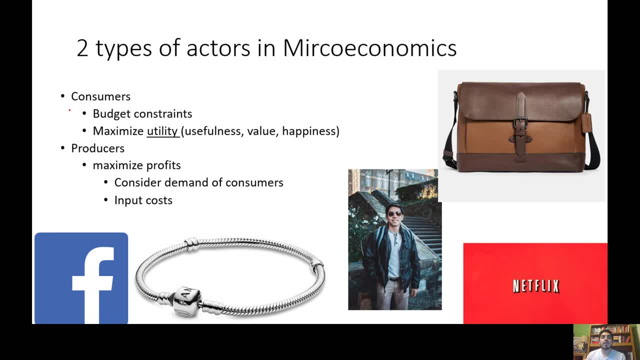 The two actors in microeconomics, and we also said: usually we're going to deal with consumers and producers. We'll talk more about this later. We assume consumers have budget constraints and that they want to maximize utility or usefulness, value, happiness, benefit. 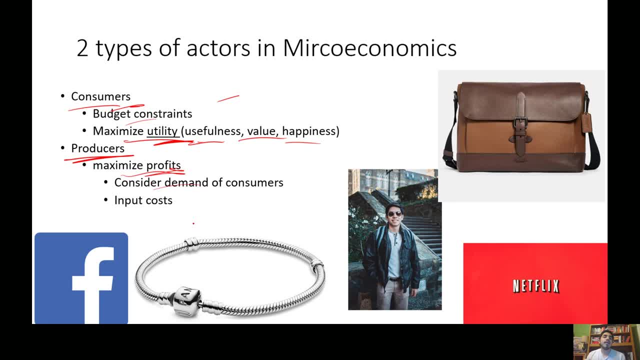 And producers will assume that they want to maximize profit and consider, in maximizing profits, they consider the demand of consumers and input costs. We're also going to add, because we're going to use game theory to describe the behavior of states, governments as well. 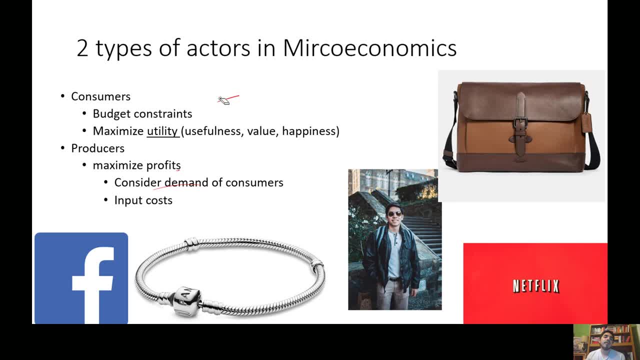 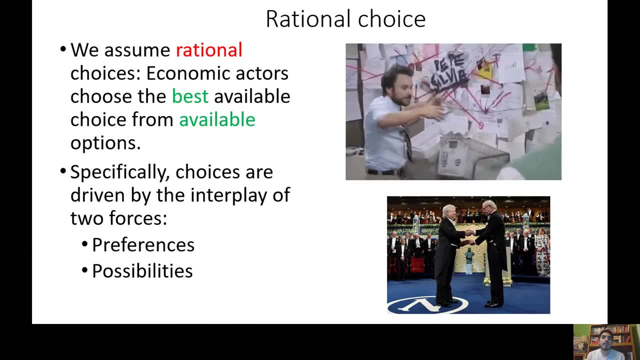 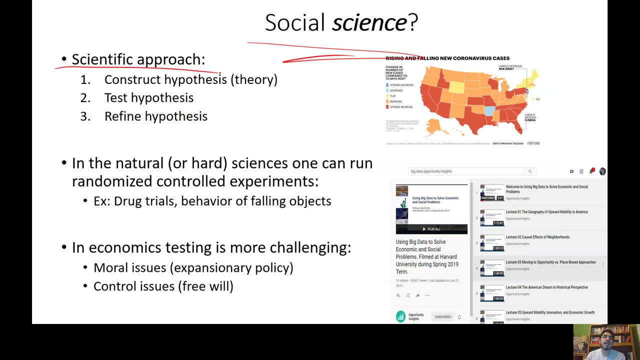 In unit one we also, when we determine comparative advantage, we also we also kind of wrestle a little bit with international trade. This we'll talk about later. We said that economics is a social science because it uses scientific approaches, right? 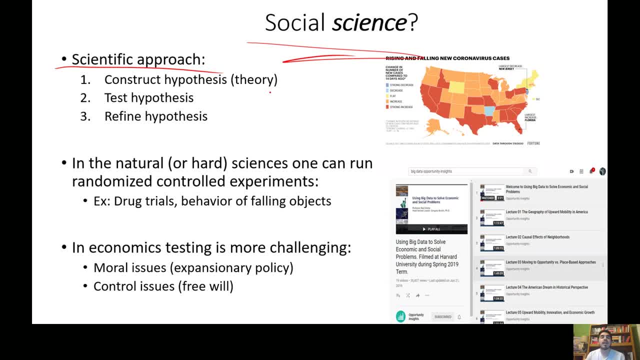 You, an economist necessarily constructs hypotheses. We are going to be wrestling with a lot of theories in economics, a lot of theories that are considered, you know, robust, well supported by the evidence. You have to test yourself, You have to find your hypothesis and refine your hypothesis, but in contrast to natural or hard sciences, where one can run what is called an RCT or a randomized controlled experiment or a randomized controlled trial, where, for example, a drug trial, where you have a treatment group, people that get a specific- so we can imagine the coronavirus vaccine- people that get the Pfizer vaccine and then a placebo group, a control group, or people that don't- 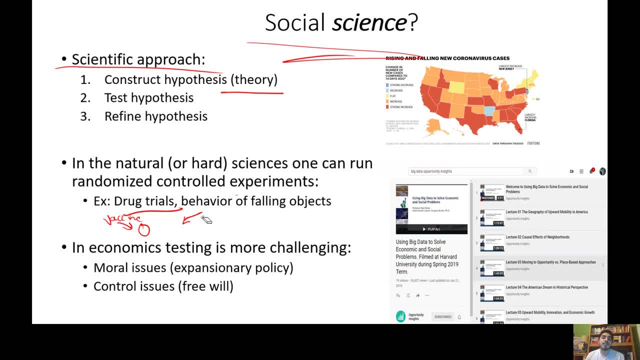 RCTs are much harder to run in economics, So it's a more precarious science- and I'll expand upon this a little bit more in a little bit- And economists are therefore stuck trying to look for natural experiments. right, It's a little bit more precarious. 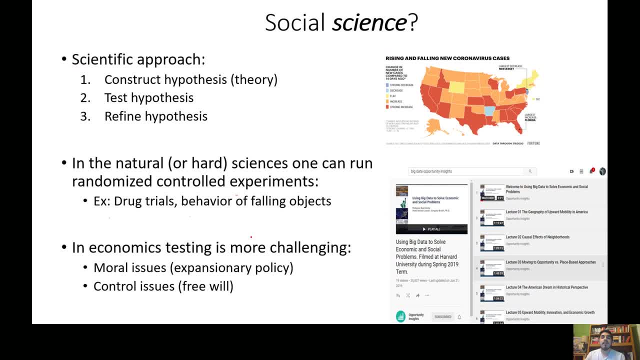 They're looking for natural experiments. They're looking for variations in terms of governmental policy. they're looking for economists. use all sorts of statistical tools that you're learning in ap: statistics, regression, analysis, all sorts of stuff- and they are economists, are looking for natural experiments, right experiments. they're looking to observe phenomena. 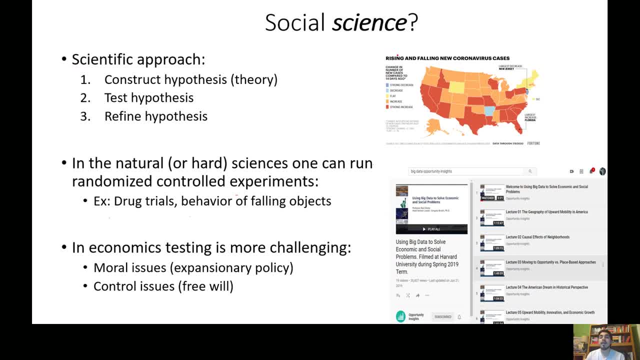 phenomenon, phenomena- i don't know what the plural is- in society and looking for natural experiments, so to speak. and so the reason why i wanted to bring this up is because this is the ap government concept, hashtag apgov. we said this principle of federalism, the sharing of power between this. 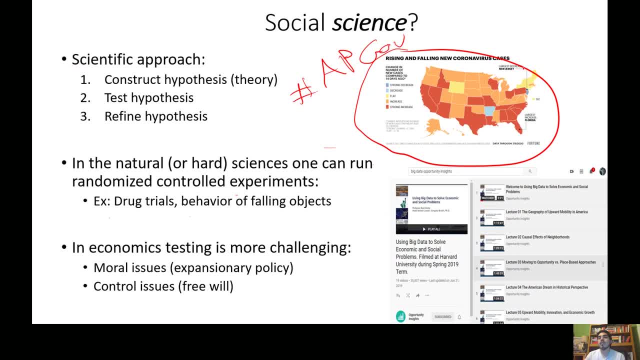 the um, the local governments and state governments and the federal and national government? um can produce inequalities in domains where the powers are reserved for the state governments. so, specifically, an economist might- um, you know, it's particularly an economist might want to study the effects of minimum wage. 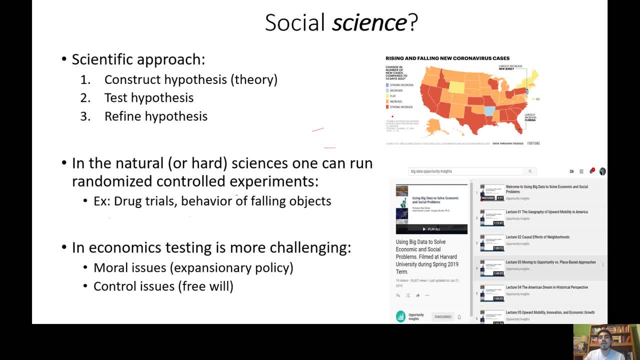 right, the effects of minimum wage: unemployment. and the great thing about our federalist system is that there are different, uh, sorts of wages. right, the minimum wage in texas is what? 750. the minimum wage in washington dc, where i used to live, i think it was like 14 bucks or 12 bucks or 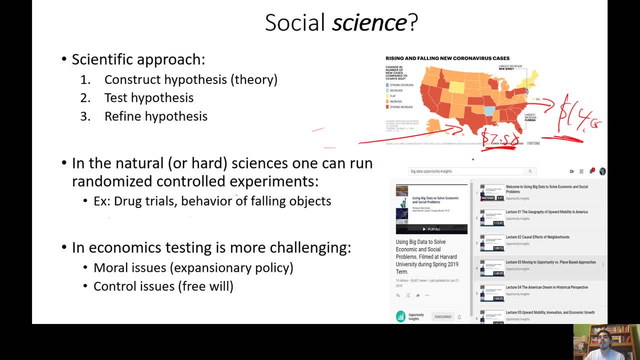 whatever, and so an economist would definitely uh be looking at sort of uh policies that raise the minimum wage. maybe in texas, if there was a law that passed that raised the minimum wage, uh to try to determine what would the effect on output be. and so our federalist 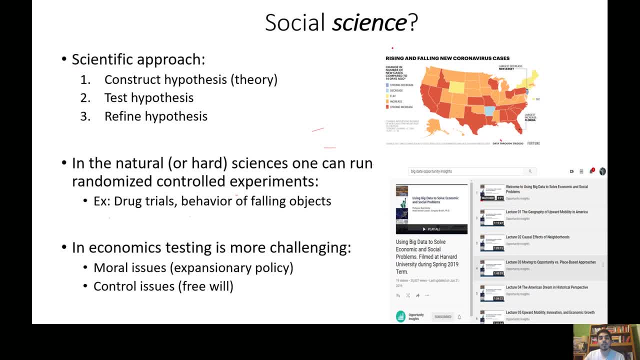 system is actually um very beneficial to economists, um, because it allows them to look for natural experiments within the system. um. one of the things that i also wanted to mention, too, uh, is that in testing is more challenging- or i'm sorry that- um the rise of big data, you know, data collected by 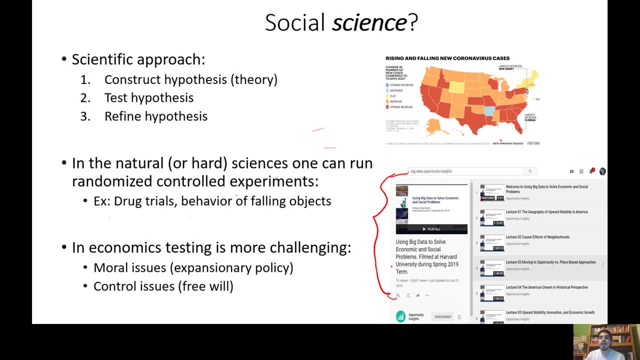 private companies like facebook and google. and then tax record data, national data has allowed economists- economics- to become even more sciency, so to speak. um, there's this great course, um called using big data to solve social and econ, economic and social problems. it's um. you can find it on: 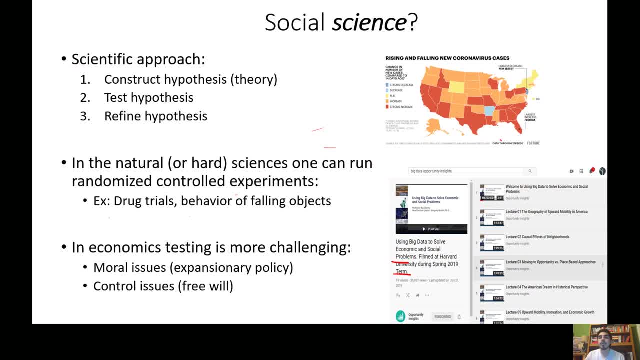 youtube: um, it's taught by raj chetty, who's an economist at harvard university, and check it out, okay, and he goes over like all the statistical approaches. um that, incidentally, uh, miss flores is teaching you so you can use it to help you review some econ and statistics crossover. 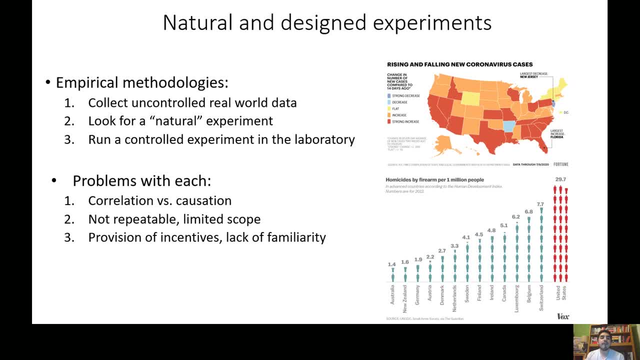 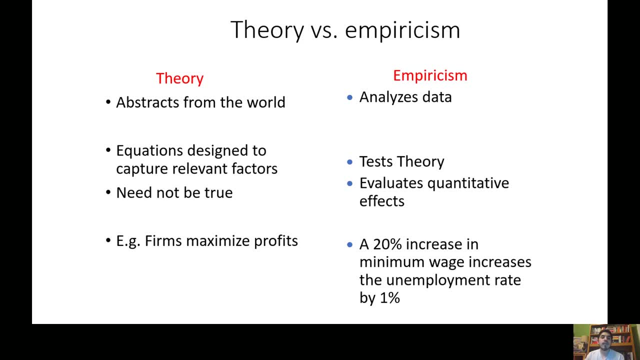 um, we talked about this in class. i don't want to go into this theory. oh yes, so, um, the principles of economics. we're going to be wrestling with a lot of microeconomic theories, um, and we're just going to explain the theories, right? um, we're going to use a lot of. 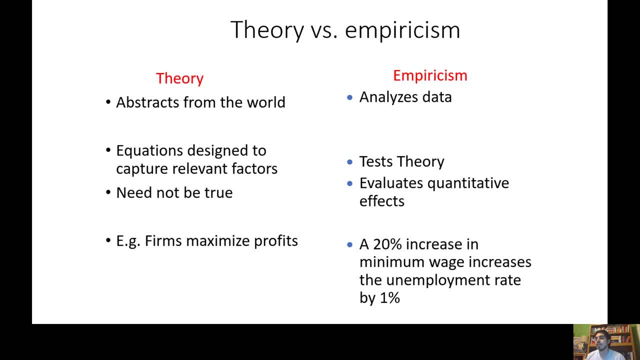 models. uh, to kind of show you, really like, the essential principles of microeconomics. what are um, the sort of um, what's the logic of of microeconomics, what is sort of considered robust and um, the reason being um that lag is based onHHOI term and um. 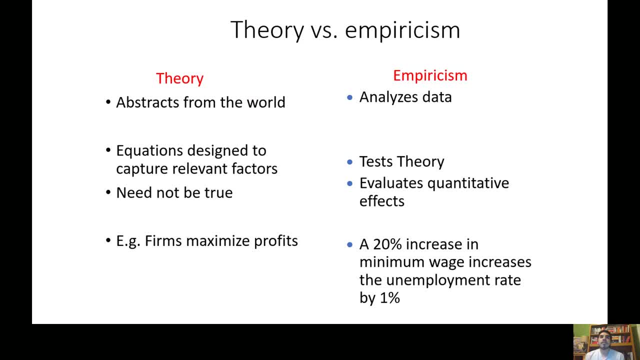 um, it's very much introductory level right. you're not expected to use, um a bunch of like the sort of statistical and mathematical tools that you can expect that you would need to use if you're an economics major and you're taking econometrics, right. um, so we're not going to really focus a lot on empirical analysis. we're 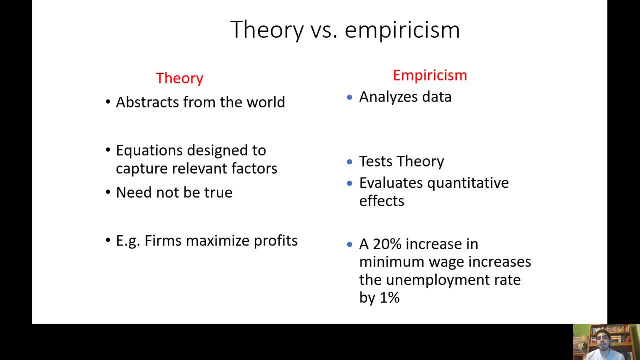 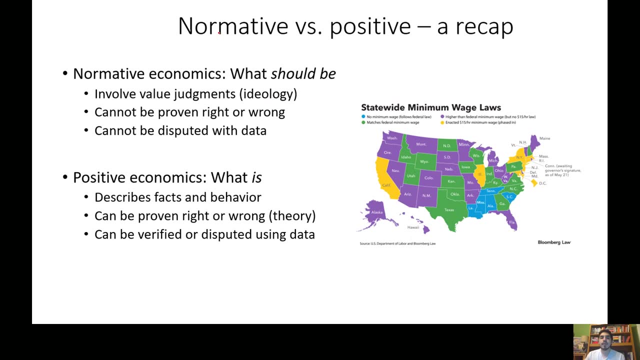 a lot of the theory that has come to us, you know, after economists have wrestled over time with intense theoretical debates predicated on empirical data. But yeah, just know that. OK, this is the first big thing that you probably need to know. 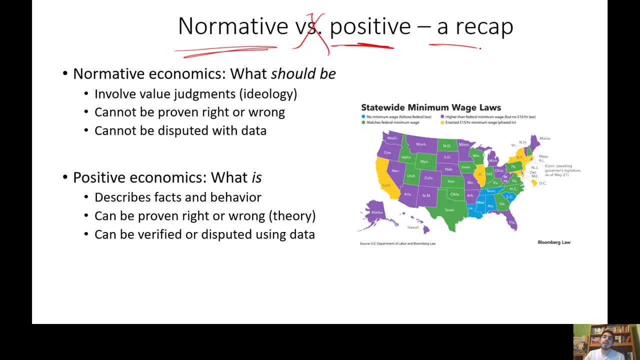 This should be a V, Normative versus positive. This is a recap, So normative statements and we can distinguish between statements and it doesn't have to be normative statements Solely in economics. normative statements anywhere or questions describe what should be or ask what should be. They involve 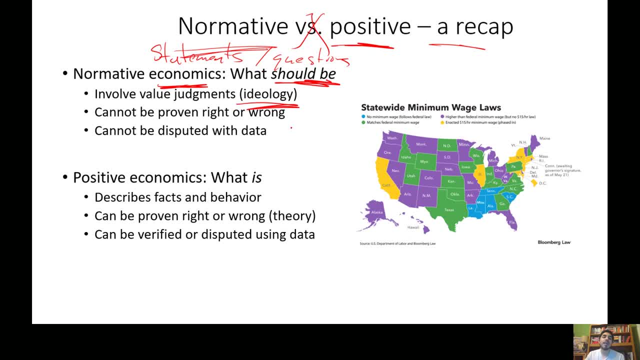 value judgments, so they might be influenced by ideology. They cannot be proven right or wrong and cannot be disputed with data. So an example of a normative question would be something like: what should The Minimum Wage B The Minimum? 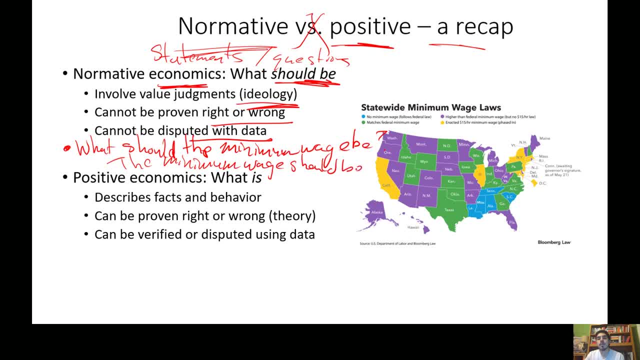 Wage should Be 15 an hour. So normative and positive statements and questions. they are often often kind of a little bit more complex than the common, kind of times You know it's hard. or there are often kind of times You know in in economic paper, assuming in a world where you're 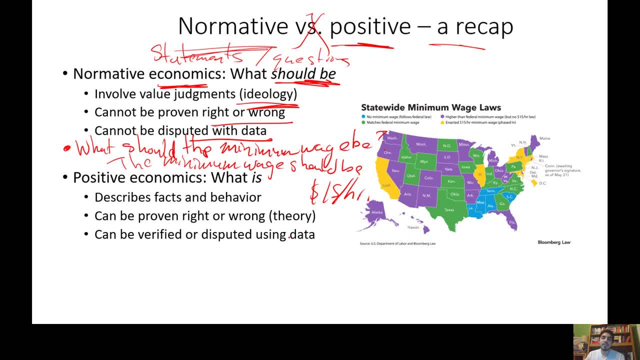 going to Georgetown University major in economics. actually, let's say you're going to Princeton major in economics. Normative and positive statements You can find a bunch in in an economic paper and economic analysis. The interesting thing about the economics profession that we 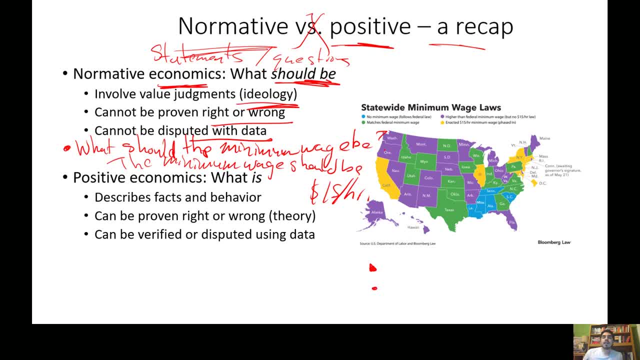 also said a lot about is the economics profession. It's not a major. The economics profession is very much seen as very prestigious. We talked about how it's one of the most pop economics, one of the most popular majors in the Ivy League. 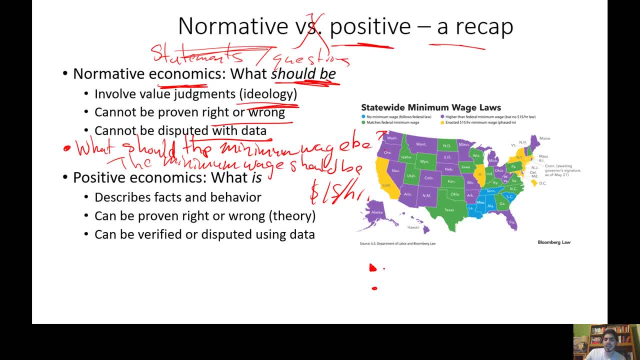 If not the most popular major in the, yet probably the most popular major in the Ivy League. But there is a Council of Economic Advisors that advises the president in terms of creating policy. There is the Federal Reserve Board, which isn't necessarily which control. 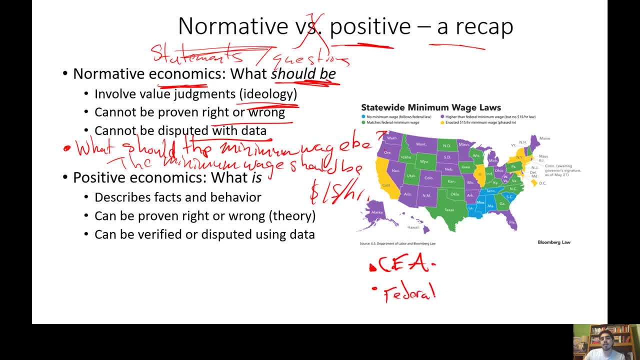 interest rates and have a dual role in the economic process. So there's a lot of discussion around that. There's a lot of discussion around that. We have a dual man. We have a dual mandate that our Reserve Board or central banking system in our 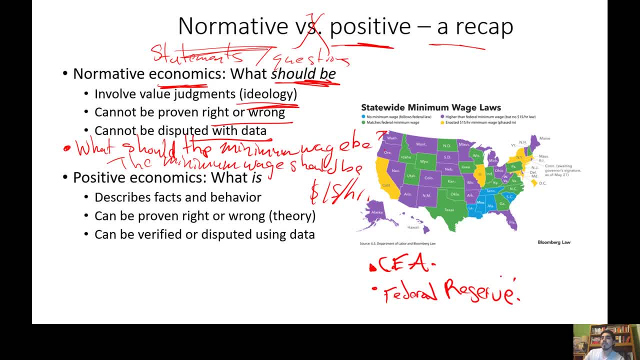 country which is tasked with keeping inflation under control and keeping unemployment below a certain level, And they do this by lowering interest rates and the mechanisms that they use to lower interest rate. That's that's AP, microeconomic stuff, or macroeconomic stuff, And we also have, of course, this: 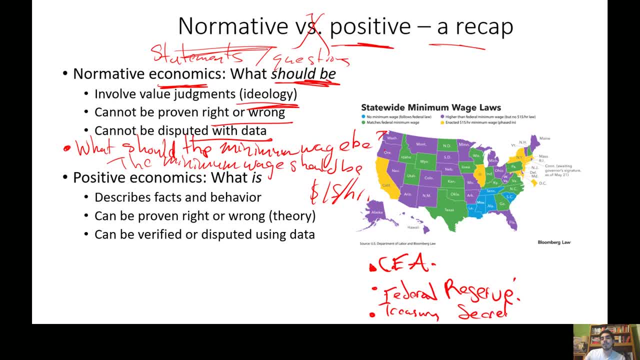 Treasury secretary, And you know, these offices, With the exception of the CEA, don't necessarily need to be manned by economists, but they often kind of are like the bureaucracy is comprised of a lot of economists. They have huge influence in terms of policy making in the United 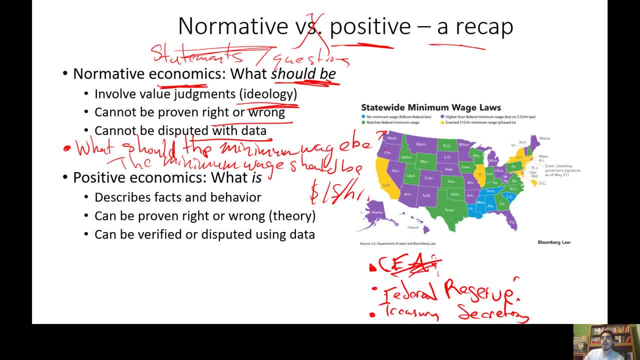 States, The Council of Economic Advisors. the chair of the Council of Economic Advisors has the president's ear in terms of economic and social policy in the United States. Having said that, Um, there is a sort of In economic papers, in economic reports, there's a lot of. 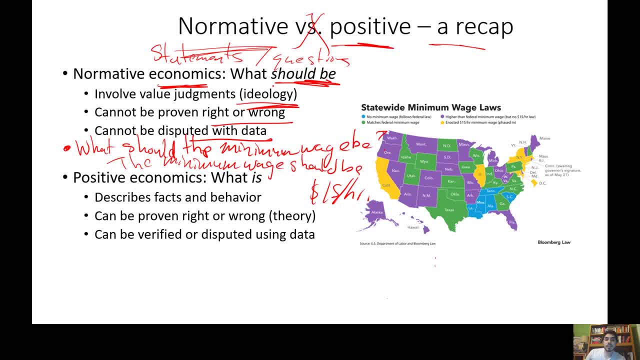 reports, maybe government reports. There may be a collection of normative statements about what should be, what should happen, and there also may be a collection of positive statements that are imbued within the same sort of paper right. So there may be positive evidence and positive 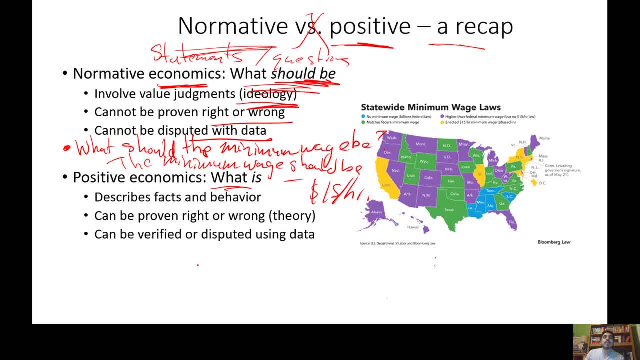 statements that are meant to support normative statements and claims or to help us answer normative questions. So an example of a positive statement could be about the minimum wage or the minimum wage, And then there's also a collection of positive statements- The minimum wage. 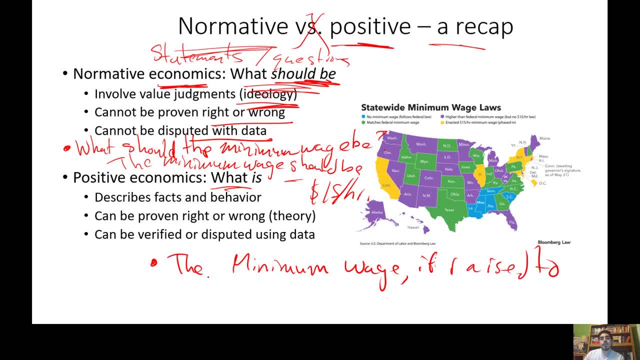 If raised to, Would Decrease Employment In the Retail industry By X percent Right, and so this positive statement would need to be supported by data. Obviously, an economist would try to support this positive statement. They're making this positive statement. 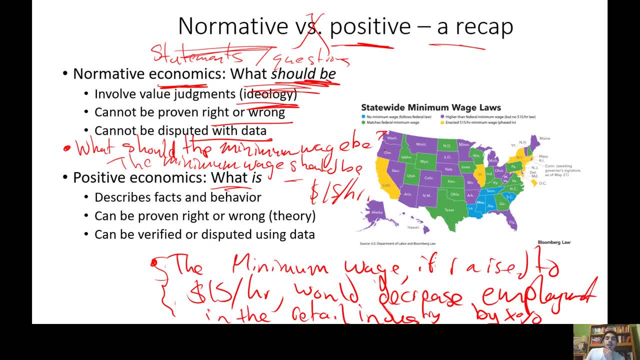 with their data and their in their sort of model. but But for our purposes, this positive statement doesn't necessarily have to be true. right, Doesn't necessarily have to be true. You could dispute it, because we said that economic economics is very much. 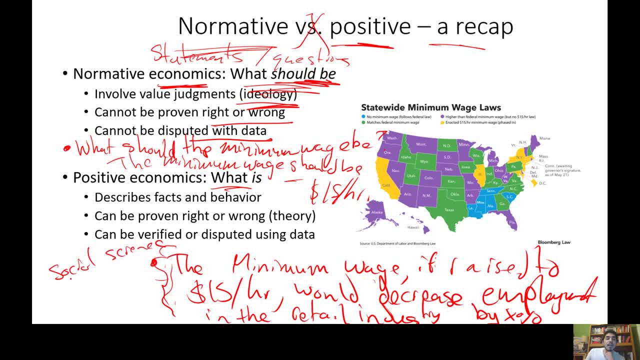 A social science but unlike a hard science where you know there are, there's a considerably more met, There's a considerably greater measure of certainty in terms of things. For example, the law of gravity, you know, is pretty certain. a negative 9.81. 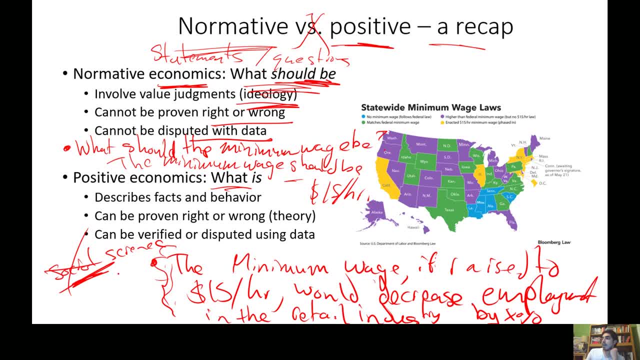 meters per second squared, or or, or, or- or- did I get that right, I don't know- But a social science and there's a little bit more evidence to support that, but there's a little bit more evidence to support that. So I think that's a good question. I think that's a good. 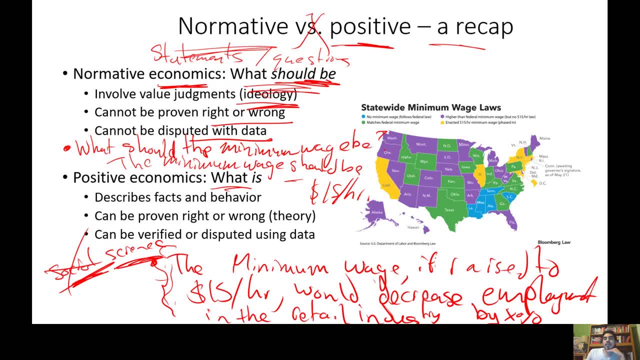 question. So in terms of the real world science there's a little bit more ambiguity because naturally social scientists have to include a lot more assumptions in their sort of models. They, you know it's harder to predict society. why phenomena? you know the data. it's harder to causal inferences. 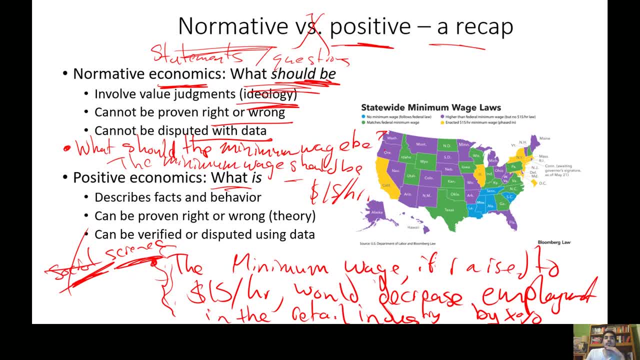 is very difficult. We can use a variety of statistical tools to try to determine causation. an we want to make sure that we're not confusing correlation with causation. with causation There's a little bit which is is is very hard and all sorts of stuff. 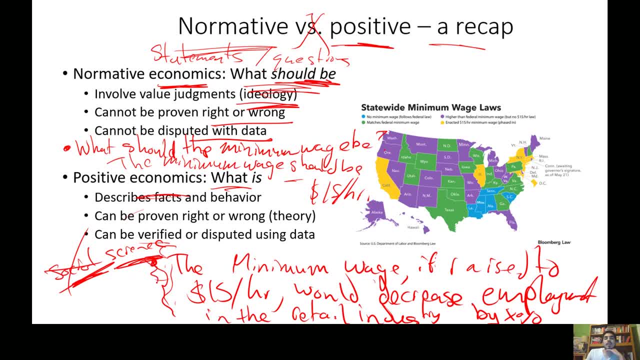 So positive statements in economics certainly can be disputed. There are all sorts of arguments that are happening in economics and really in all sciences too. that take place because science is very much an intellectual and practical activity That involves, You know, oftentimes disagreements and and 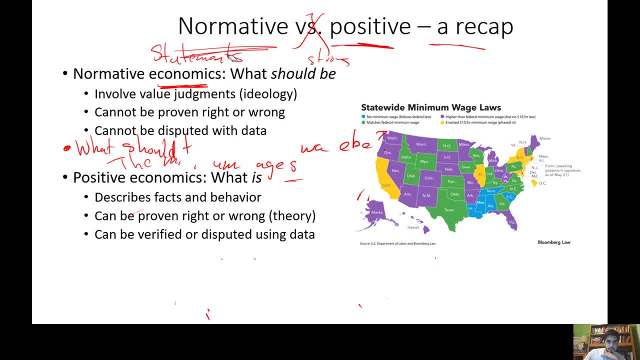 eventually, hopefully, consensus. OK, But the positive statement that you create here is in theory, for an economist Might support your normative statement on economists. I might also just make that positive statement and then might not offer issue any suggestions or policy recommendation, but certainly an. 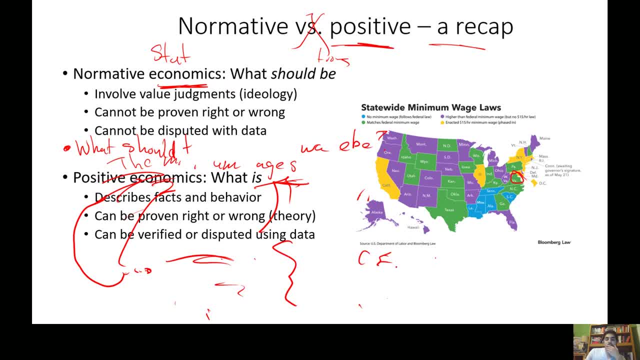 economist at the center or the CEA, The Center for Economic Advisers in the White House. Certainly they're expected to make a lot of normative statements and to support him with positive statements, And sometimes you know, the president has a lot of normative values and that goes. 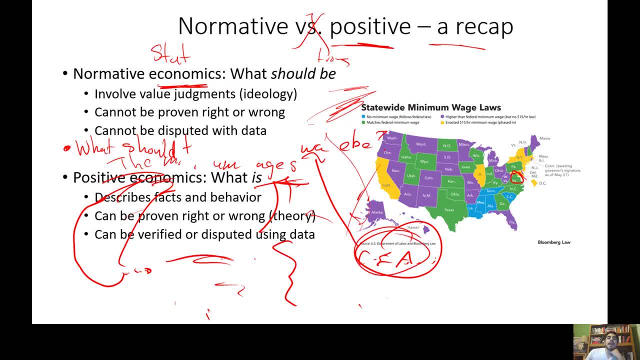 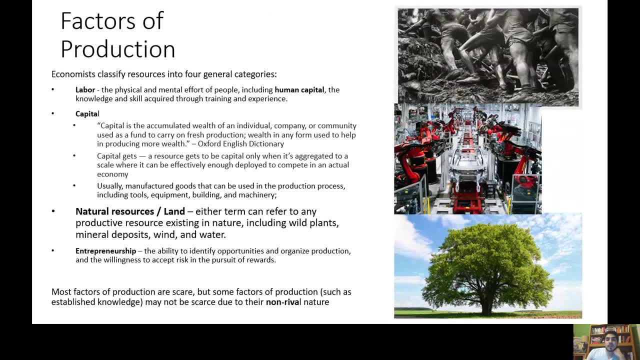 into the selection of the specific economist that chair the committee. So that's something that we look at in the CEA and that obviously influences data collection and stuff like that. OK, Factors of production. Go ahead and take up or pause the video. 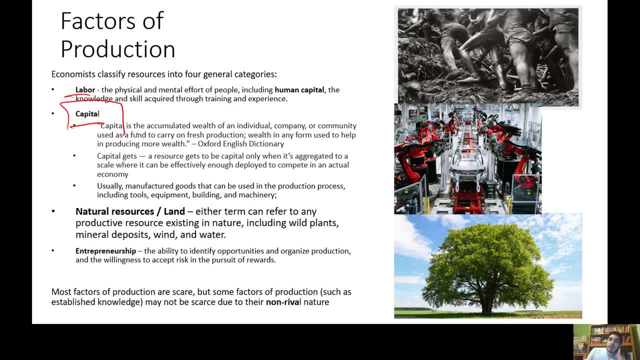 Remember the different factors of production. This one is very important. Capital is the wealth used to create other wealth, and we said that specifically, it's wealth that needs to be scaled to a certain degree to be able to compete in an actual economy for us to be considerate capital. 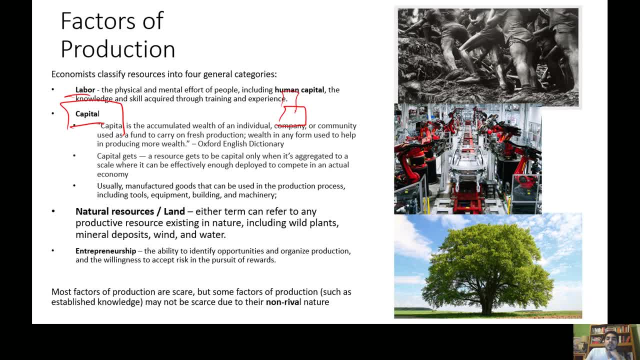 And so you can think of it as wealth used to create other wealth. You know tractors, maybe trailer trucks. you know carrying different goods and services. you know bank deposits, IPOs, all sorts of stuff that can be considered capital natural. 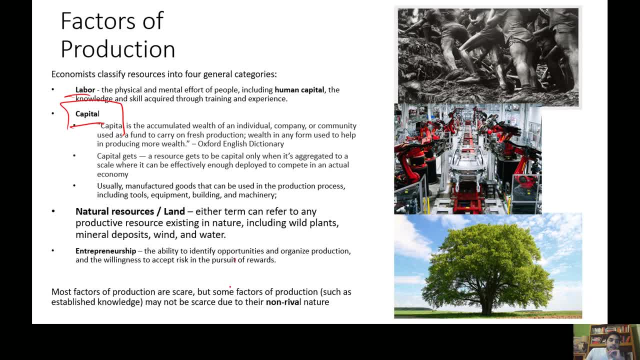 resources, land, entrepreneurship, all that good stuff, all that jazz. Most factors of production are scarce, but some factors of production, such as established knowledge, may not be scarce due to their non rival nature. I'm not going to go into this, but just read the slide. Take a. 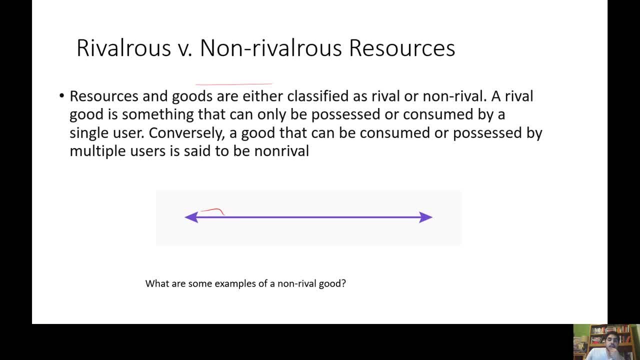 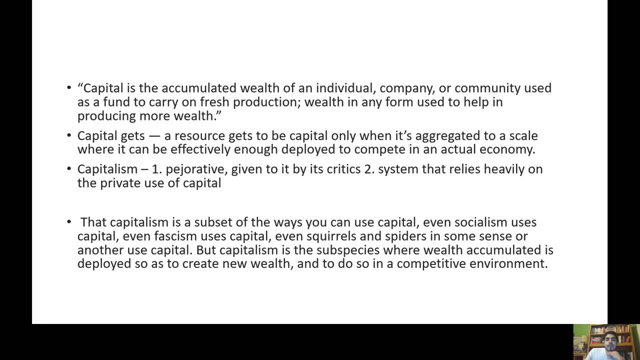 picture Difference between rivalrous versus non rivalrous resources. We're going to come back to this when we get into public goods at the end of the course. Again, we said: capital is accumulated wealth of an individual company. Wealth in any form used to produce more wealth. 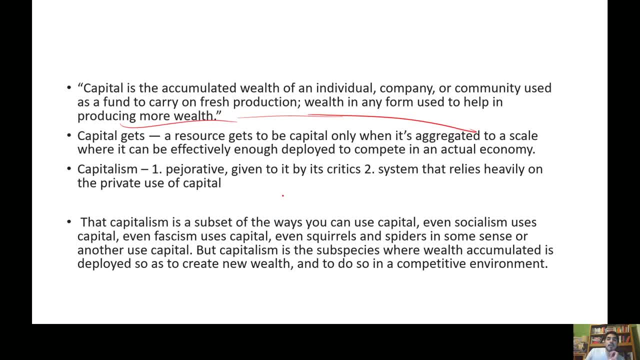 Wealth used to create more wealth. scaled to a certain degree, Yeah, Capitalism- and this is something that I wanted to distinguish early on- capitalism is a pejorative meaning. it's actually a negative term given to it by its critics, right? So? 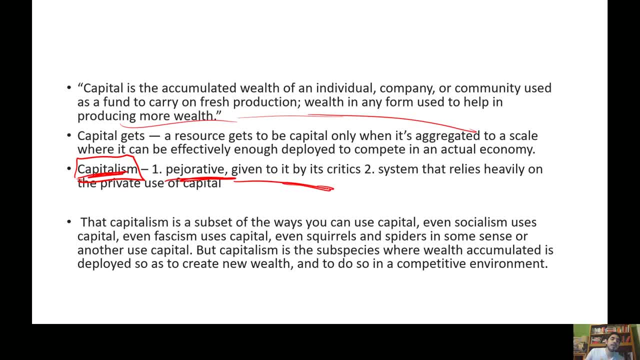 we oftentimes associate capitalism, we use it interchangeably with free market economics and stuff like that. But capitalism describes a system that relies heavily on the private use of capital. So the private ownership of the factors of production, private ownership of capital, I should say private ownership of the factories, private ownership. 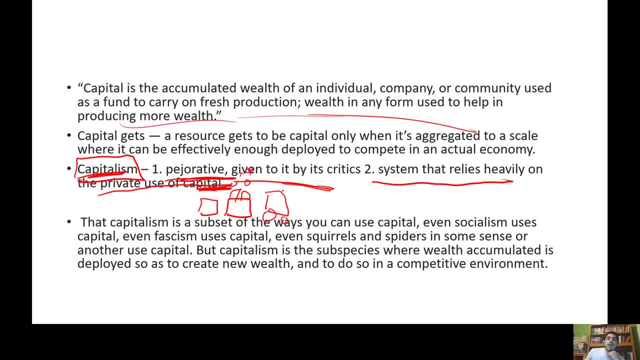 of the steamships of the railroads. So you know, the term capitalism was used to describe a economic and political system that critics that developed in during the Industrial Revolution, that critics, you know, wanted to disparage and, in a sense, stuck. 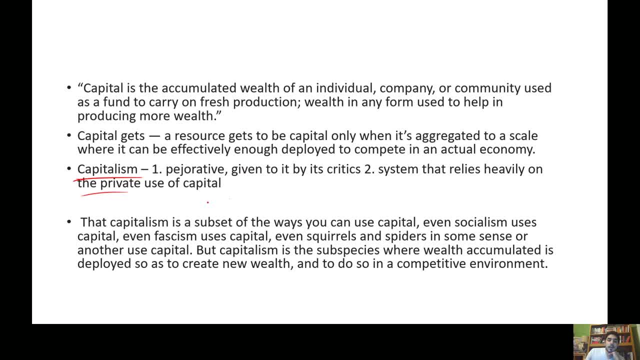 Now people call themselves capitalists and they identify as capitalists, But the thing is, this is not a good stuff. Capitalism need not go with democracy, nor cap, nor democracy need not, or nor capital itself can be, can be used in the creation of our capital itself. 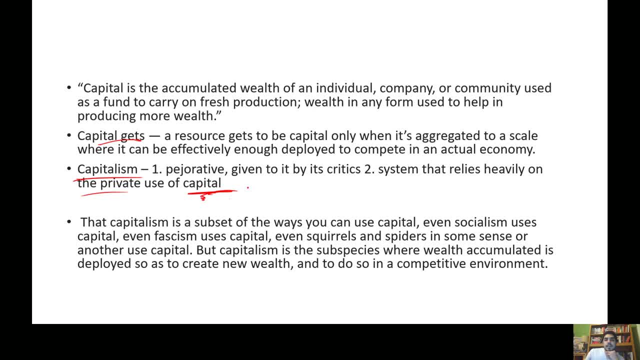 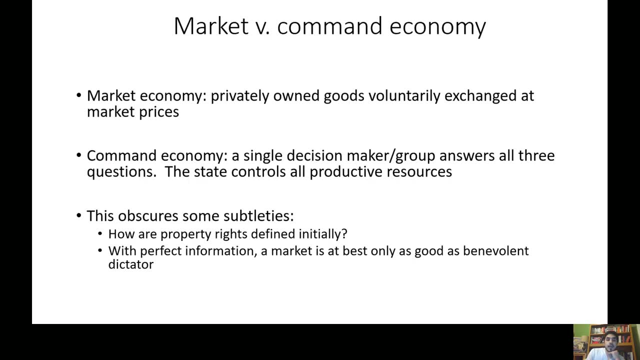 I'm sorry. capital itself is used by fascistic societies, socialistic societies, all that store stuff, wealth used to create other wealth. But capitalism- this is an important distinguishment- just describes a system that relies heavily on the private use and ownership of capital. Okay, cool, We'll talk about the distinguishment. 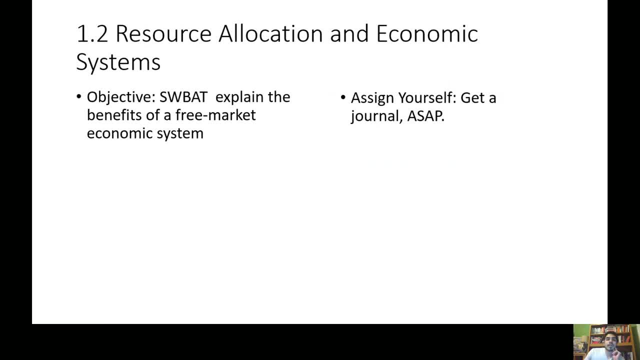 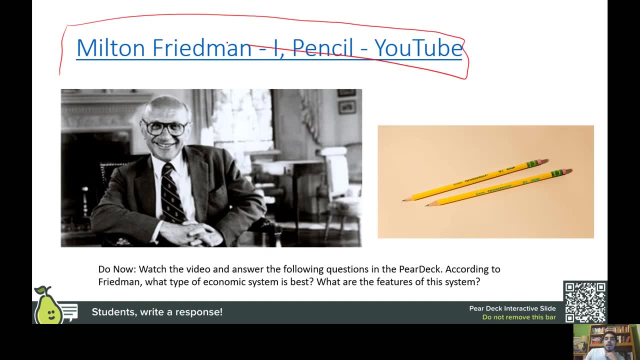 between market economy and command economy. later This gets us into resource allocation and economic systems. We watched this really lovely video by Milton Friedman. Milton Friedman is a Nobel Prize winning economist that was very influential into the economic thinking of Alan Greenspan and Ronald Reagan. He really is trying to talk a lot about and Milton Friedman 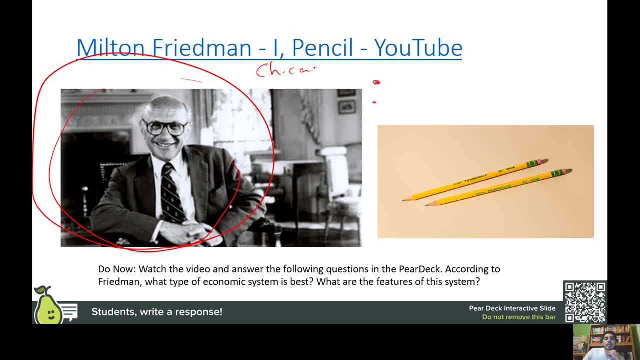 is what is called. he's in the Chicago School of Economics. The Chicago School of Economics are people from the University of Chicago, famous economists, that oftentimes are really, really pro-market, pro, pro, pro-market. We'll see that the market can do a lot of good things. The free. 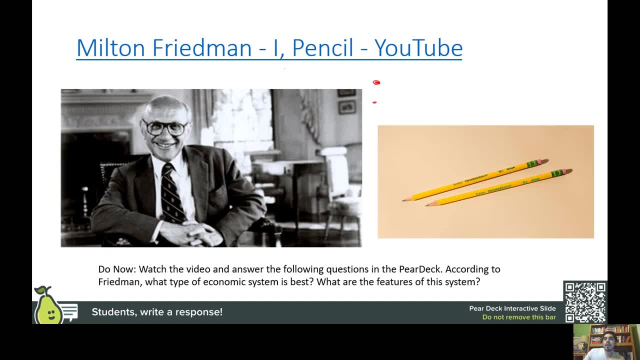 market, I should say, can do a lot of good things. The free market can do a lot of good things And we'll kind of try to. I'll try to spell out the logic a little bit in this video, but I don't want to spend a lot of time on it because I want to reserve the majority of the 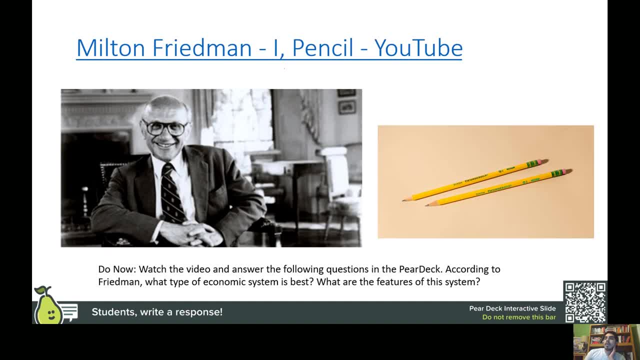 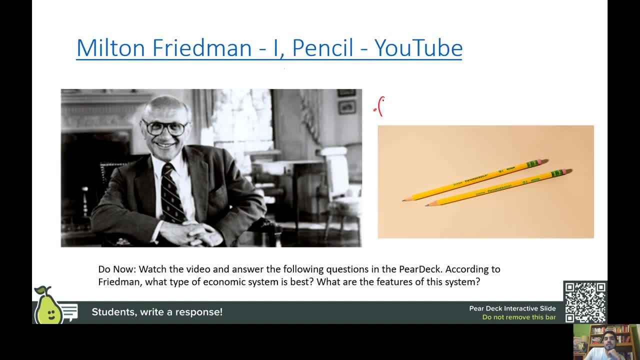 You know, Mutz and Friedman did talk and he kind of suggested that the free market, which is often used synonymously with capitalism, which is okay. he talks about the pencil and he talks about the different inputs and the different people that are involved in the creation of pencil: the graphite, the wood, the paint, the eraser, all of that. 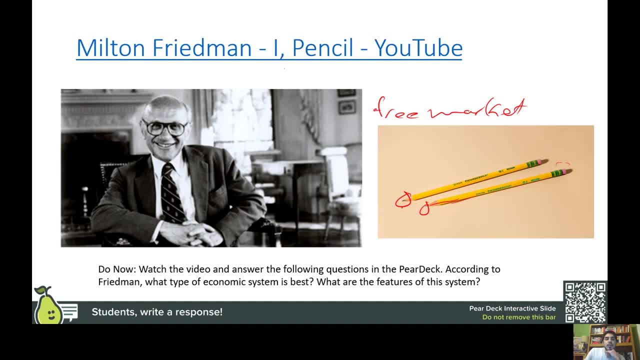 And he really kind of shows how marvelous, how much poetry really is involved in the creation of a simple pencil and then how cheap. it is right, And he attributes a lot of this to the free market. but some of the aspects of a market system that he really does, you know, or features of a market system that he identifies as specialization right, 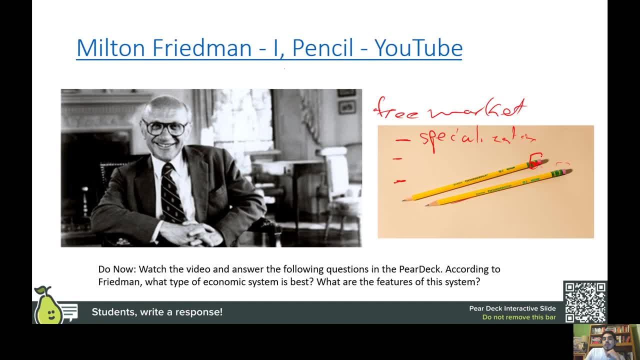 He says that there are going to be people that specialize in producing a certain aspect of this pencil and that increased specialization, He claims it's a feature of the market economy but also leads to greater productivity and, of course, social welfare, because now you're able to buy this pencil at a cheap price. 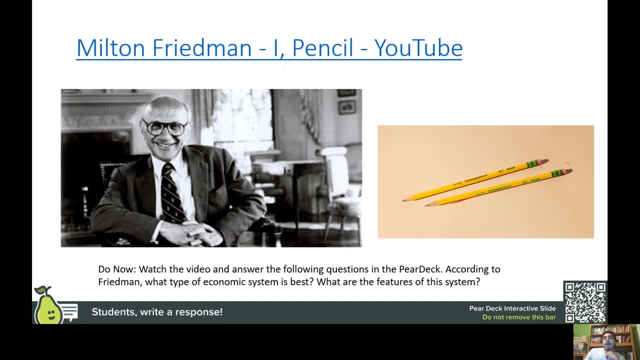 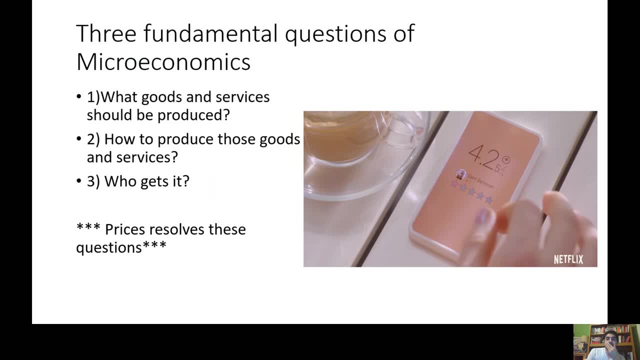 He doesn't really explain the logic very well in the video and how he arrives at that, but the Lehigh piece that we did read on knowledge and society does explain the logic. The fundamental questions of microeconomics are what goods and services should be produced. 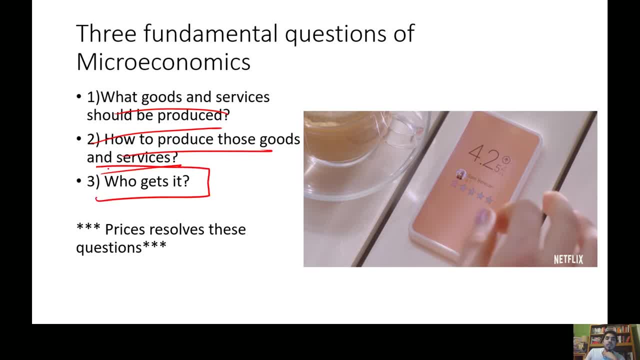 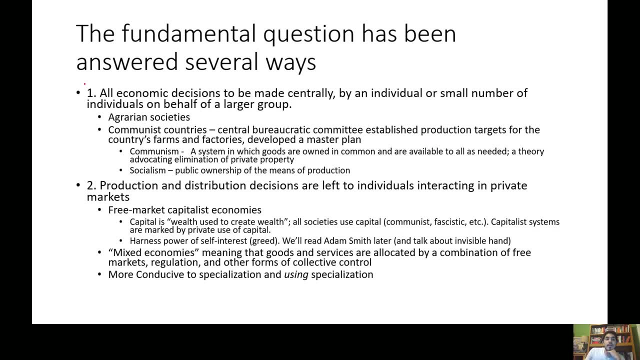 How to produce those goods and services and who gets those goods and services. And so the ways that historically they have been solved- or, I'm sorry, these questions have been addressed- is historically all economic decisions have been, or, in some societies, economic decisions across time have been made centrally by an individual or a small number of individuals on behalf of a larger group. 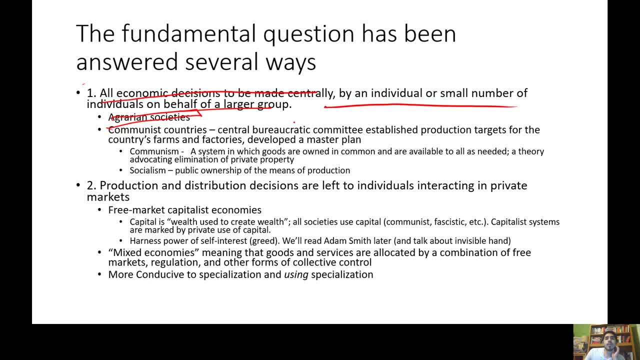 So think agrarian societies. Okay, You know, you might have a very small tribe, that, where there are production and consumption decisions being made centrally. or you might have, like a very small, you know, a family that is literally just producing and consuming whatever it may, or, I'm sorry, consuming whatever it produces. 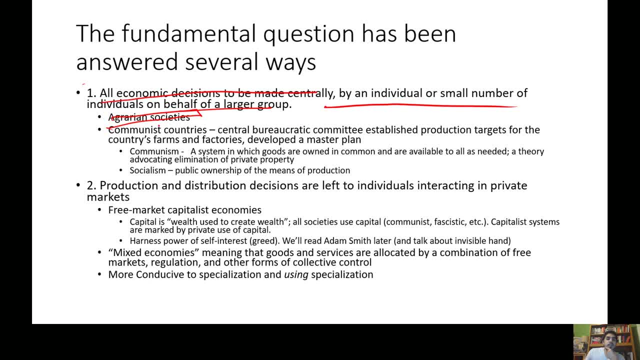 There's no excess, there's no exchange of resources and all that sorts of stuff, And but of course these have fallen out of favor. But in communist societies, in communist countries, there's central bureaucratic committee established that establishes production targets for the country's farms and factories. that develop a master plan. 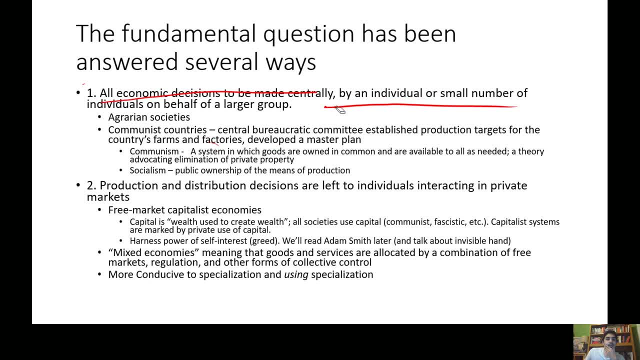 So a lot of us kind of use this language of like China being a communist country, but the truth is China is an authoritarian country. But they do have a very interesting and weird sort of state capitalist model: heavy government intervention in the economy, For sure. 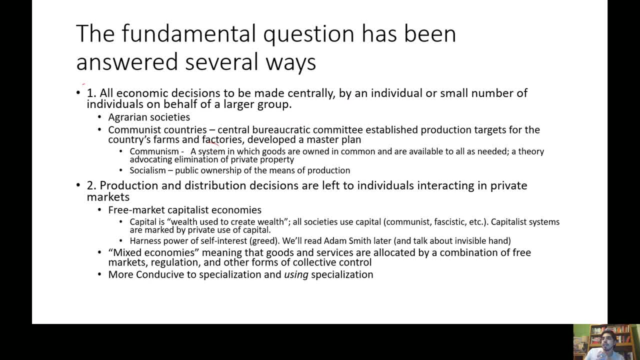 But also sort of using, you know, quasi sort of free markets to achieve efficiency, And we'll see why markets are efficient in a bit. So the definitions of communism and socialism, Cool, And then production and distribution decisions are left to individuals interacting in private markets. 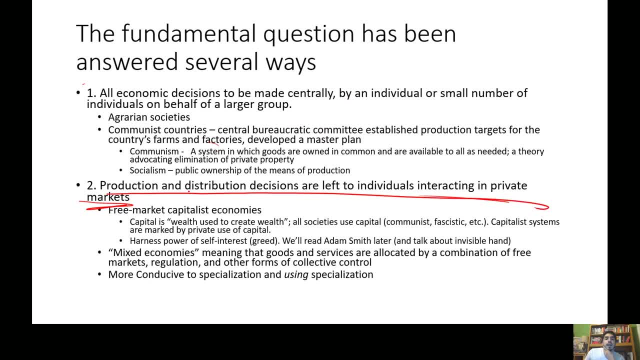 Right. So this- and we'll discuss why- The free market conditions, Free market capitalist economies and mixed economies tend to be very efficient at allocating resources. So we talked about capital as the wealth used to create other wealth. And so in free market, capitalist systems, since the private ownership of the means of production, or the means of production are privately owned, 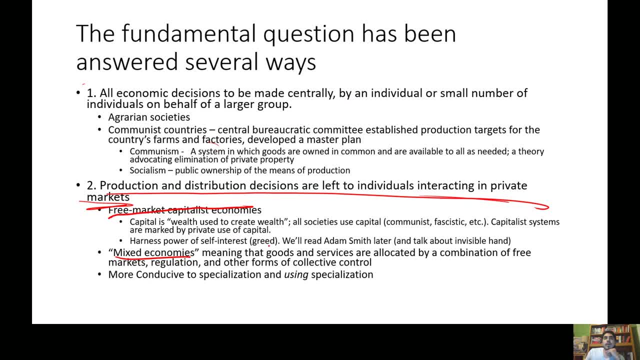 People are assumed are producers and consumers Are sort of left, left to their own devices in this sort of system to produce and consume whatever it is they desire, And as they exchange whatever excess is that they produce with another person, they are able to acquire different goods. 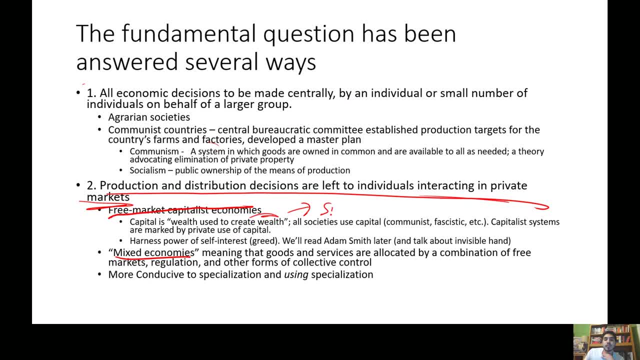 Right. And this system, we are told, is conducive to specialization. You're going to produce, You're going to produce whatever it is- you're good at producing and you're going to sell whatever it is- you're good at producing- and you're going to consume. 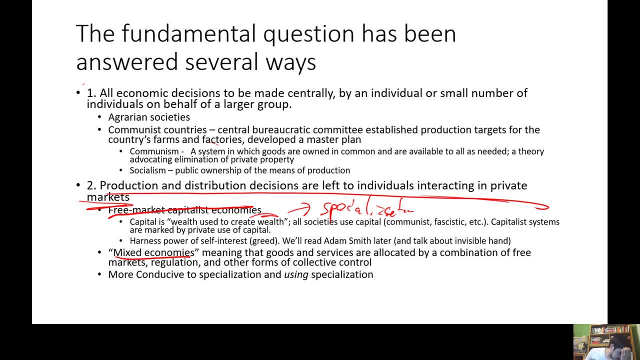 Or you're going to trade with other people and consume whatever it is they're good at producing and all that sorts of stuff. in this sort of system, like the ideal typical, We have a mixed economy. We have And we rely on the market for allocating resources. 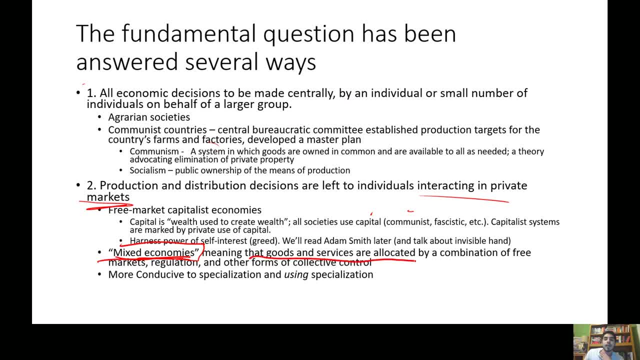 And we'll explain why. that's an efficient way to allocate goods and resources most of the time. But there are these things called market failures, which we're going to talk a lot about at the end of the course. But our economy has a combination of governmental development, free markets with regulation and other forms of collective control. 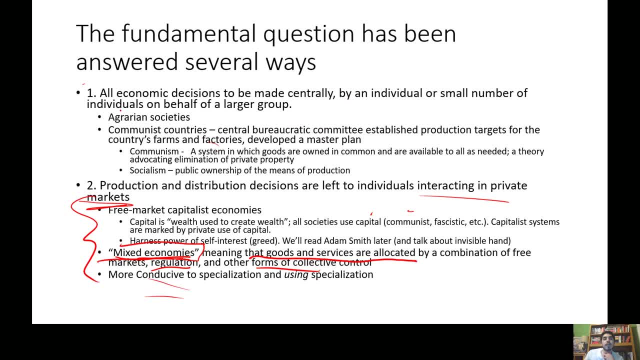 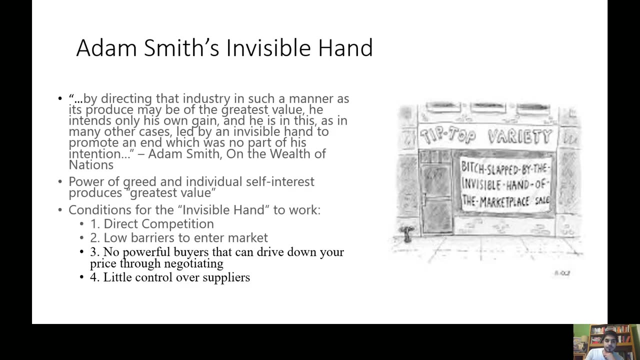 These are much more conducive, these systems, than these centralizing decision making in a small group or committee Right. They're much more conducive to specialization and specialization is very important for increasing the production potential of people and an economy. So we'll talk about Adam Smith's visible hand when we get into unit three and talk about perfectly competitive markets a little bit. 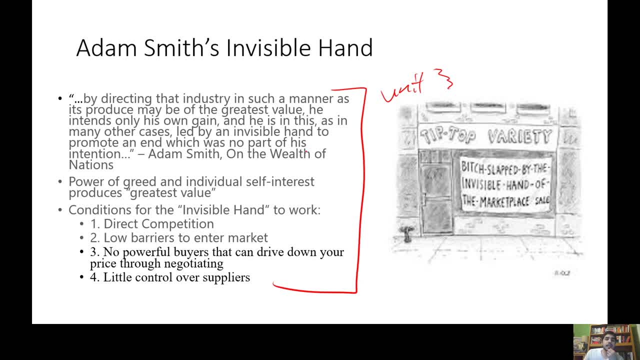 But all I wanted to say is that in a free market system, The theory is that there's an invisible hand that develops, that if people operate and are left to their own devices to produce and consume whatever it is they may do, This system is more conducive to specialization. 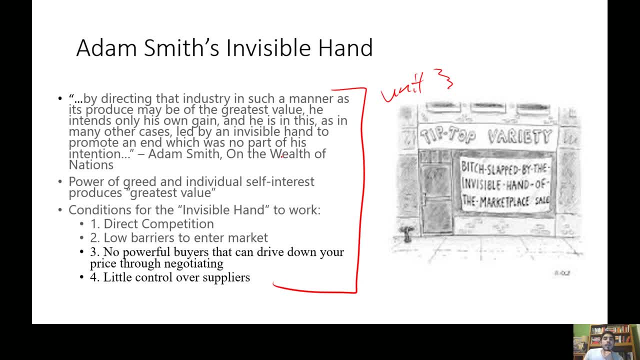 It's going to increase greater productivity and productive potential of people, But it's also- and it's a system that is fundamentally motivated by greed and the interests and self interests of people- But it's also- But it's also going to sort of, you know, produce a a just result, like it's going to produce a socially or welfare maximizing result by itself. 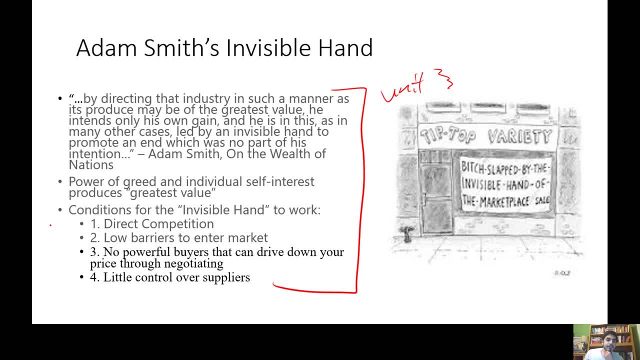 And we'll explain this logic more fully later. But for this to hold, for the invisible hand, as Adam Smith articulates it here to hold, You need direct competition, Low barriers to enter the market, No powerful buyers that can drive your price to negotiating. 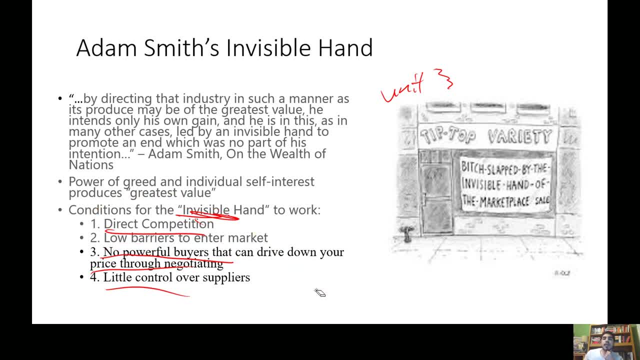 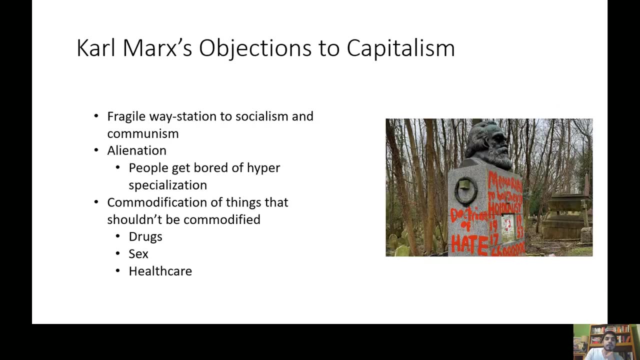 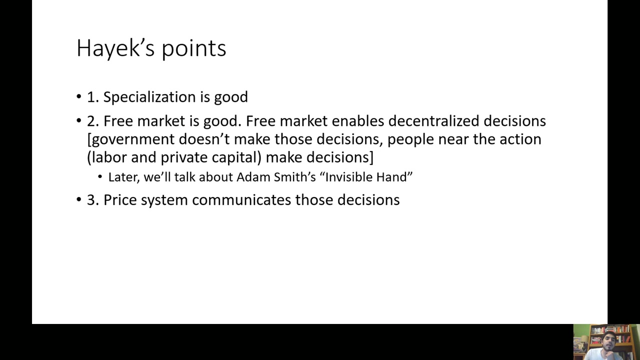 Little control over supplies. We'll talk about this in unit three, And then we'll talk about how this doesn't always hold in unit four, when we talk about imperfectly competitive markets. And so we read Hayek's on knowledge and society, And then I asked you to summarize his main points. 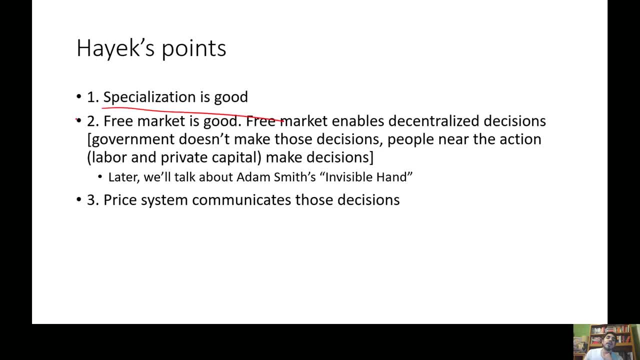 And one of Hayek's main points is: specialization is good. The free market is good. Free market enables decentralized decisions And specifically he says: Hayek says that decision making should be made decentrally if possible in an economy, And the reason why you are, when determining answers, are trying to come up with answers to society's three fundamental economic questions of what to produce, how to produce it and who should get it. 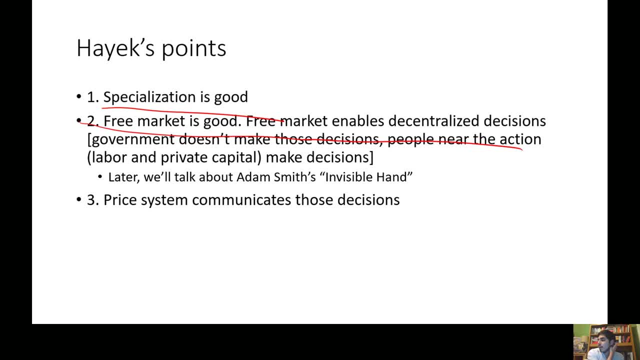 And the reason why he says that decisions should be made Be made decentrally is because he says there's a variety of different things that happen in an economy. right, There's so much information that is that goes on in an economy that is relevant for an efficient allocation of resources. 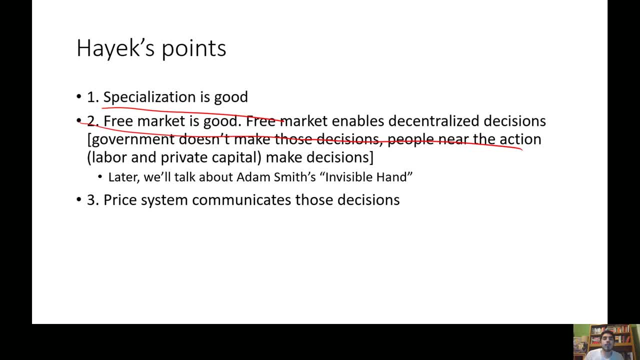 There may be like a sort of you know machine failure in one firm And that should impact- that's going to impact production. There may be a shift in consumer preferences overnight And that's going to impact consumer preference decisions and so forth. 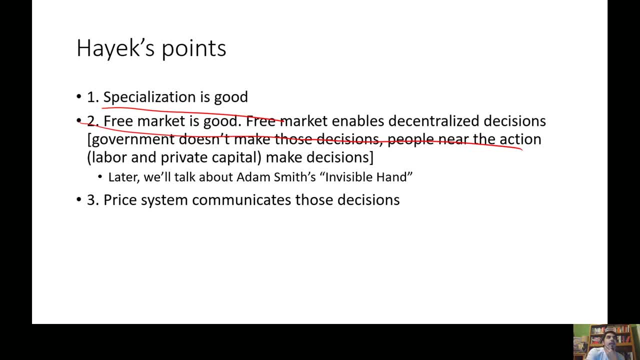 All that sort of stuff he says can't possibly. It would take a lot of time to gather that information, send it to a central committee and ask them to make consumption and production decisions and determine how to allocate scarce resources in an economy. 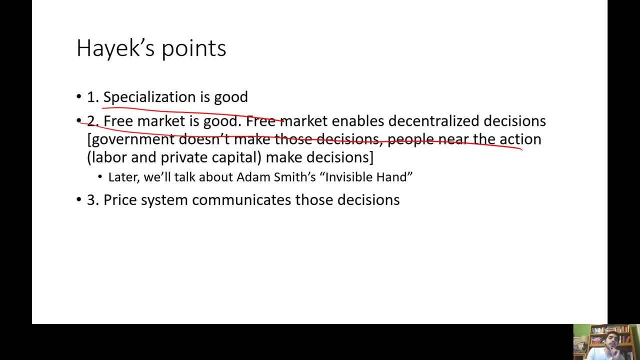 And he says that would be very inefficient. And he's largely right. So he says: And the way that these Decentralized decisions can be made is through a free market system, obviously a capitalist system, where we have private ownership of capital. 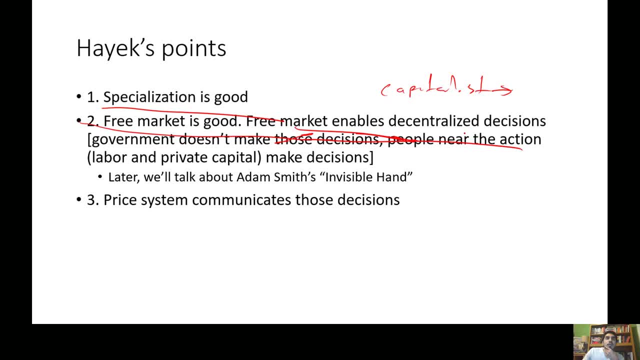 Where we have people that are, you know, have private ownership of capital, that are producing goods and services for profit, Right, You know, kind of relating to Adam's invisible hand and all that good stuff And so he. But the way that these decentralized information is made, 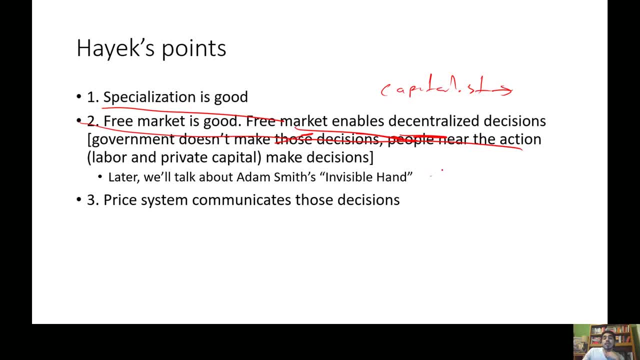 Or the way that information is communicated from these decentralized vantage points is through a mechanism called price And through price systems. Right, We see this all the time. Right, And without getting too much into supply and demand, which we're going to get into in unit two, 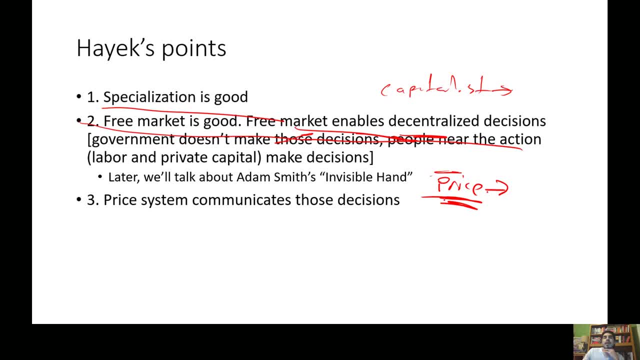 We see that the price system is very good at communicating information Right. If the price of Gasoline goes up, You don't necessarily need to know that the reason why the price of gasoline went up was because there was a war in the Middle East. 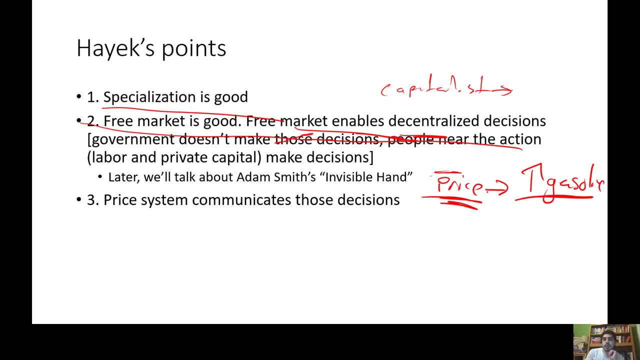 I mean it'd be cool if you did know that, but you don't necessarily need to know that. And there's different producers and consumers that are modifying prices constantly, Right Their own prices and looking at the prices, And we'll talk about you know how, how different productions 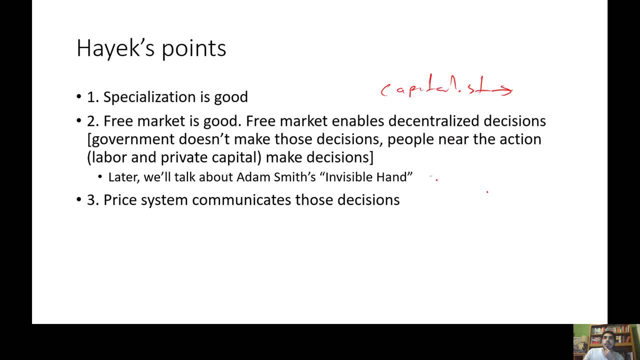 Or how Our producers may be either price takers or price Pricemakers later. But But They're communicating these sorts of information through the price system, Right? And maybe changes in how consumers Or what consumers prefer to buy. 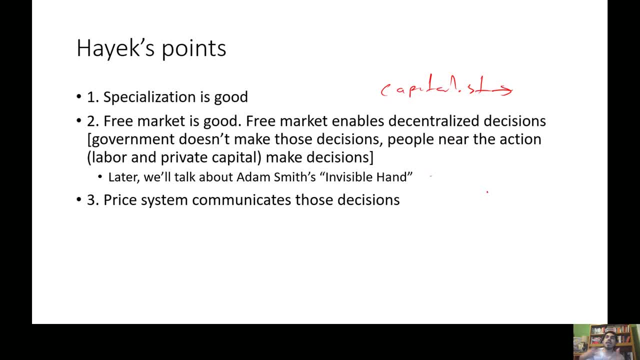 Right And what consumers will ultimately increase consumer utility Are reflected in the price system Right. We know, for example, Bernie Sanders Middens have gone all over the internet And I think You know, You know, You know. 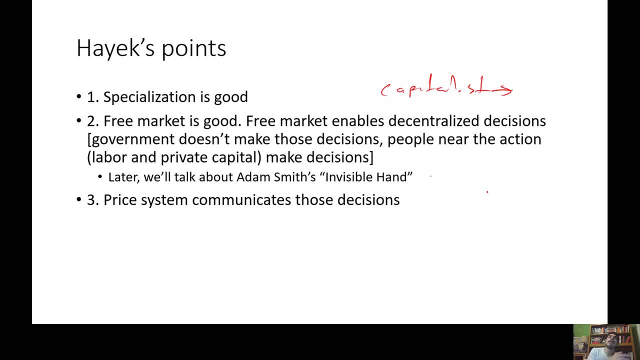 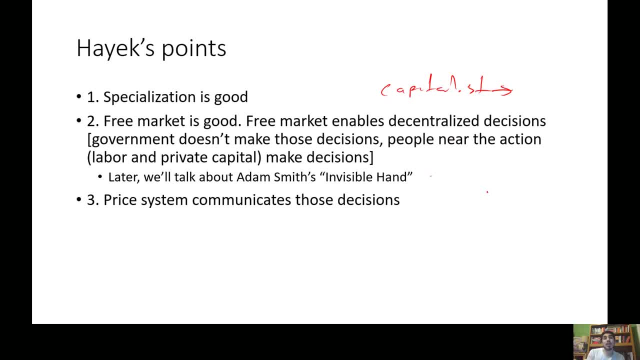 She's going to say good good事 and ad testimonial and concentration over the internet, And I imagine the teacher that made buddy Sanders middens Is now, You know, would be wise to raise her prices on those types of middens. 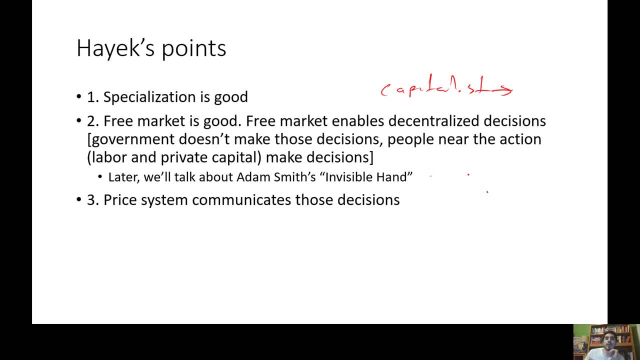 If she were, you know, selling them for profit, So Cool. So all of these stuff. When we talk about all these stuff, We're talking about the efficient nature of the market. The market free markets lead to specialization free markets. 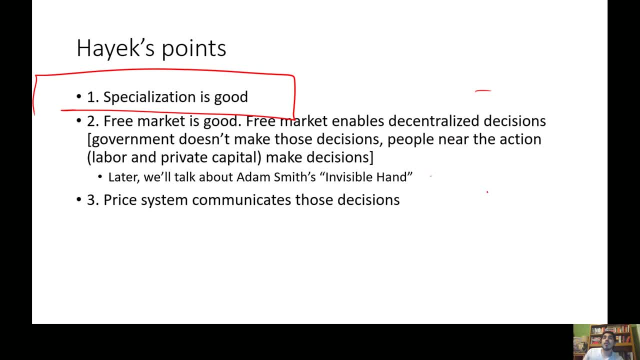 Are characterization By the private ownership of the means of production, They're in centrally planned command economies and so forth. they lead to specialization, they're conducive to specialization and the way that this information, all this information in the market system is communicated about. you know different production possibilities, about different consumption. 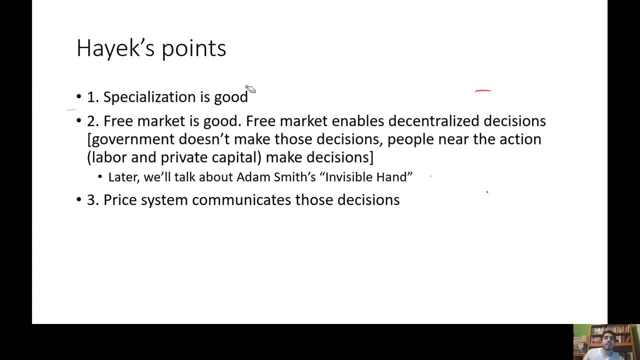 preferences is, through the price system, right, and so free markets, for the most part, are really good at allocating resources, and it seems- and to go into ap government, it seems- like laissez-faire economic ideology is for the win, right. a lot of you might think that this is the logical conclusion. mr diaz, this is it. 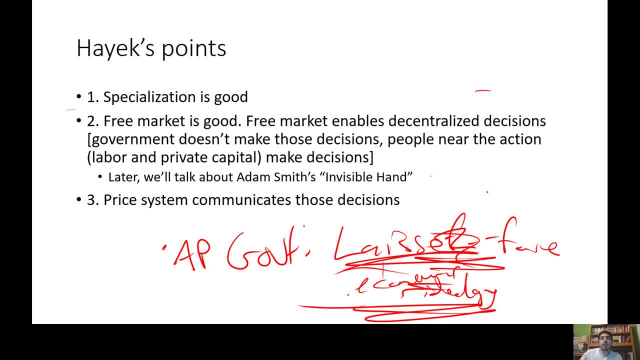 well, you know- and this is me not taking a position on this, but you know, economics is not done right. there's this thing called market failures, and we'll get to this at the end of the course, where the market does in fact fail and the market does in fact produce outcomes that are not optimal for society. 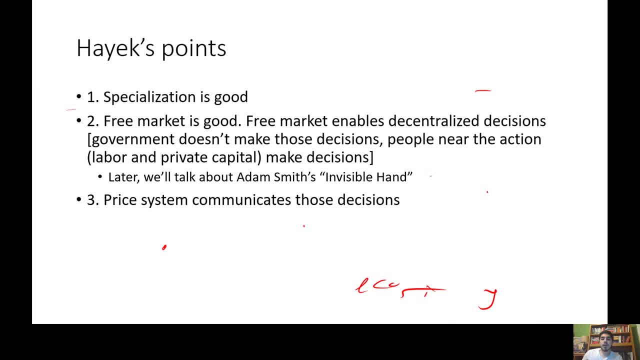 not optimal for, um, you know, social welfare and stuff like that, and we'll talk about that at the end of the course. so maybe, if you have this ideology- remember we talked about this in ap government- you're feeling pretty good, okay, mr diaz, i'm feeling pretty hot and sure, right. 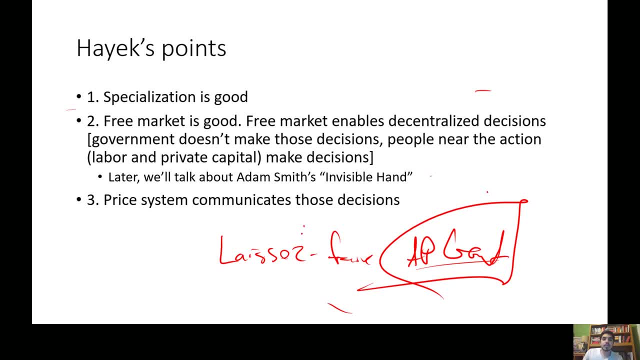 as you should. you know the market is an efficient mechanism for allocating resources most of the time. but just be beware that unit four we're talking about imperfectly competitive markets, and unit five or unit six, i believe, we're talking about what are called market failures. we'll get more into that later. 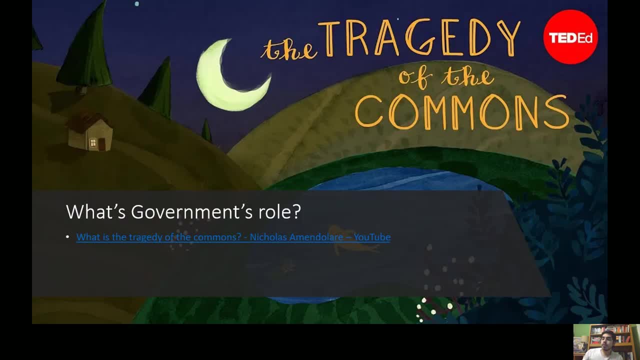 what is the role of government in this? well, the role in government, according to economists, would be in market failures- and we'll talk about market failures in a little bit, but i'm going to talk about failures later- and for the protection of private property rights, i'll include this video about the 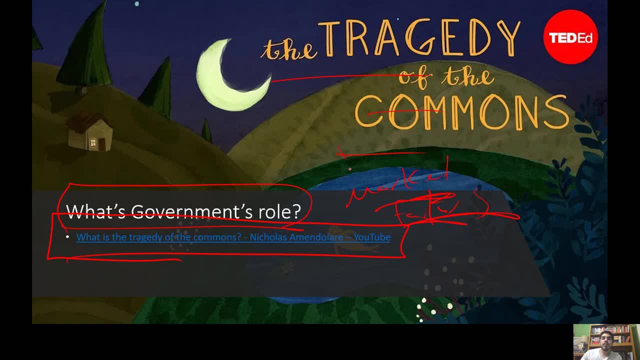 tragedy of the commons. that should make clear to you the importance of private property rights and then, therefore, the importance of protecting private property rights, the importance of maintaining or getting us out of the state of nature. remember ap government content. it's coming back to hide us. remember hobbs and the state of nature where 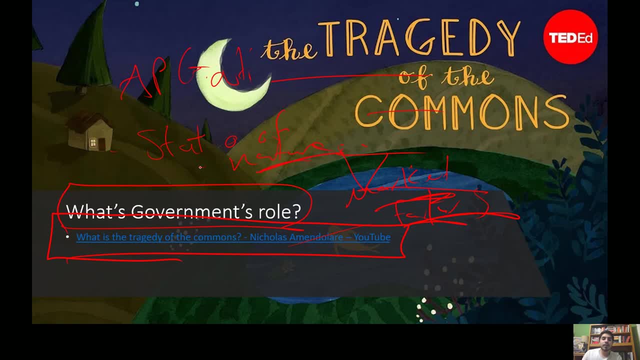 life was nasty, british and short. well, and then we entered into a social contract and you know state and government. well, yeah, government has a role, and we'll find out later. government has a role in rectifying market problems or market values. okay, now we're getting into production possibilities: curves. 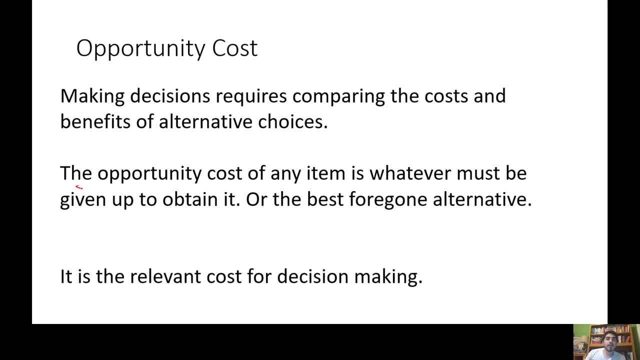 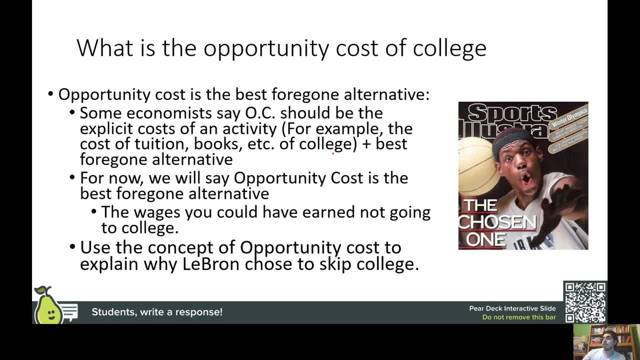 so we talked about this opportunity cost. is the opportunity cost of any items whatever must be given up to obtain it or the best foregone alternative. that's the opportunity cost. we talked about the opportunity cost lebron james would face going to deciding to go to college instead of going to um. 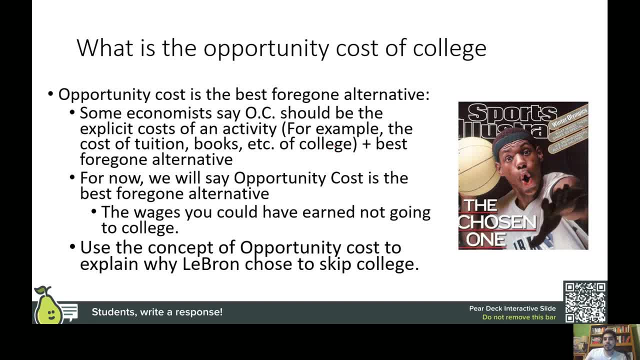 i'm sorry that was gross, but i am so thirsty because i've been talking so much. but the opportunity cost lebron makes to face, he might face explicit costs of going to college, explicit costs or accounting costs of college itself, but economists don't just care about this, right, he might face, you know, cost of books. 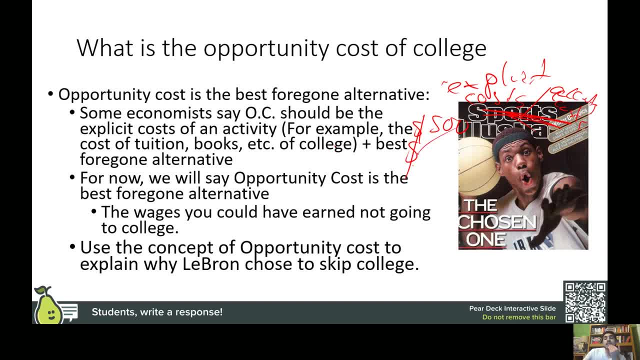 500 books, cost of tuition and fees. economists don't just care about this, they care about the opportunity costs. what did lebron james give up to? go to four years of college at, let's say, duke university? if he decided to go to college, he didn't, he went straight to the pros. well, he would have. 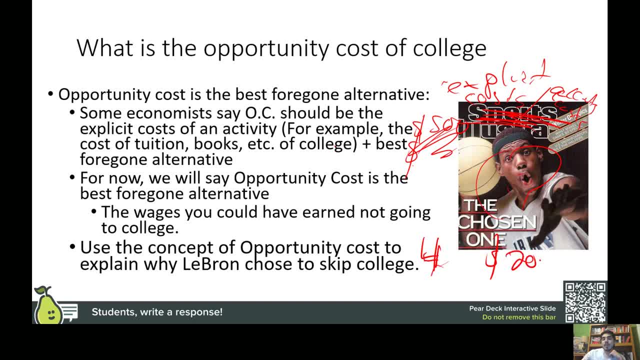 given up you know millions of dollars because let's say he would have been making 20 million, um, i don't know how much he made in 2003. 20 million dollars per year. you know a duke degree which he probably could have gone to duke um basketball is worth what? about 2 million, i think. 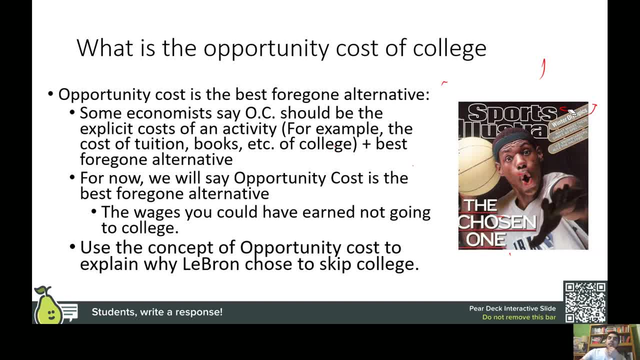 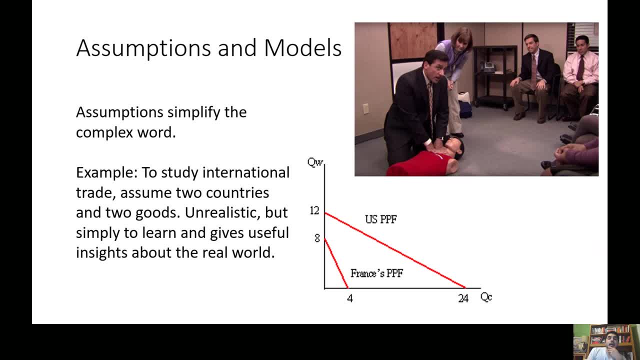 over a lifetime right, not worth it. but the opportunity cost is prohibitively high and so he was rational in deciding not to go to college. and we'll talk about rationality and optimal decision making later. um so the production possibilities frontier. we said that it's a model and um, it's an economic model. it's specifically a pedagogical model mostly. 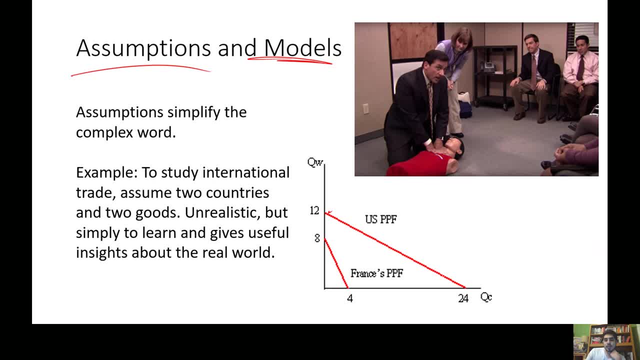 um, nobody's going to be like, bro, i need you to draw production possibilities frontier um, or you're not gonna get the job. no, uh, production possibility for frontier is a very, very, it's very, it's a very. it's a simplification of um the production possibilities. 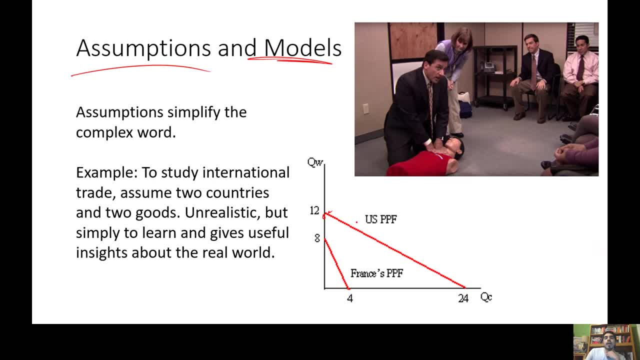 um of a person, business or a country, and when we're going to use it in this class, we're going to use it to illustrate the gains of trade. so it's a pedagogical model in the. in the sense, pedagogy means um, um, an approach to sort of teaching and learning um, but it's a pedagogical model in the. 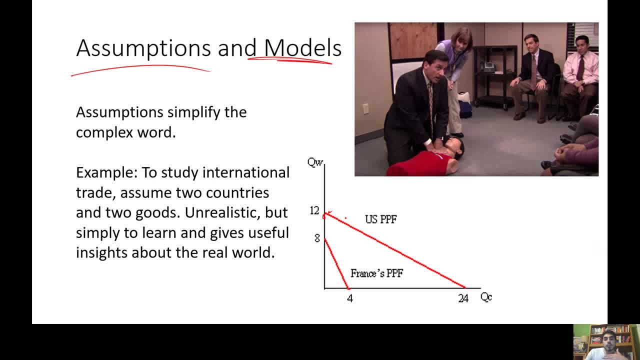 sense that it's meant to. it meant to teach you a concept about trade, teach you a concept about specialization, teach you a concept about the benefits of specialization, specifically. so we'll talk about this in a bit. so, to study international trade, assume two countries and two goods. 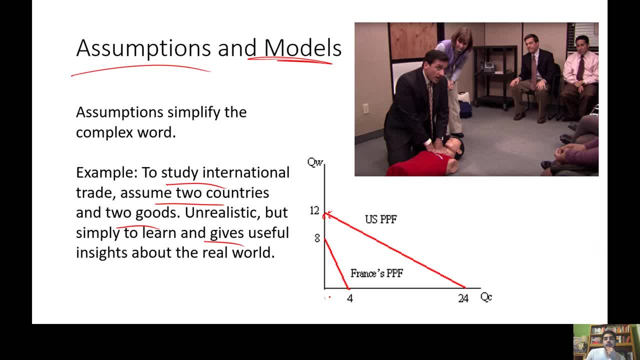 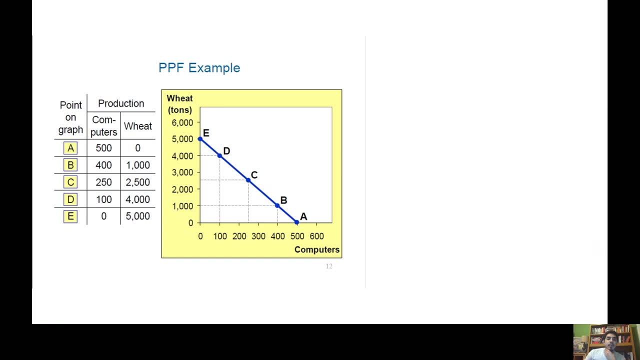 all that cool stuff. so we'll talk about this using um pps. so this is an example of a ppf. uh, wheat in tons. we said that you might be forced to graph a ppf and we said that oftentimes you'll have problems that are going to. 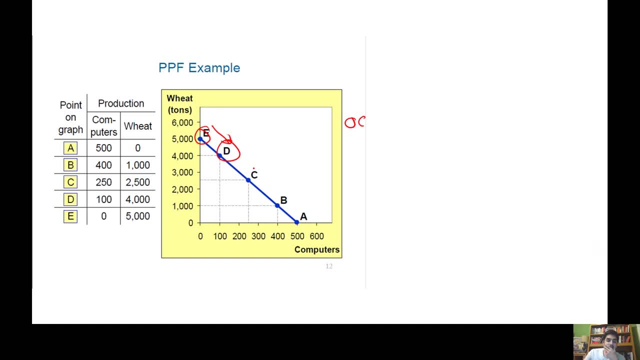 be a little bit more complicated than what we're going to talk about today. so we're going to talk about this again, explaining to you what the opportunity cost looks like. what are the cost of moving from D to E? it would be, of course, from D to E, is what is that? 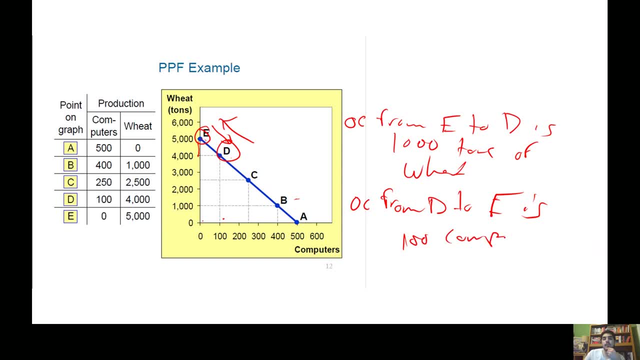 Is 100 computers right, Because we go from making 100 computers to zero computers, Boom, Okay, And so linear. this is a linear PPF, PPF production possibility frontier And this is significant because linear production possibilities frontier have this special 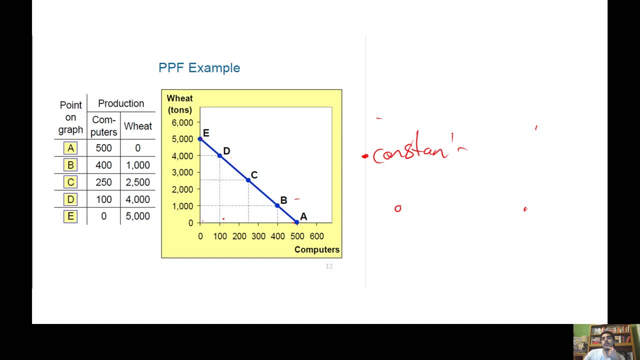 idea of a constant opportunity cost. And what specifically I mean by a constant opportunity cost is similar magnitude movements along this line. So what I mean specifically, if you increase units from increase production, from zero computers to 100 computers, your opportunity cost is 1,000 tons of wheat. 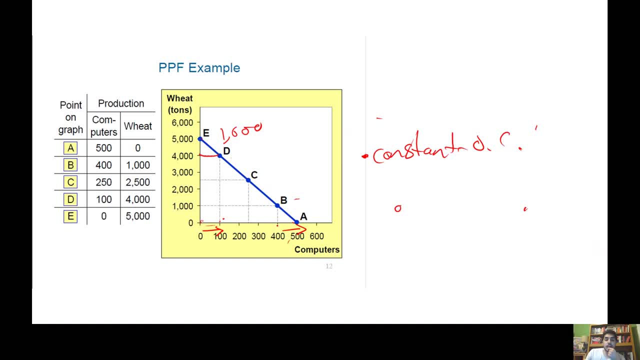 This, because of the constant opportunity cost, means that if you increase production by the same magnitude- 400 computers to 500 computers- you should expect the same opportunity cost, which is what you have, which is 1,000 tons of wheat, Not all PPFs. this is. 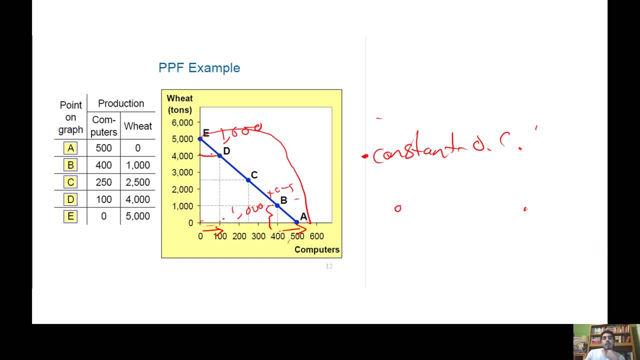 this is a very unrealistic PPF. A more realistic PPF would be one that's bowed outwards and one that's bowed inwards, And we'll talk about why they might be bowed outwards, But we won't. we'll talk about why they might be bowed inwards, yet So cool. 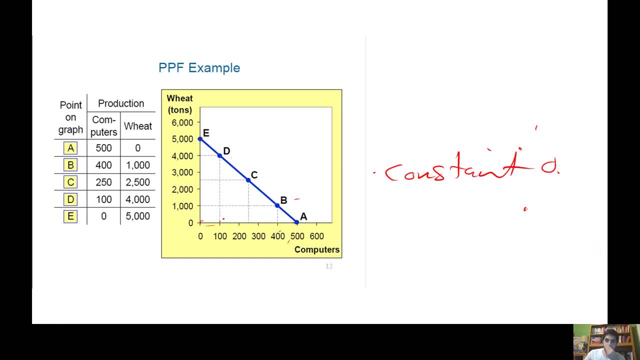 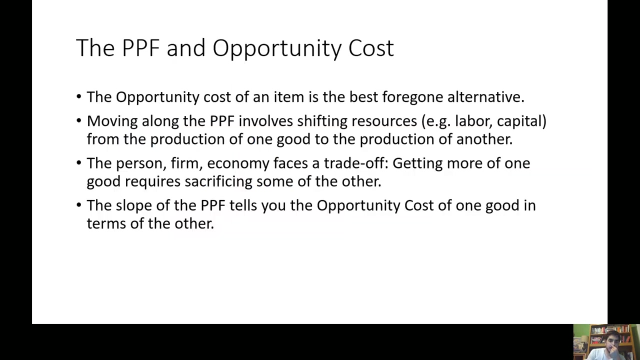 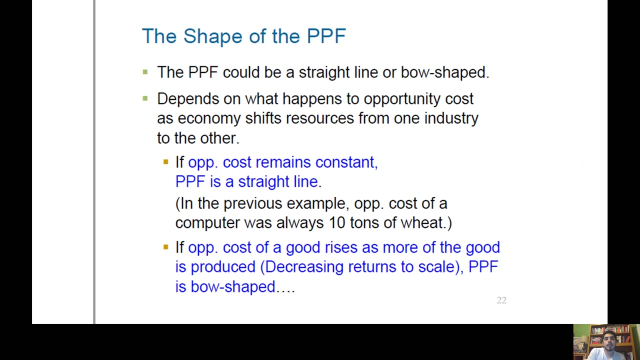 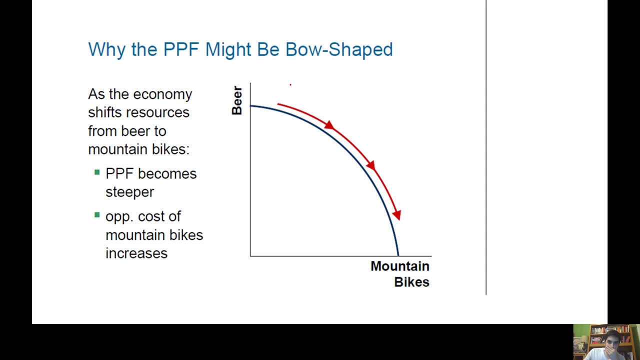 Also. for now we'll talk about returns to scale when we get into the unit on imperfect competition, But unit three. but just remember that a constant opportunity cost reflects that there are constant returns to scale, And so a this is the shape of a bowed out PPF And this in this PPF of, let's say, economy, A. 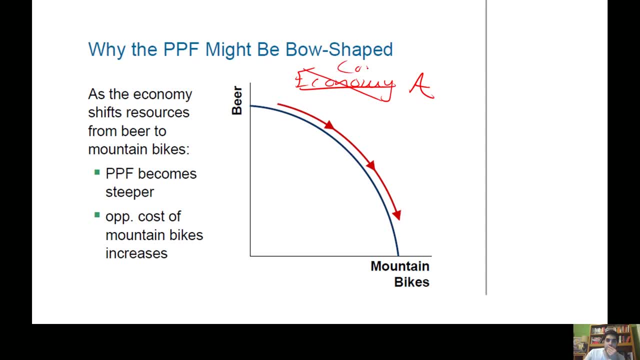 or a country A maybe, And this production possibility, frontier of country A, and remember, a PPF can be of a country, a person, a business, doesn't matter. We can see that there are increasing opportunity costs, meaning that a similar magnitude shift from here, as we can see, would not significantly impact. 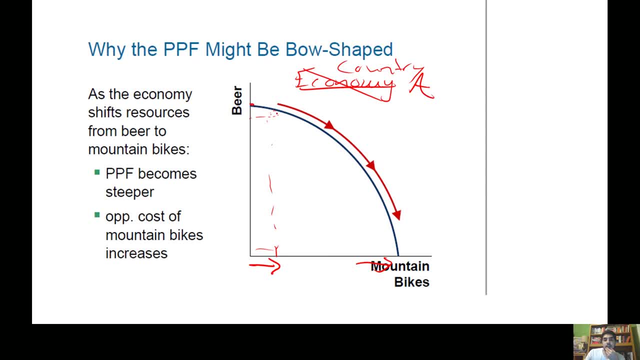 opportunity costs, right. So we start here and then we go to the end, to the end of the project, to the end of the transition process, and then we go to this unit right here and we don't expect a major drop off in terms of. 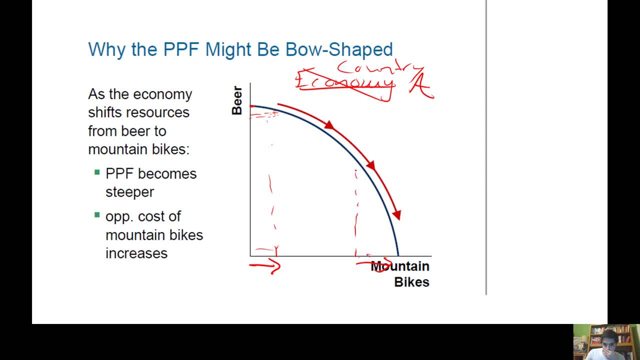 opportunity costs. however, the same magnitude shift here. from here to here, we can see a major drop off in terms of opportunity costs and the magnitude of opportunity costs. the question is why? what does this vote out? ppf, you know, signify well. so, at point a, the opportunity cost of mountain bikes. 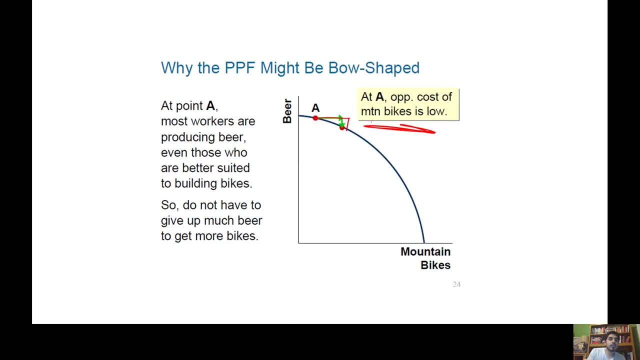 is low, as we can see, so do not have. but at point b, most workers are producing bikes. oh, so, at point a, workers are producing beer, even those who are better suited to building bikes, right. and so you know, giving up a lot of workers isn't going to significantly alter your production. 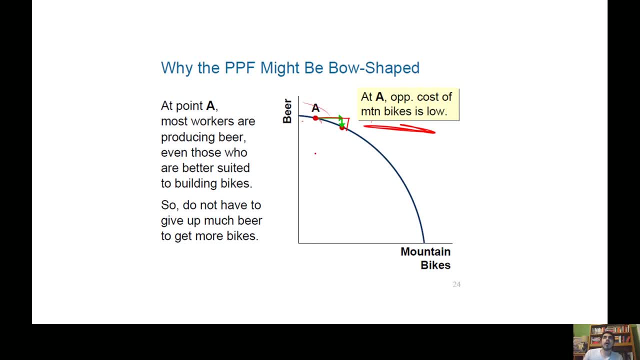 also i will say that these pps assume they're, uh, assume- one factor of production. in these pps there are different types of models that assume multi, multiple factors of production. but i mean you're allocating resources, you know, towards mountain bikes, you're allocating units of labor. 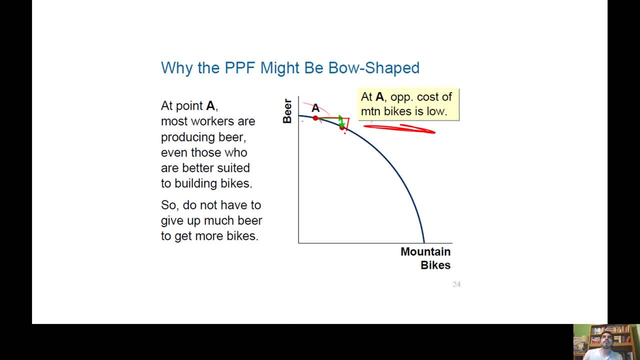 and all that sorts of stuff. but you can also think of it in terms of of: um, you know a lot of chefs in the kitchen. uh, maybe you really don't need that extra labor. um, you know, producing beer, like there's maybe a lot of people that are just like so crowded in this, this, like beer. 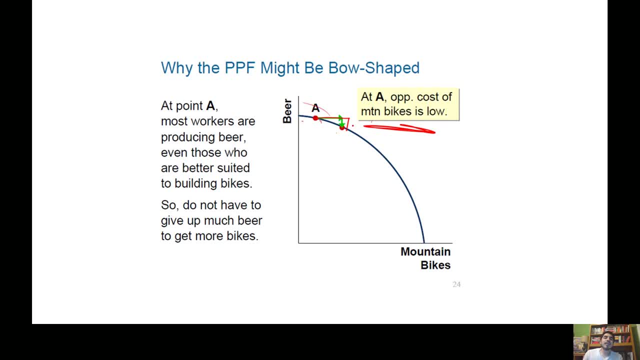 production facility, that letting a couple go isn't going to significantly affect, uh, your output or production, and maybe you can let, like, the losers go right, the ones that really suck at making beer. uh, that may be really well suited to making mountain bikes, right, so that's okay. but as 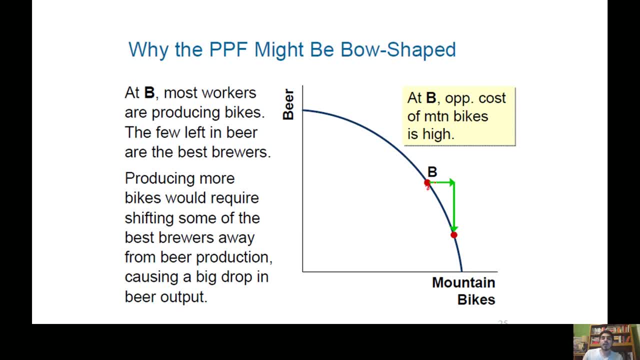 you get closer and closer, right. you're really at this point you're giving up maybe the best and most skilled beer makers. so hopefully that makes sense to get you into that, into the realm of beer making. right, but at this point you're giving up maybe the best and most skilled beer makers. so if you get to 20 beer makers, 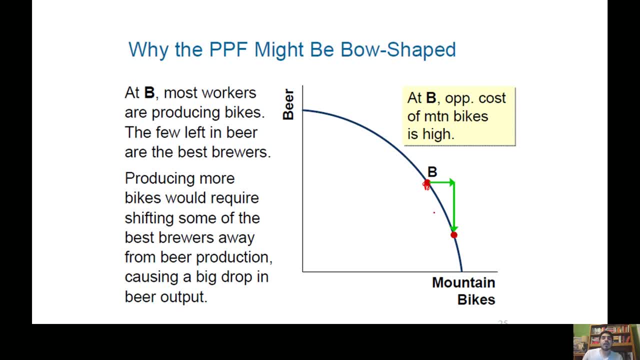 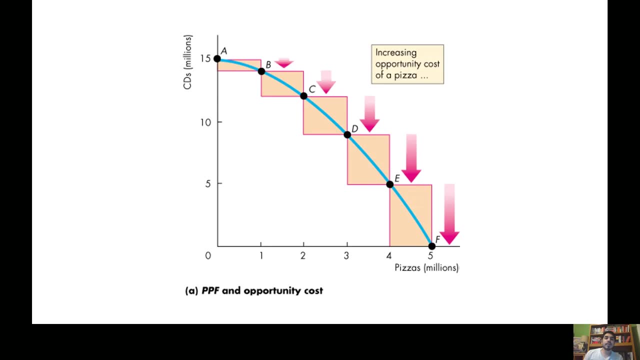 makers and and and putting them towards the production of mountain bikes. so you should expect your opportunity costs to get increasingly, increasingly higher in this boat out shape. so this is an increasing opportunity cost of a pizza. you can see it here. similar magnitude shifts and you see that there's an increasing opportunity cost. 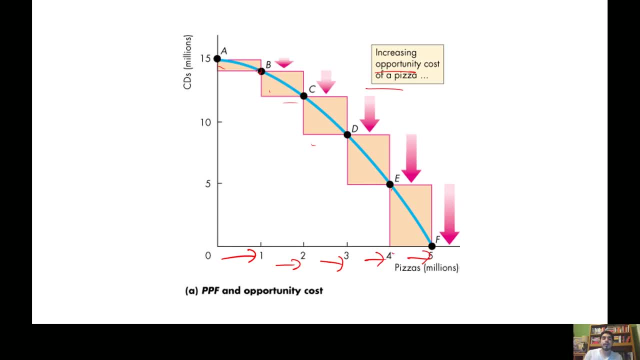 despite similar magnitude shifts, increasing opportunity costs. before i continue, i want to say that this represents increasing opportunity costs and decreasing returns to scale. you can also manage, or as a- okay, there's also another sort of graph- looks like this and we'll explain when you can expect increasing returns to scale. 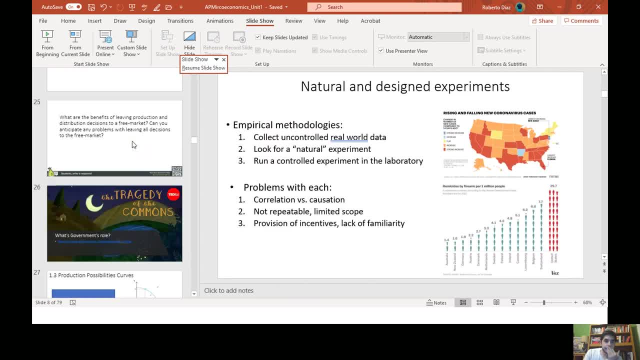 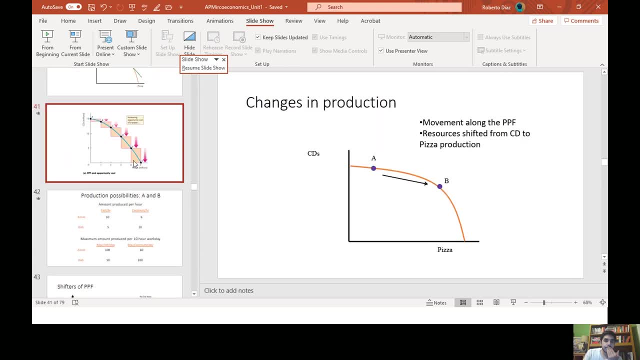 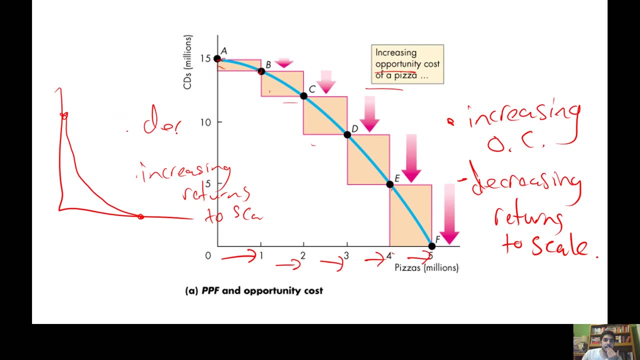 damn it. oh, that wasn't to say that one decrease in oc and decreasing oc. this happens in a lot of natural monopolies and we'll talk about this in unit three. but just know it, just memorize it. so if you're graphing a ppf and they look like that, memorize. 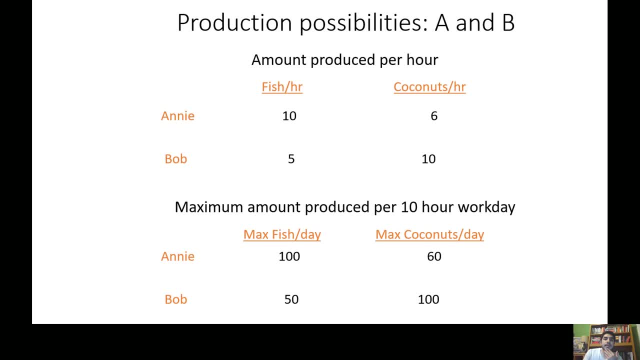 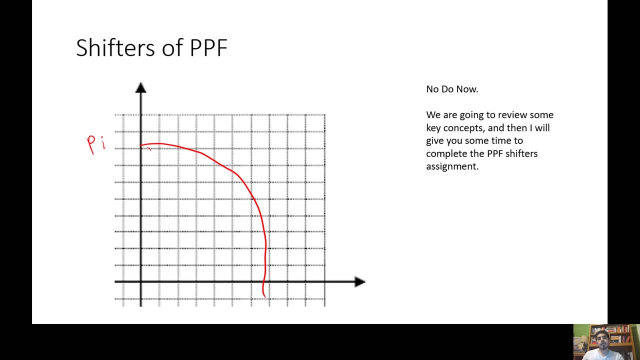 google, production companies, amd, shifters of ppf. oh yes, so we also want to talk about shifters of ppf. let's see, i'm not gonna go into that because we're gonna talk about the ppf. that's just something right out of pizza, pizza and bikes: shifters of ppf. so at these points on the production possibilities frontier. 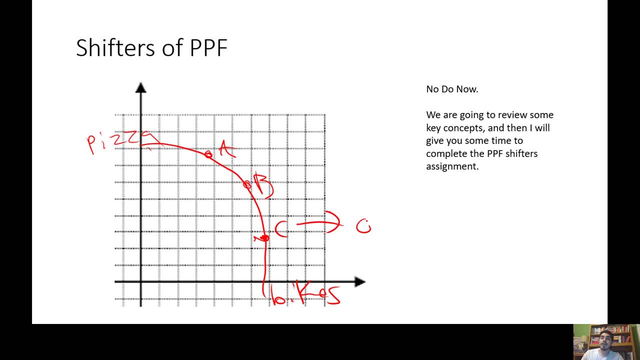 they're at the frontier right, and so we should expect that these are obtainable because they are at the frontier. but and efficient abc right here, that is definitely obtainable right. you can obtain this combination of pizza making, let's say, and bike production, but you are wasting a lot of. 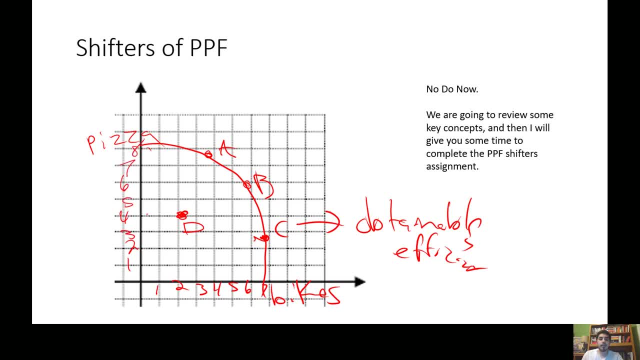 resources. it's obtainable, but not efficient. right, four and two, okay, that's use you suck. you suck at using things efficiently: it's obtainable, but not efficient. and then, over here at point e, that is not currently obtainable, but efficient, cool, cool, cool, cool. and then, when we think about shifters of production, possibilities, frontier. 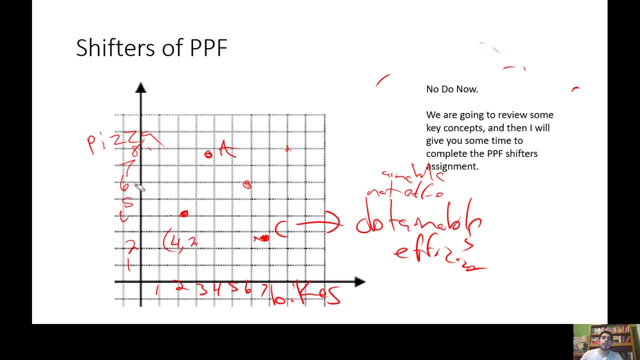 you always want to think of in terms of- let's make this more realistic, you know, maybe effects on the factors of production, technological impacts, financial services, and then let's see on this end- i don't know- let's see fully autonomous weapons. so right and left hand sideニ. 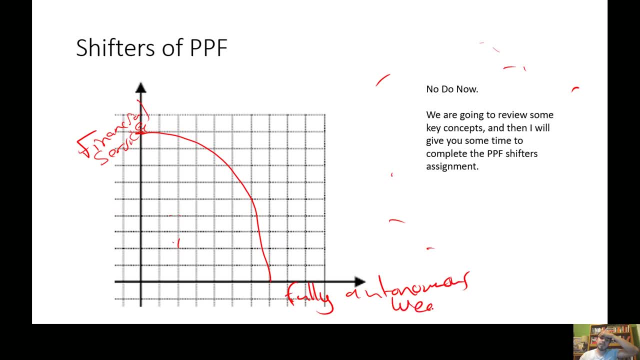 ニ, a, a, c, c, n, s, n, robots- we'll talk about this. we might talk about artificial intelligence later, but so we have financial services and fully autonomous weapons. let's say this is a PPF for a US economy, and so to think about shifters in the production. 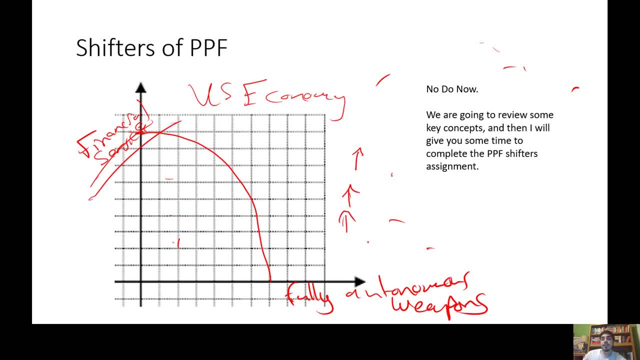 possibilities frontier. we really want to think about factors of production and stuff that might impact factors of production. so, for example, this is remind me to also talk about something else later. all right, no one's there, but you want to think about factors of production and stuff that might impact factors of production. so, for example, 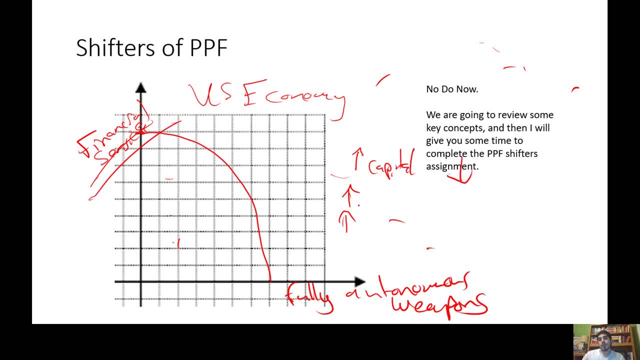 you want to think about shifts in terms of capital, labor. maybe something happens to the labor so they become more productive or less productive. something happens to maybe the entrepreneurial know-how which might relate to labor, or maybe capital, labor and natural resources. so, specifically with capital, you can imagine a world in which, let's say, more artificial intelligence. 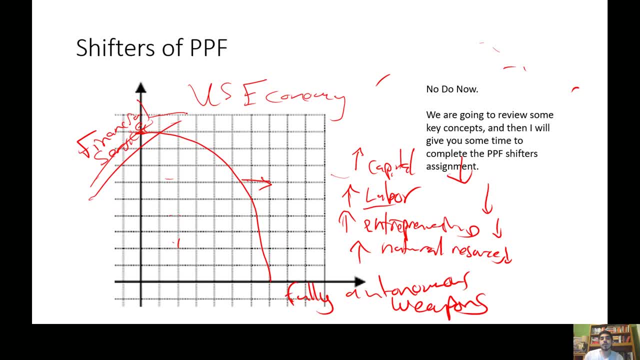 the United States makes significant investments in artificial intelligence. there's breakthroughs in terms of artificial intelligence. this dramatically improves financial services and fully autonomous weapon systems, and so you can imagine a rightward shift from the production possibilities. frontier, right a capital has fundamentally changed. right capital has become. 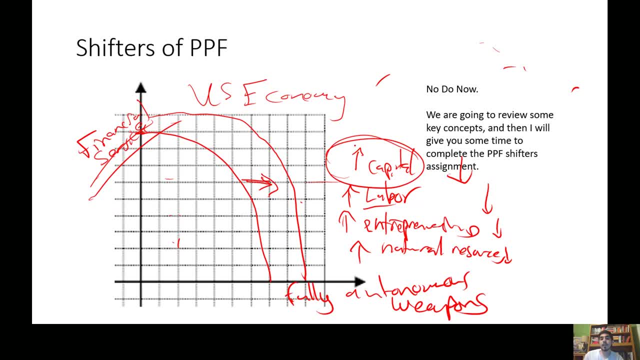 much more. I wouldn't say the supply of capital necessarily increased, but like the technological or the productivity of capital increased. that's what I should say. so think of in terms of the productivity of these services being affected either positively or negatively for labor. one thing that might cause a rightward shift in a production possibilities frontier is maybe 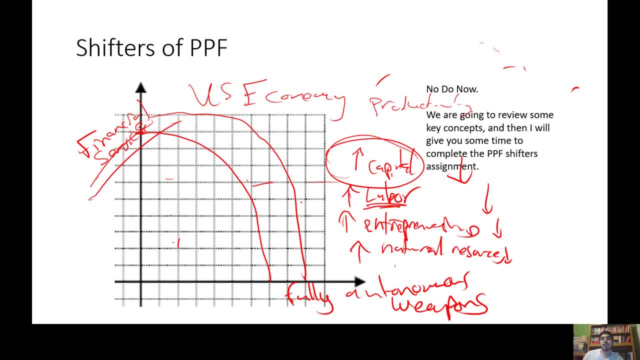 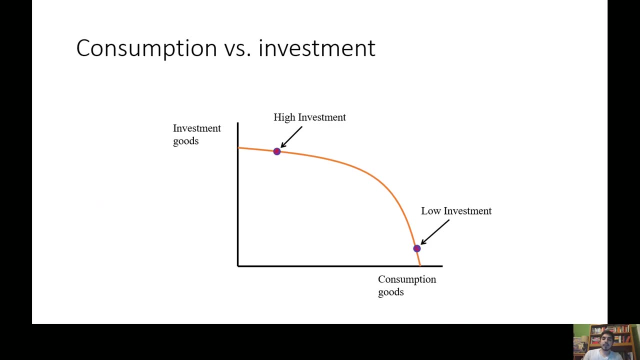 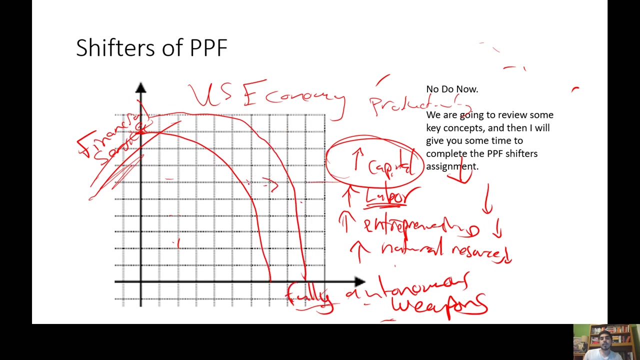 suddenly compulsory education? education is known to increase the ppfs. maybe compulsory stem education, right, this would seem to to dramatically affect. you know, stem is kind of needed for financial services a bit less than fully autonomous weapons, but certainly it would affect fully autonomous weapons. maybe compulsory stem education? maybe everybody is. 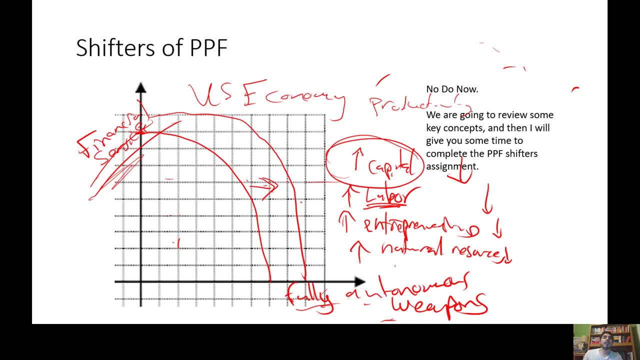 forced to take pre-calculus and engineering in the country and this could dramatically affect the ppf entrepreneurial know-how. that's something that I can imagine, if this is maybe not a ppf, or maybe or maybe. I can't really think of a good scenario, but let's say there's. 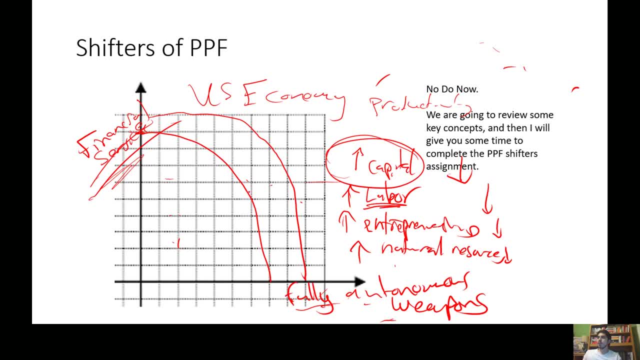 new, I don't know, an organization model, new governmental guidelines, less regulation stuff. oh, I don't know. I don't know what would be a good one, maybe better new resources, maybe an increase, and I don't know what would be a good natural resource like rare earth minerals that might, you know, increase the ppfs. 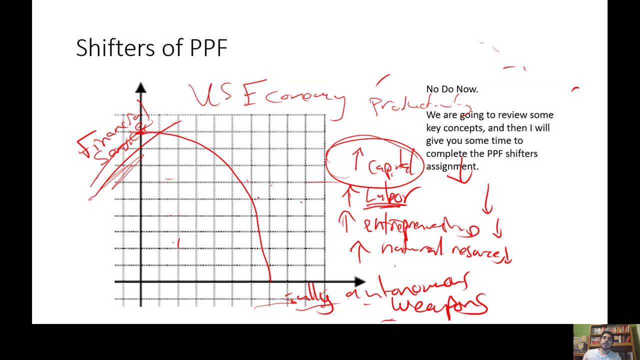 a little bit more towards fully autonomous weapons systems. all that sorts of stuff might lead to a rightward shift. a leftward shift could involve, you know, you know, a breakdown in capital. maybe the united states bans the use of artificial intelligence or, in certain contexts, right and so that you know, decreases the productivity of capital, right, or the productive. 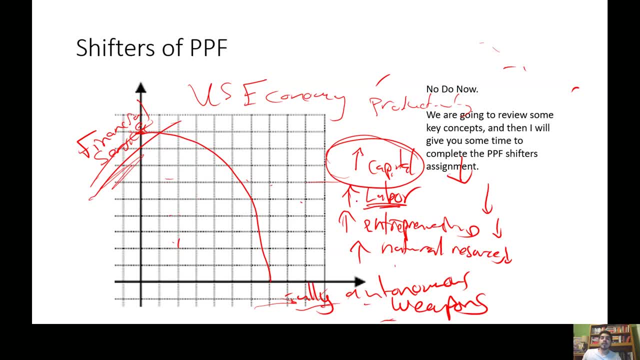 ability of capital. maybe the labor force is going to be able to reduce the productivity of capital. maybe the labor force is going to be able to reduce the productivity of capital. maybe the labor force is. a lot of talk about how distance learning has is probably going to have deleterious effects. 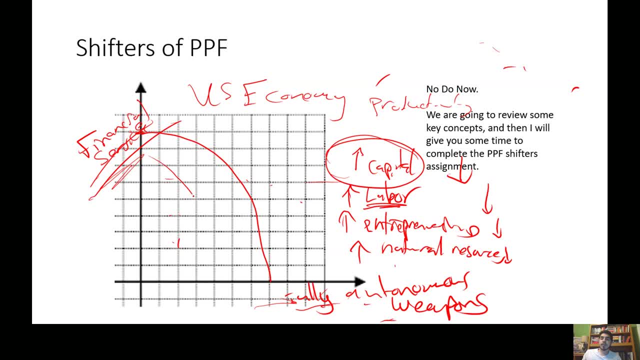 on the productivity of the united states workforce. so we can imagine that you know, kids that are not doing their ap microeconomics homework or not tuning in for the ap microeconomics class are not going to be as well prepared as other kids, and maybe we say that a lot. 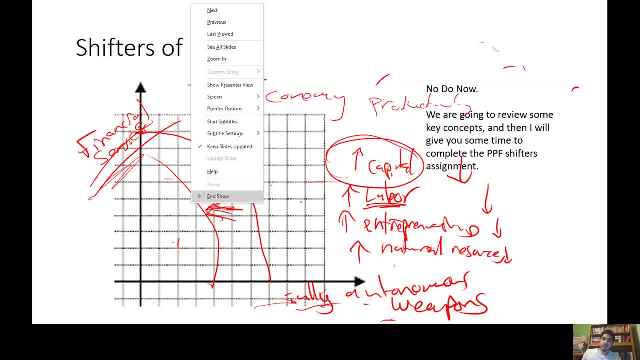 this is happening to a lot of kids and this would be a leftward shift of the curve, right, all that sorts of stuff. okay, so think about when you're thinking about shifters of the ppf, think about in terms of, you know, enhancing or decreasing the productivity. 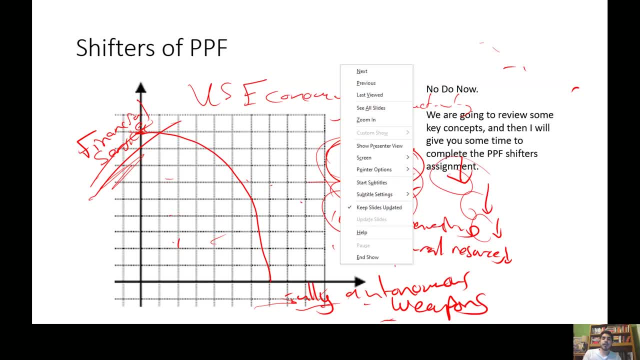 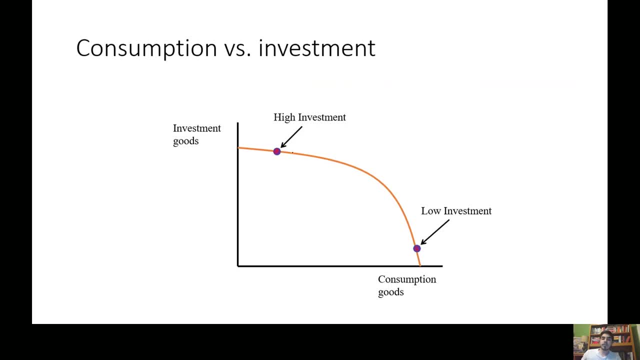 of one of the factors of production and that should have an impact. so we can also use the ppf to visualize the cost of you know consuming a lot of what our students are doing right. so we can also use the ppf to visualize the cost of you know consuming a lot. 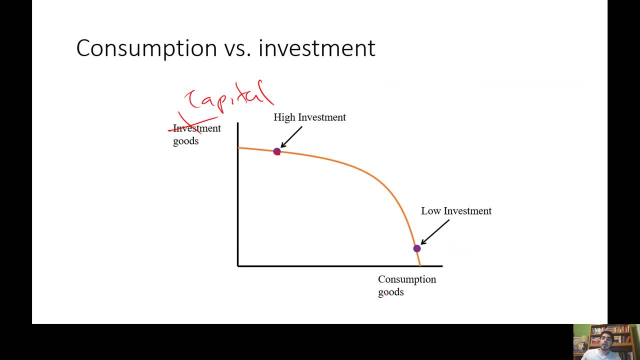 capital goods today and the or consumption goods and investment goods today over capital goods- right to visualize the sort of trade-off in doing that. and so specifically we said capital goods, we talked about capital as wealth used to create other wealth. we can also talk, we can say that these are also investment goods. it's wealth used to create other wealth. so we 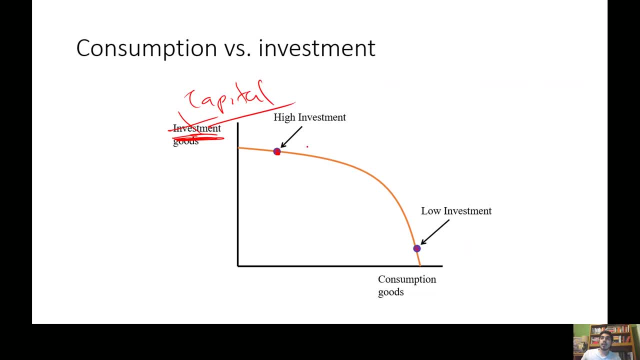 can imagine, if we're producing- i should say not consuming- producing a lot of capital goods, if we're doing other types of investment, right, we're producing a lot of industry goods. um, i don't know if we're going to include the city of california but say, for example, uh, we're producing. 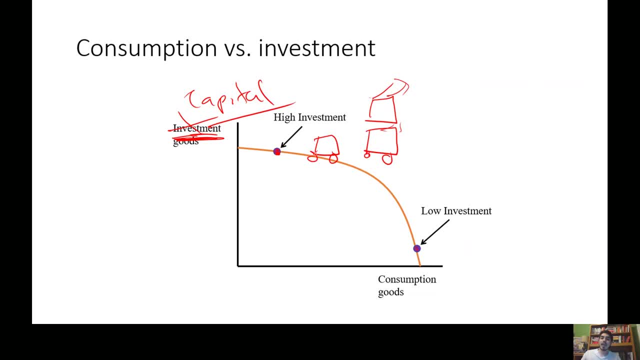 um, some sort of stuff like tractors and trailers and artificially intelligent- um i don't know- services or whatever right. we're producing capital wealth that's going to be used to create other wealth. this is going to lead to a more positive economic growth for the us economy. assuming this is a ppf of the us economy, or this could also be a ppf of a business or firm, but if that business is investing in capital equipment today, then that's going to lead to a lot of investment in capital equipment today. so here's. 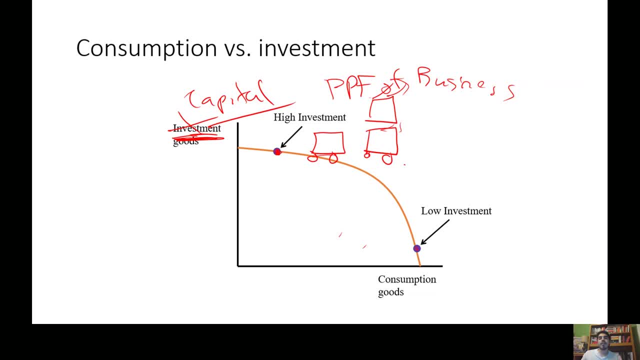 higher growth tomorrow. right, so we can kind of see the temporal trade-off. in contrast, if that business is, you know, producing a lot of consumption goods, not really producing a lot of capital goods, or that that country is producing a lot of consumption goods and in turn consuming, 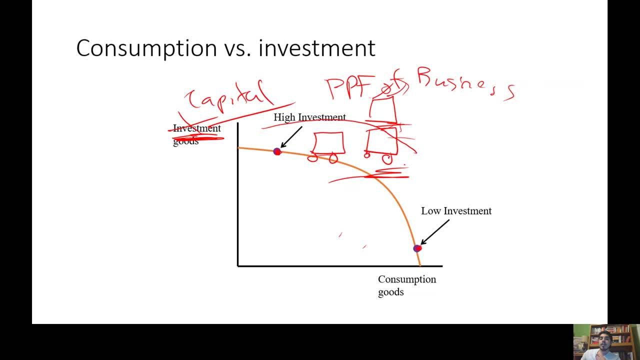 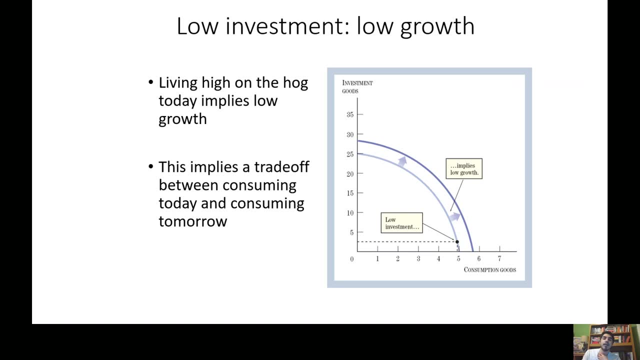 a lot of consumption goods. possibly, then, that that might not lead to a lot of economic growth tomorrow. right, and the way what this implies is: living on the height lot high on the hog today implies low growth. so we can see, right here we're consuming a lot more consumption goods, and here's relatively 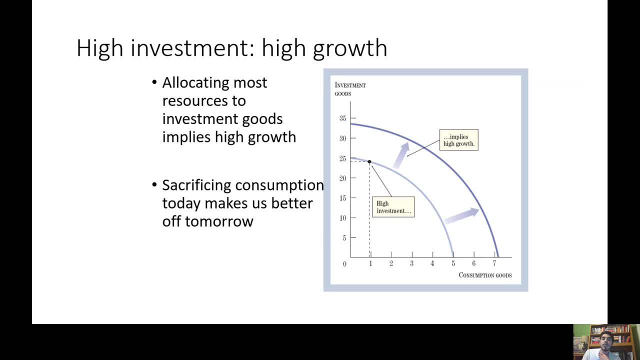 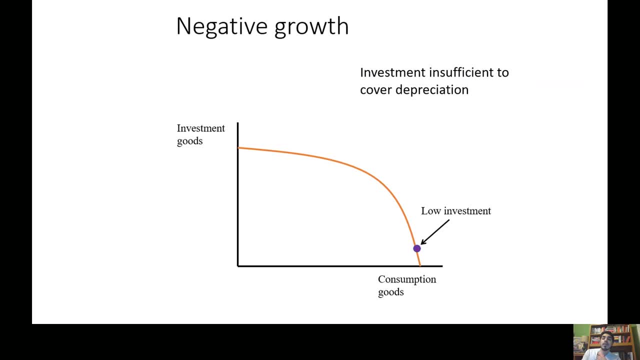 low growth compared to um a more expansive rightward shift of the ppf of consuming a lot of capital goods. you might also get through what is called capital depreciation. um, if you're not, if you're pretty, producing a lot of, you know, consumption goods, um, you're not producing a lot of capital. 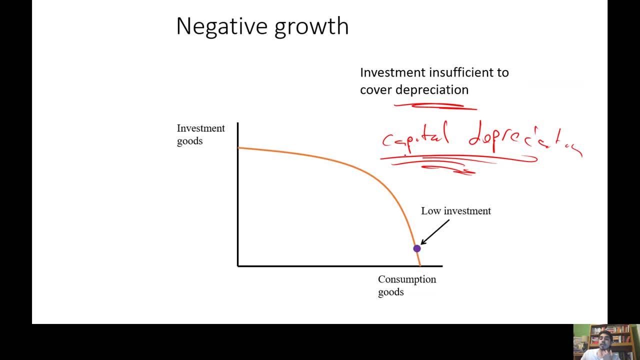 goods and in turn your economy, consuming a lot of couple of years. you might look it's called capital depreciation. you might actually get negative growth. so capital depreciation is like you should expect your capital equipment to get run down, uh to facial, um, you know, deterioration and all sorts of stuff, and so if your your your ppf point is over here, you should expect even 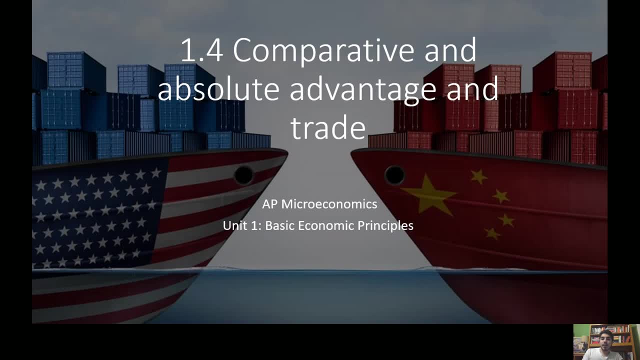 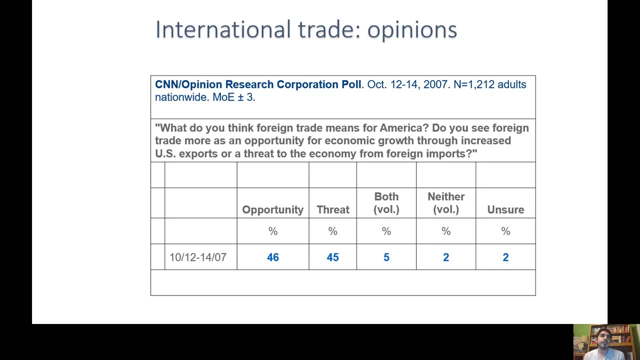 negative growth with capital depreciation. okay, now we're into comparative advantage and absolute advantage and trade. we talked about international trade. this is sort of, you know, delving into specialization and the benefits of specialization. we said international trade is not very popular in america. we talked about the protectionist policies of president trump and sort of the protectionist. 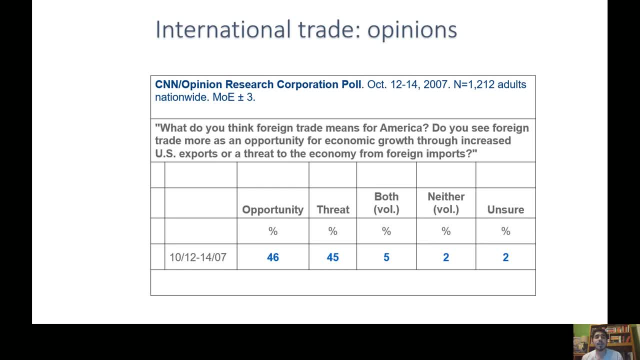 ideologies that exist across the political spectrum, specifically more so at the fringe, like towards the far left- left um of the democratic party- i'm talking about the bernie sanders of the world, um elizabeth warrens, and kind of the far right, um. well, i guess now more the mainstream. 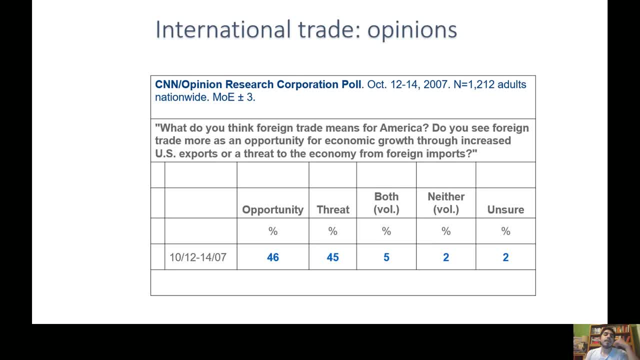 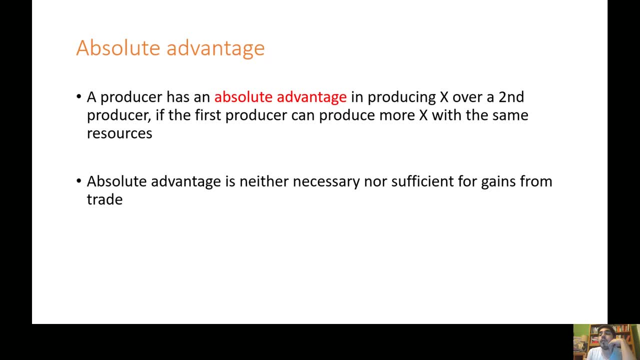 of the republican party in in donald trump and protectionist policies. they're not very popular or trade is not very popular. however, there are gains from trade, there are gains from specialization, there are gains um that can be attributed to comparative advantage. but to understand comparative advantage, we also have to understand what is absolute advantage. 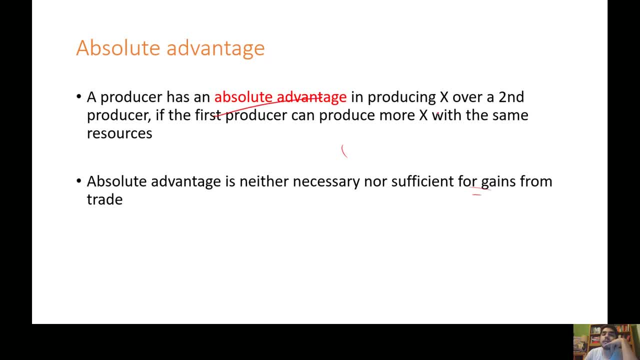 a producer of a good has absolute advantage in producing x over a second producer. if the first producer can produce more x with the same resources, so, um, with the same resources, they're more productive at producing x. that means that somebody has an absolute advantage in the production of x. cool absolute advantage is neither necessary nor sufficient for gains from trade. 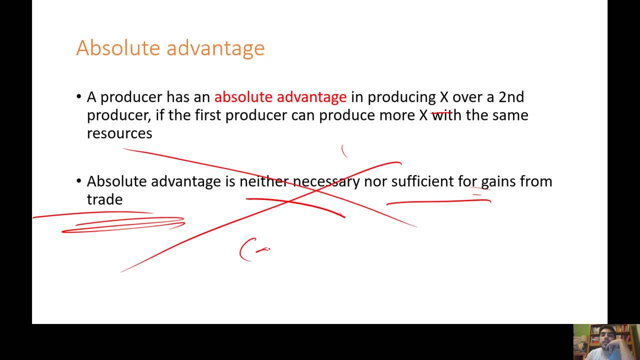 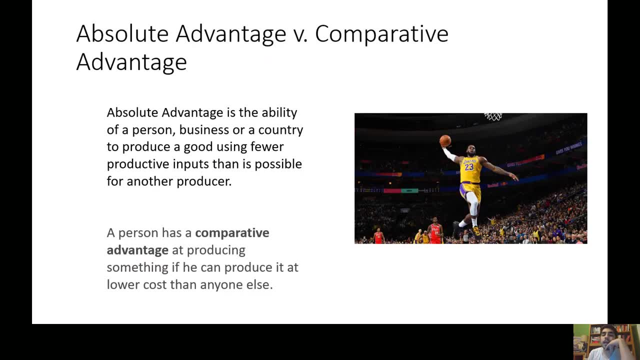 um, so it's not the big picture. what what's the big picture is? the big picture is comparative advantage. that's what we care about. nobody gives a crap about absolute advantage, and so we talked about this example of absolute and comparative advantage with lebron james um, and i'll leave it, or i'm not going to repeat that example here. but a person has 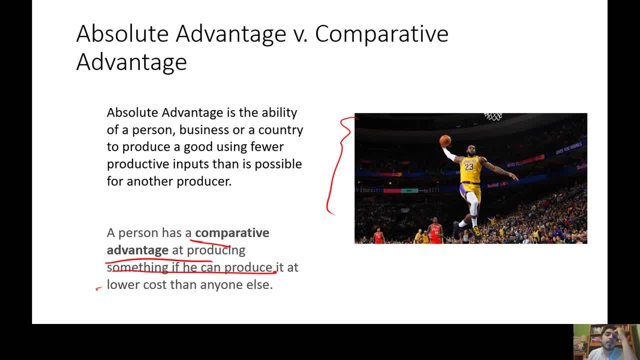 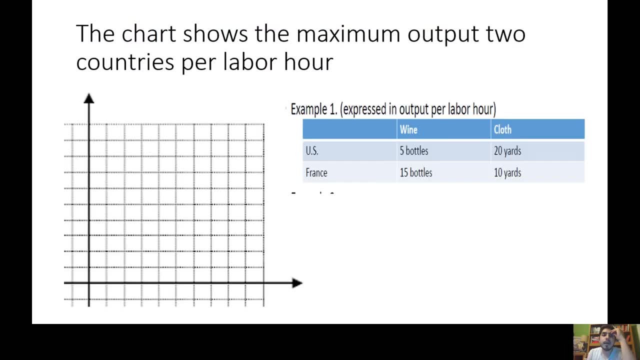 comparative advantage of producing something if he or she or they can produce it at a lower cost than anyone else. and so, specifically, um, i can do a example of comparative advantage, the principle of comparative advantage. there's a positive aspect to this and i shall say, i shall say this: there's a positive economic aspect to this because this: 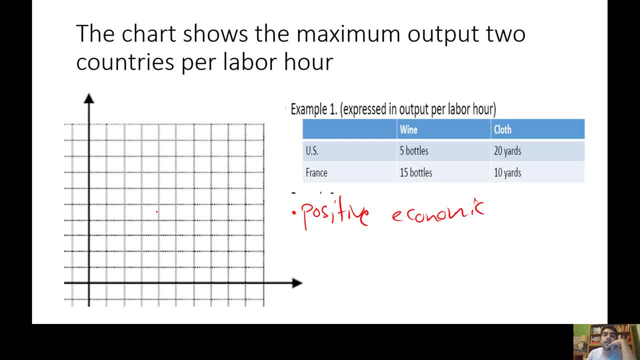 is very much an economic theory and it's a robust economic theory. we're going to use what is called the ricardian model to demonstrate the gains from trade and comparative advantage, or the demonstrate the gains can from trade that is attributed to um people or businesses or 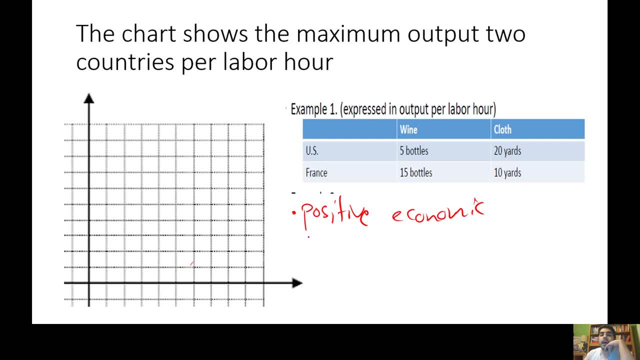 countries specializing in that which they have a comparative advantage in a positive economic- uh sort of um analysis, predict, prediction or description to to this in the sense that if a country signs a free trade agreement with another country, a economist might make a positive economic prediction using this sort of theory and in this sort of model, saying: 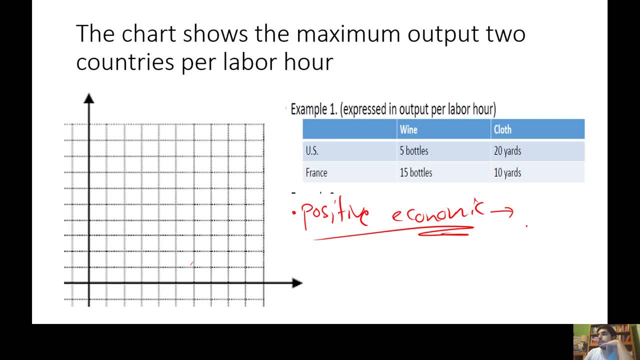 that um country a will specialize in that which they have a comparative advantage in and country b will specialize in that which they have a comparative advantage in. right, that's a positive economic description, right, and they might use this kind of theoretical model to explain why that positive economic description is true. and there's a lot of support for this. um countries tend 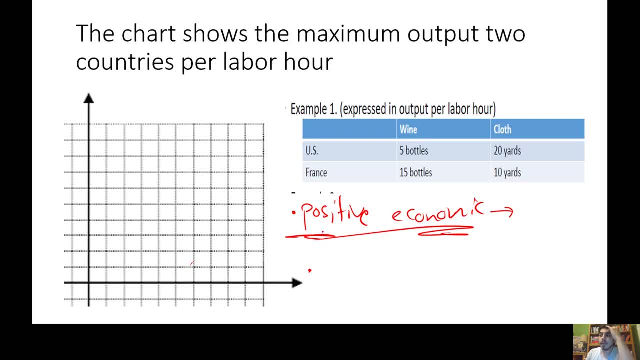 to um export that which they are more productive in um than other countries, and and they tend to import that which in which they are less productive than relative to other countries. we'll explain a little bit more, but there can also be a normative economic statement that 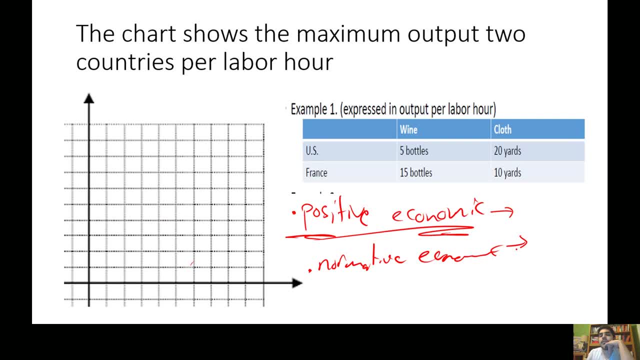 we'll explain a little bit more. but there can also be a normative economic statement that maybe an economist that you know is kind of ignoring, maybe international security implications or maybe political implications- might say: hey, the united states really should trade with china, and they should, you know drop making, um, you know steel, and they should just trade electric cars because 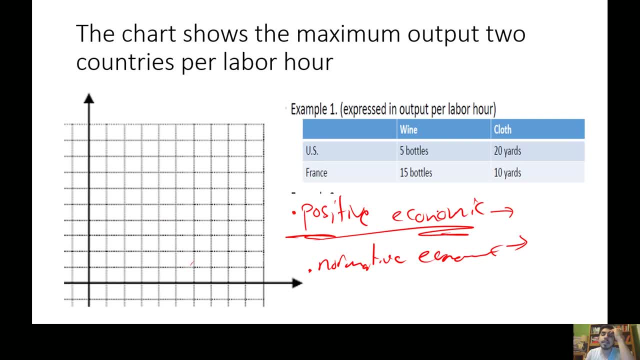 they have a comparative advantage in electric cars. and china should trade steel because this, would you know, lead to gains from trade. increase, uh, the ability for the us and china to both, um, you know, go beyond their production possibilities, frontier um and acquire more, more um goods and not acquire more goods. but 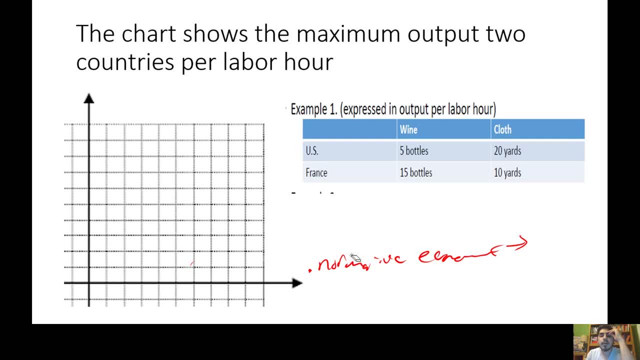 to be able to make goods and and make the good that they're good at, and be able to trade that good for goods that the other country is specializing in at a lower opportunity cost than if they were to make. that we'll go, we'll get into it, okay. so 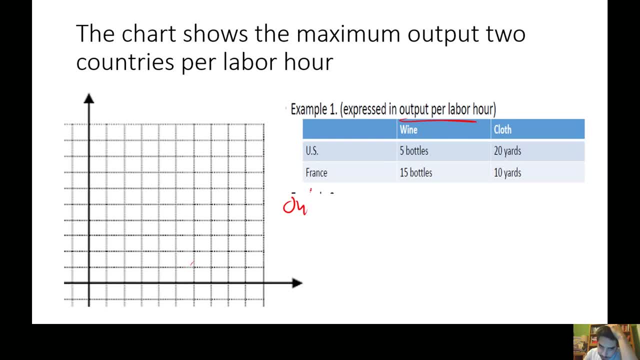 this is an example. this is output data. i'm going to show us a shortcut to find the per unit opportunity cost, because we want to find the per unit opportunity cost to be able to compare countries opportunity costs and to be able to um determine which country has a compare for advantage. 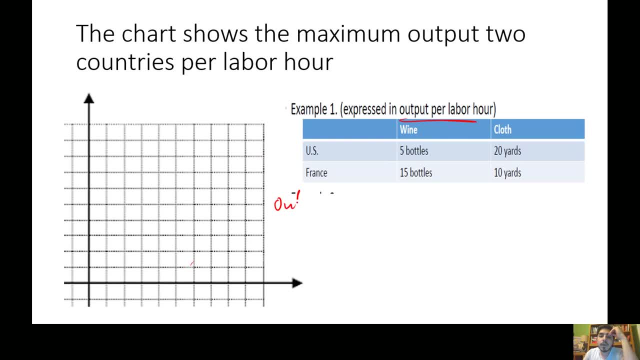 and not for benefit to can computing generally. which country? which right hand hand line, middle hand and left hand, Jeff? um, you should use the hex thing, which is to say the vertex range area. you should also use the hex you left and right hand side linear graph. that's whatわか. 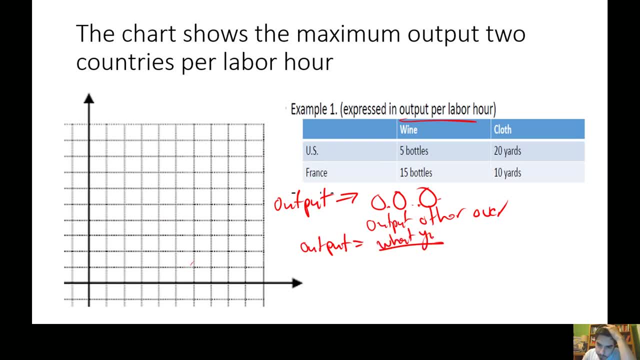 you for measuring benefits and we're focusing on learning what y what you see here, but you don't know what an output is. in the numerator i put what you give up over what you get. this is the formula for finding per unit output or, i'm sorry, the up the. 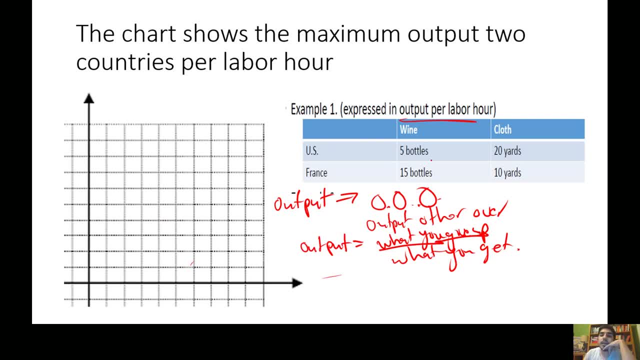 per unit opportunity cost. so per unit opportunity cost is for one bottle of wine. how much cloth do you give up? and the reason why you want to do that is so that you can be able to compare with the per unit opportunity cost of of france to determine who has the. 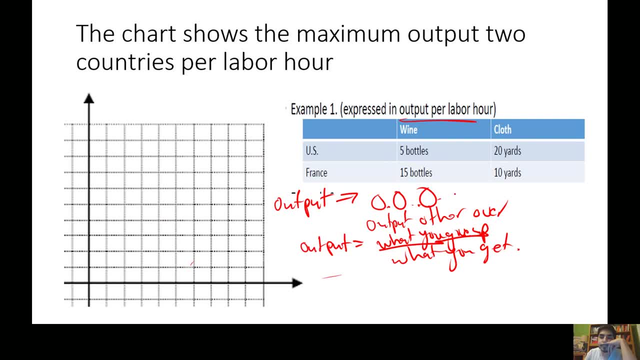 the lowest opportunity cost and therefore the comparative advantage. so five bottles of wine. so to find the per unit opportunity cost. given this, you put what you give up in the numerator. so 20 yards of cloth. don't have to put the units yet. and then what you get, so what you're going. 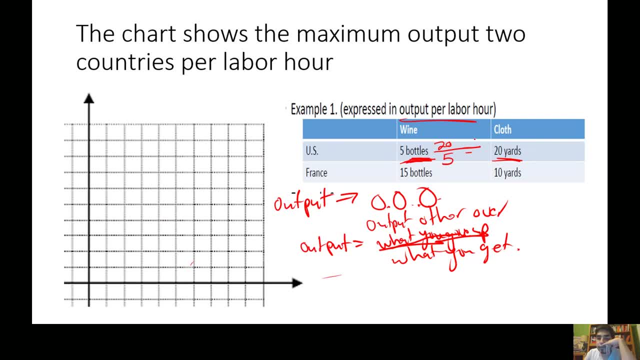 to produce and specialize in. instead, 20 divided by 5 is 4 yards. so for one bottle of wine, the per unit you can write it out- oc is four. oh, All right. All right, And you get the Javelin, But i'm not going to write that out. so that's four. 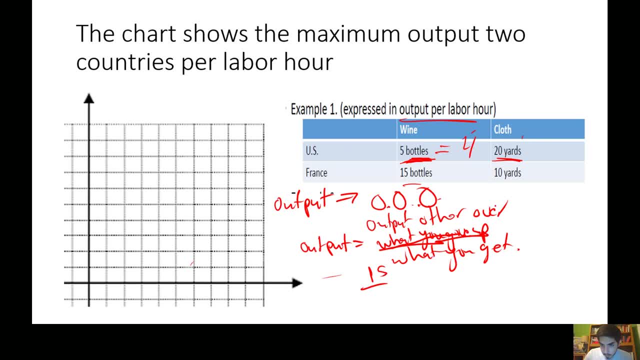 for one bottle, because we can't compare this for one bottle of wine for france. again, we use the formula what you give up, all right, so that's four you give up, or the other over, meaning the other in the numerator. so what you give up, we put the 10. 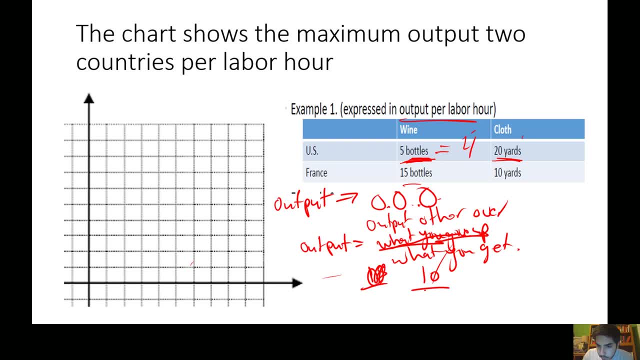 sorry, 10 in the numerator over 15, simplify five. oh, what the hell did i do? sorry two and then three, two-thirds yards. did i do this right? 20 divided by 5, 10, yeah, two-thirds yard. and so who has the lowest opportunity cost, meaning who gives up less? it's france. 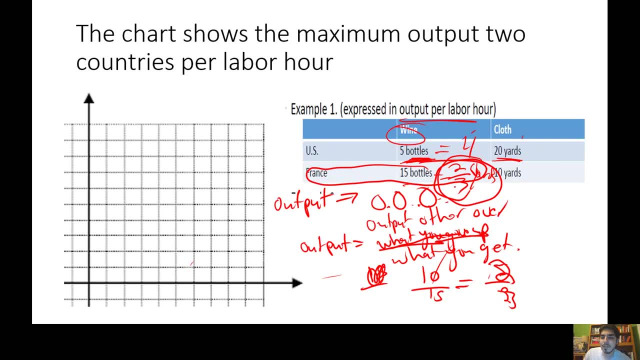 and so therefore france has the comparative advantage in the production of wine, kind of a little racist, uh problem, not a racist problem, it's kind of funny, a little stereotypical, i mean. and then, um, um, four, four yards is a higher opportunity cost than than france's two-thirds yards, and so 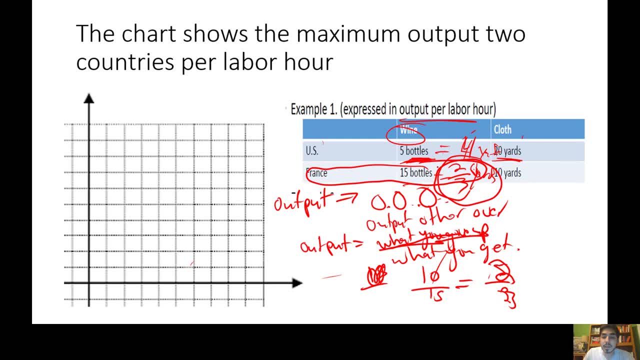 this means that the us- uh, because the comparative advantage you can have the absolute advantage in both goods, but the you can only have the comparative advantage in one good. there's some situations where there's no comparative advantage and we'll talk about that in a bit. it's just that the slope of the ppf, so to say. 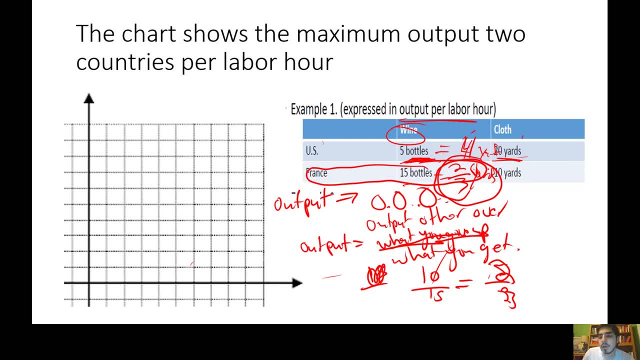 um, but oh, or i'm hint, hint. i'm going to put a word problem on that for the in the reveal, um, but i can, i can show you these, but i'm not going to. but you'll see that the opportunity cost for the us and cloth is going to be um, um. 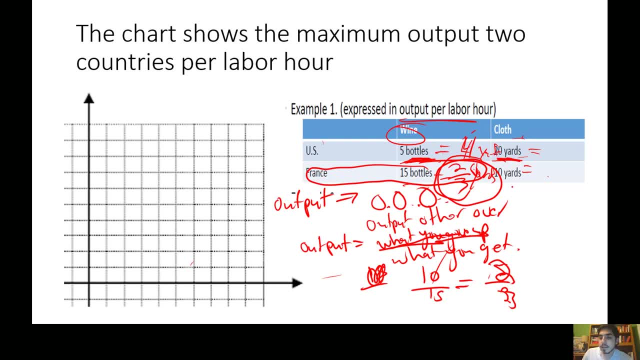 smaller than the opportunity cost for, uh, france in in cloth, and these are actually the reciprocals. so this is three half and four, so it'd be one fourth. so you can see one fourth is actually smaller than three halves because these are the reciprocals and you can do the little mental. 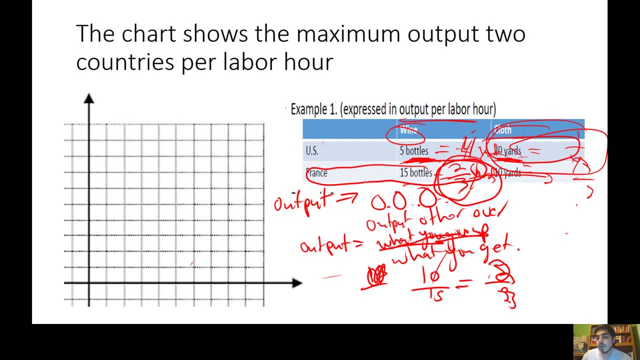 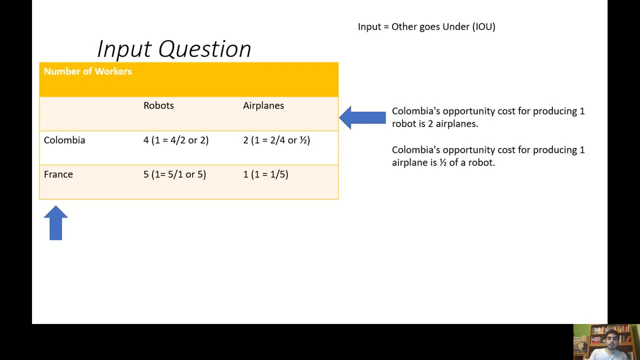 shortcut to see that they're the reciprocals. but just know that if you have the comparative advantage in one good, you can do a full stop and find the comparative advantage of the other good. okay, we did input questions, so this is an example of an input question. 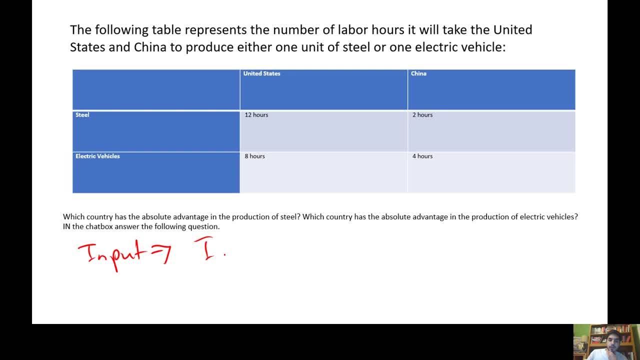 and for input questions you can use this sort of mental shortcut: i o u input other under and then what i i would just memorize is that for input questions i would definitely just put: um, just remember what you get over, what you give up. of course these mental shortcuts are defined. the per unit opportunity cost of a good 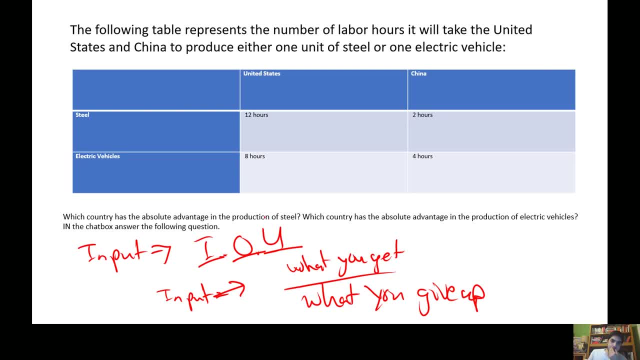 or service. but first i want to talk about absolute advantage. um. so in input questions you have to be a little bit careful. um. so an output question- whoever has the absolute advantage in something- would obviously be producing more units. but an input question- whoever has the absolute advantage in something is producing, um, those units in less time. and so it's clear that china and the 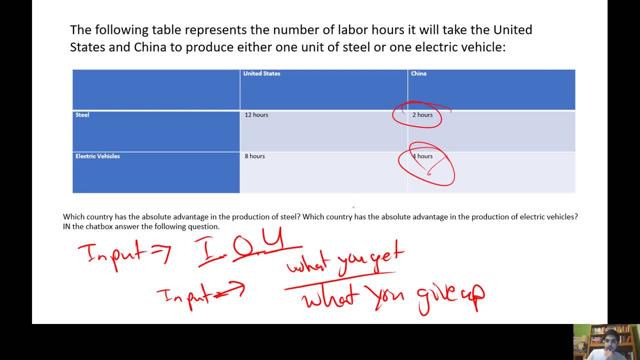 united states have the absolute advantage in the production of both steel and electric vehicles, but because they only take two hours and four hours it will take the united states to produce either one unit of steel or one electric vehicle um to to produce one of both. but this doesn't. 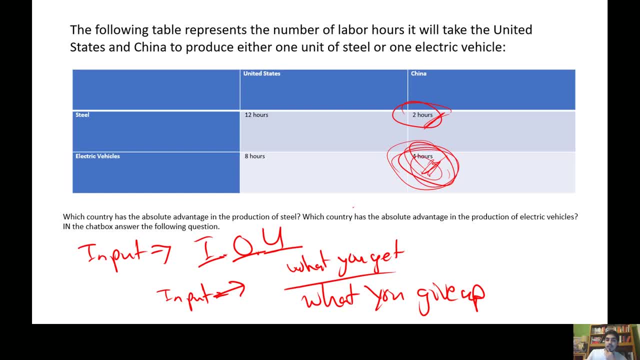 matter. this does not mean that you, china, should specialize in both of these things. um, an economist might make a positive prediction if, that is, if china and the united states were to engage in completely free trade. uh, that, um, you know china is going to, um, you know, exchange and export to the united states and specialize in the production of that. 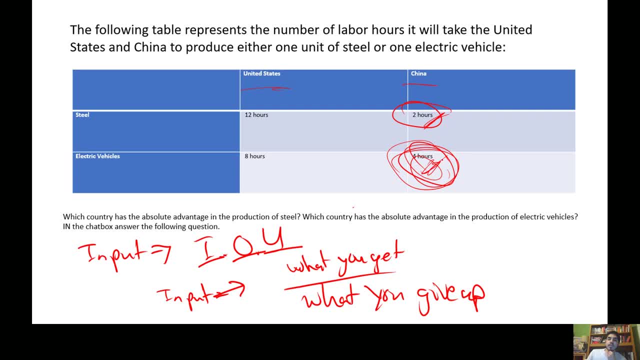 which it has comparative advantage in, and the united states is going to specialize in the production of that in which it has comparative advantage and all sorts of stuff. or an economist might make an enormous statement saying that china, um or the united states needs to stop wasting resources and and trying to um give um steel, are trying to to special, trying to 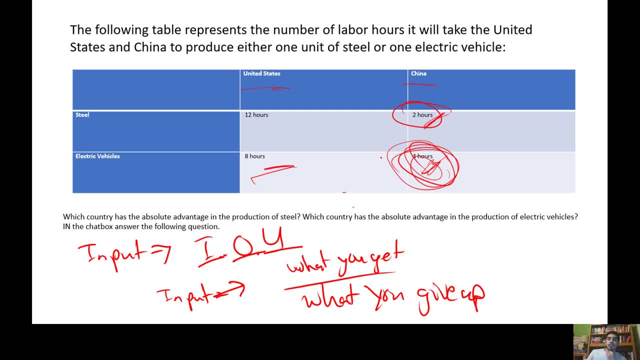 produce steel and should just reallocate all resources to produce steel in the production of electric vehicles. um, oh, but i give, i gave it away. so to find the per unit opportunity cost, and remember per unit. so one unit of steel opportunity cost is what you get put in the numerator. so what are you getting? 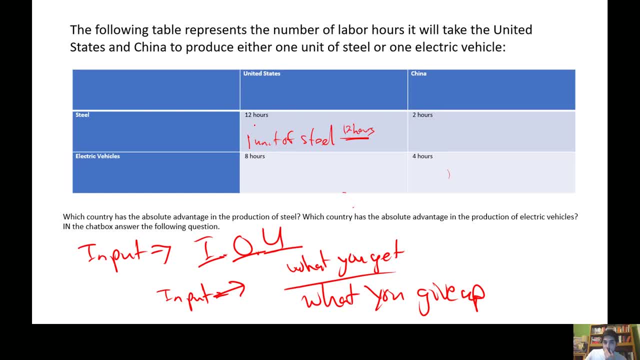 you're getting, or put the, the input value of, or the in. here we have, like the labor hours it takes to one. make one unit good, the input value of what you get, which is the steel, over what you give up, which is the electric vehicles. simplify by before: three, halves right, so one unit of steel, the opportunity cost is three. 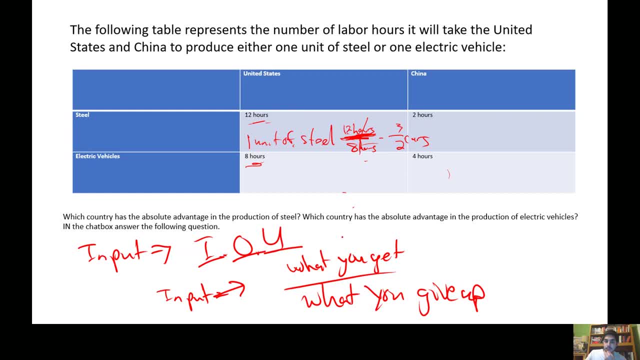 half vehicles or cars, cool until it comes up in the final unit. so that's at least not everything. if you mention this, suppose, if you just do like a five Gore unit plus you give up, that would be zero and that would be thirty four. so that's kinda just measure, uh um. 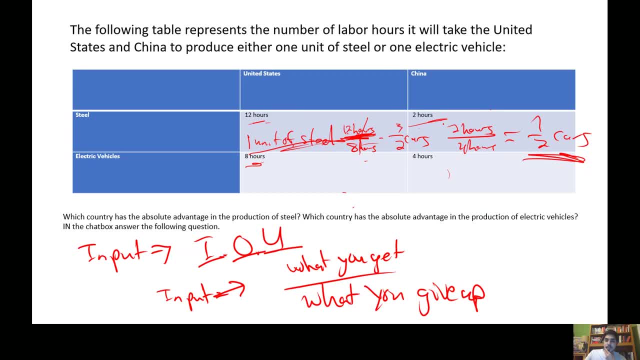 per unit opportunity cause. so it means per unit opportunity class for china. what you give up or what you get, is what I meant of sense, because you can see that it takes that this would make sense because if china were to to, you know, make one unit, which is what a per unit opportunity cost is. 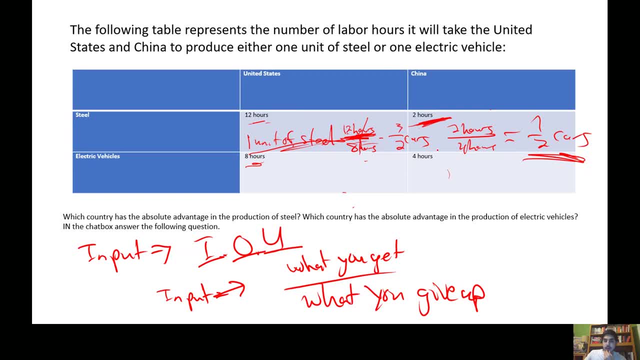 then two hours. they would all. they would only take them two hours and they would only have two hours. right, that would be worth half a car, which is lower, half or one and a half. the lowest one is half a car. so that means china gives up less, so, despite the fact they have the absolute advantage in both, it means that china should. 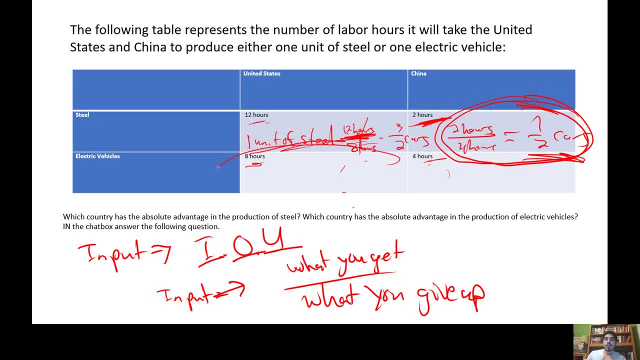 specialize in the production of steel and the united states should specialize in the production of electric vehicles. if you don't believe me that the opportunity cost of the united states is lower than china's opportunity cost of producing electric vehicles, please just run it. do the formula, plug in the numbers, but also know that this is just the. 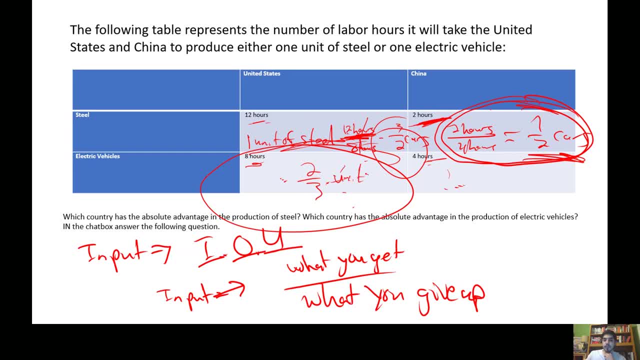 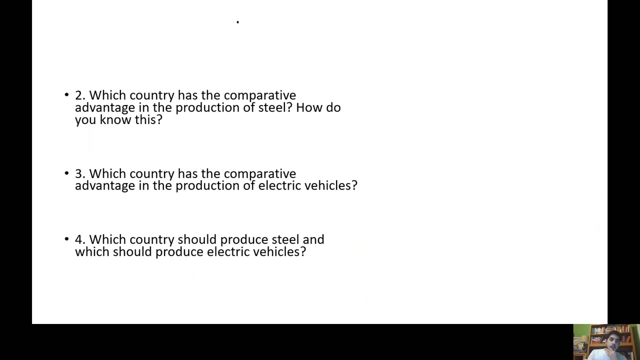 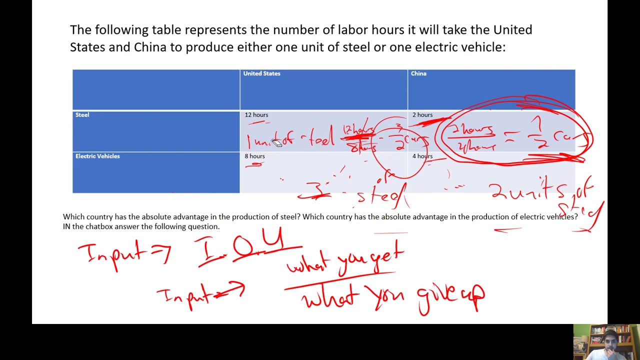 reciprocal: two-thirds units of steel is the per unit opportunity cost of producing one electric vehicle and then producing one electric vehicle for china. the opportunity cost is two units of steel, the per unit opportunity cost. and two-thirds is smaller than two units. cool, okay, answer the questions. boom. should i do a ppf to show the gains from change? should i do a ppf? 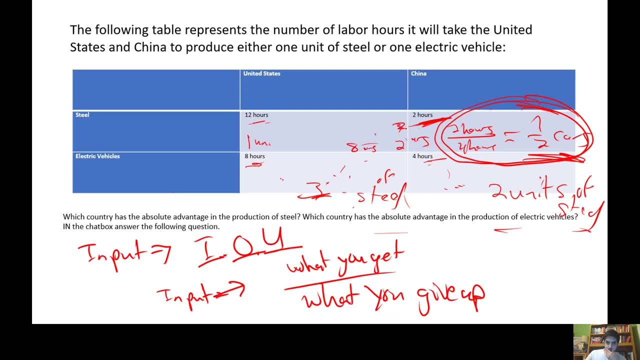 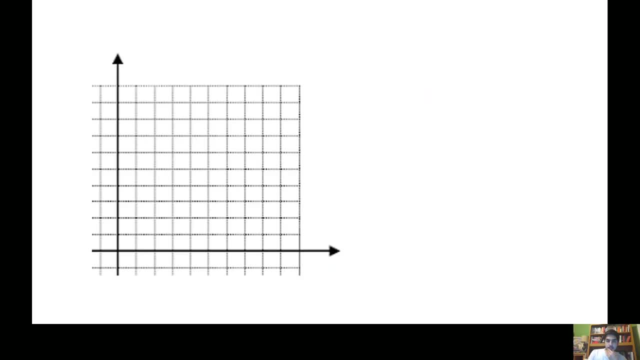 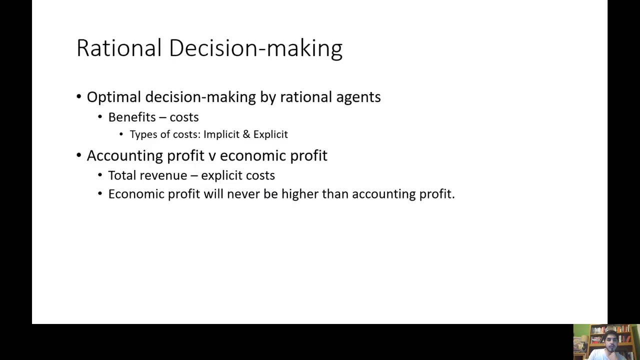 to show the gains from trade, um, so sort of. i'm going to keep these opportunity costs so you can see them per unit opportunity class, um or no, i'm not going to do show conceptually the game from trade here. i already showed it in class and then it gets complicated and you all 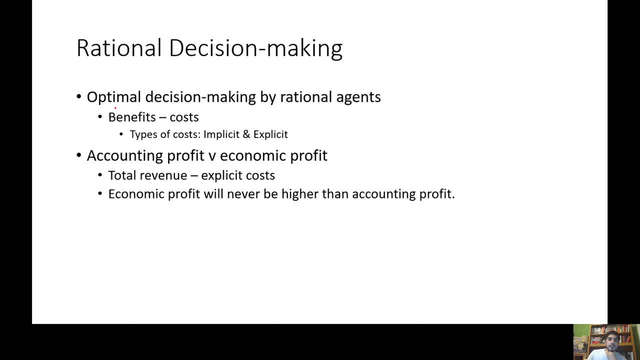 get lost and it's not relevant. so rational decision making. so we assume rational decision making. rational decision makers do what is called um our cost benefit analysis. so they consider the benefits of a choice and they consider the costs. so we said earlier that in economics there are 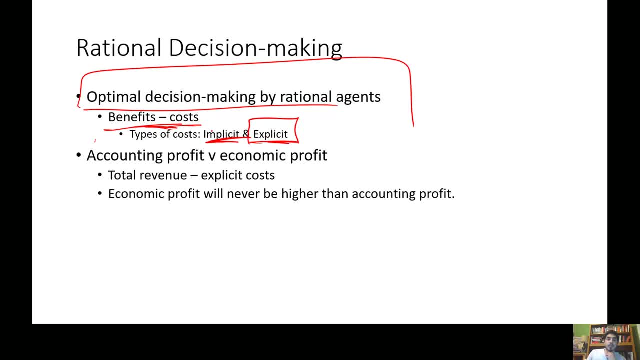 explicit costs there. there's a cost for going to the movies, the ten dollar movie ticket, the gas money, their implicit costs. implicit cost is probably one of the most important concepts in economics and the implicit cost is an opportunity. it's the only way you can measure the cost you. 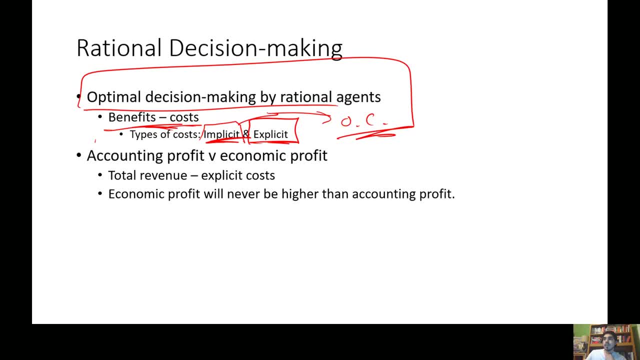 the cost, it's the value of the best foregone alternative. so in addition. so the concept of no free lunch is saying that you know you're giving up time essentially, and so for going to the movies, there's an implicit cost associated with going to the movies. so, for example, for me, 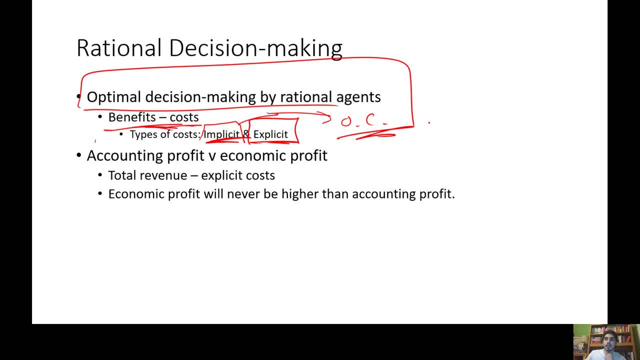 i can go to the movies or i can teach saturday school. right, there's a cost associated with me going to the movies because, um, i could have made 40 teaching saturday school, and that is the value of the best foregone alternative, so that 40 would be added to the 10 movie ticket. 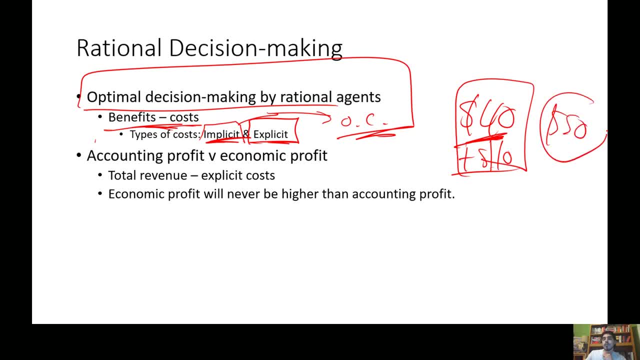 and that would be equal total costs, so 50. so we have the value of the explicit cost would be the 10 movie ticket and the implicit cost is the value of the best foregone alternative or the opportunity cost, the 40 that i could have made but i chose not to. that equals the total cost. 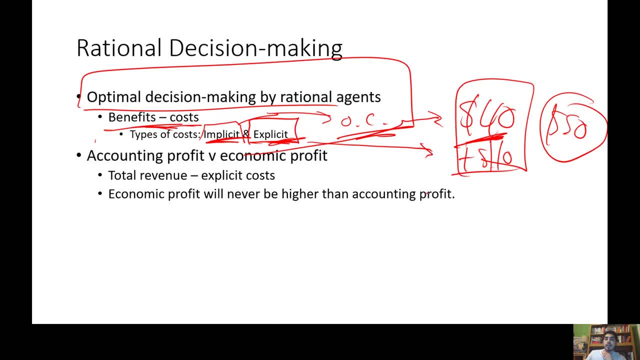 and so when conducting cost benefit analysis, a rational agent conducts cost benefit analysis um and and makes decisions based on that, and my benefit in theory is supposed to be greater than this. 50 accounting profit versus economic profit. accounting profit is total revenue minus explicit costs, so accountants are only concerned with explicit costs, but economic profit is always. 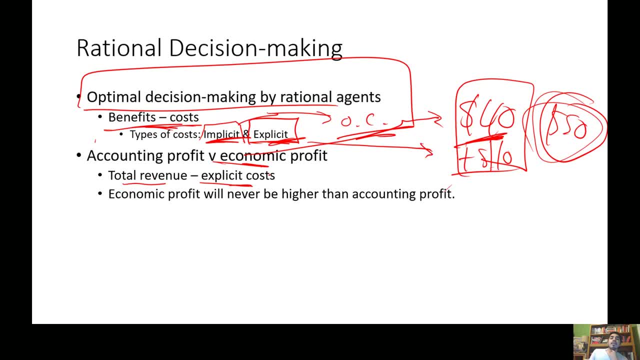 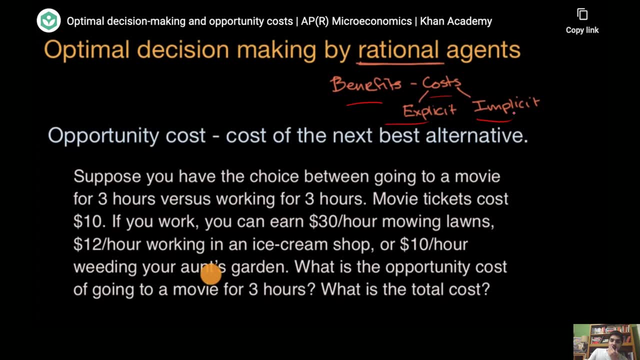 going to be lower than accounting profit, because economic profit considers the value of implicit costs. so let's look at an example. con academy, don't sue me. here's an example of benefits and costs. explicit and implicit opportunity cost is the cost of the next best alternative. so in this example- suppose you have- 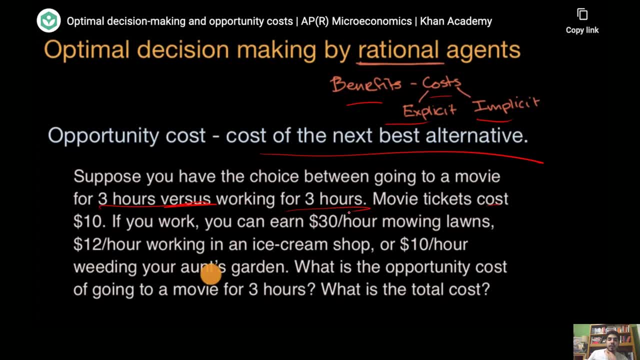 a choice between going to a movie for three hours versus working for three hours. movie tickets cost ten dollars. if you can work thirty dollars per hour mowing lawns, twelve dollars are working ice cream shop. or ten dollars an hour wedding your aunt's garden. what is the opportunity to cost of? 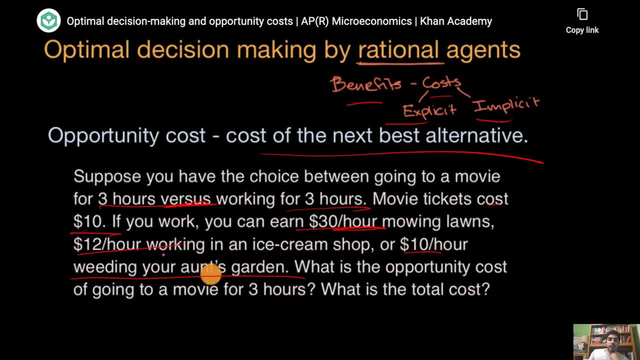 going to movie for three hours. so, first of all, the opportunity cost of doing anything is not the sum of all the alternatives that you could have done. no, it's the value of the best alternative you could have done. and the value of the best alternative you could have done is the 30 hours. 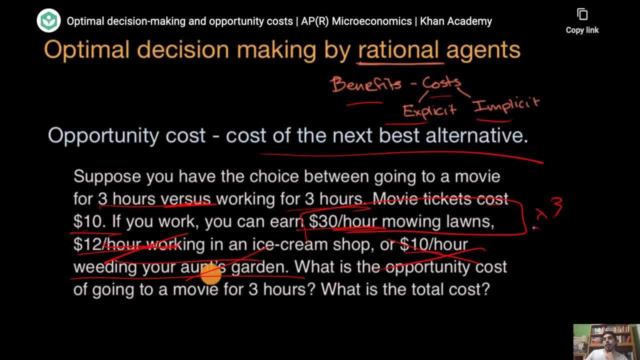 an hour mowing lawn and we know that we're watching the movie for three hours. so that's 90. so the opportunity cost or the implicit cost of going to the movies is 90 bucks. what is the total cost? remember that total cost is explicit plus implicit cost, and so the explicit cost is 10 bucks. 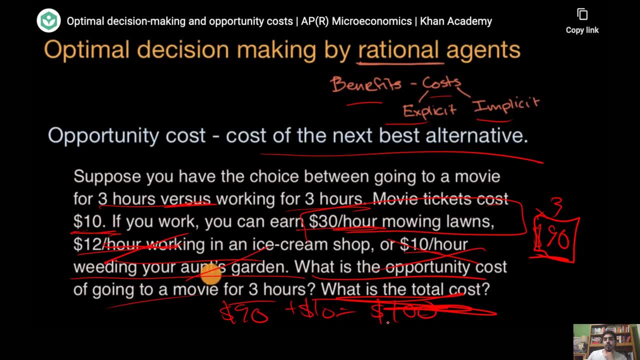 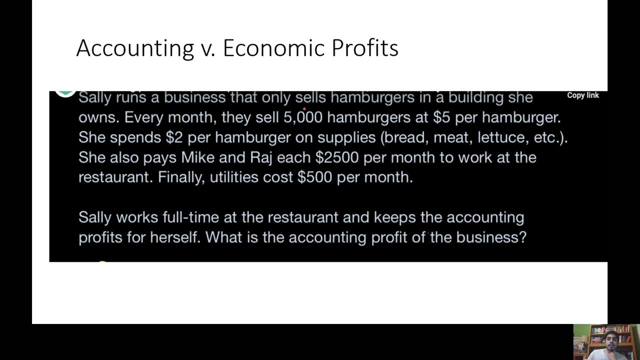 of the movie ticket. so it's 100 bucks now. an accountant would only care about the 10 loss. an economist cares about the implicit cost or the opportunity cost, the value of the best work on alternative. it's an example of accounting versus economic profits. every month you sell 5 000 burgers at five dollars per hamburger. she. 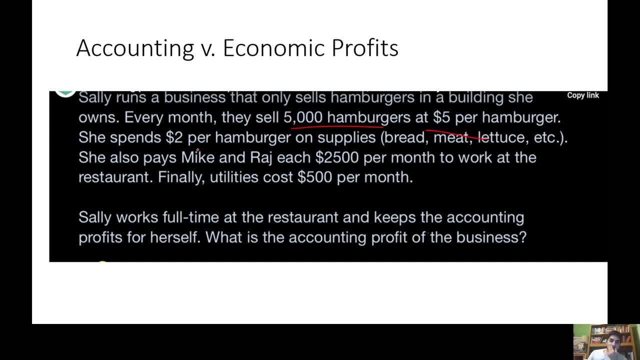 spends two dollars per burger on supplies. she also pays 2500 per month to two people and then utilities cost 500. so an accountant would only care about the 10 dollar loss and an economist would only care about the 10 dollar loss. and an economist would only care about the 10 dollar loss and an 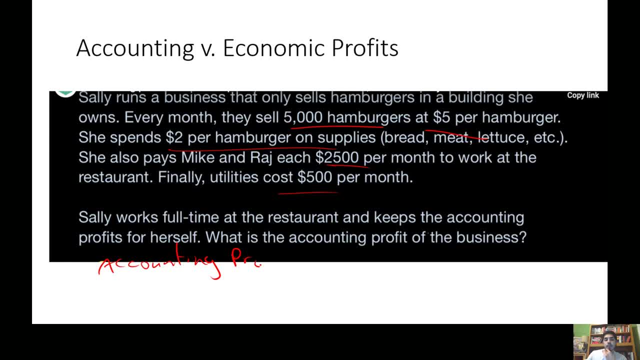 accountant would only care about the 10 dollar loss and an economist would only care about the 3 dollar loss and about the 10 dollar loss and an economist- both accountants- would only care about the 10 dollar loss and would research both services, including health care facilities and other 라. 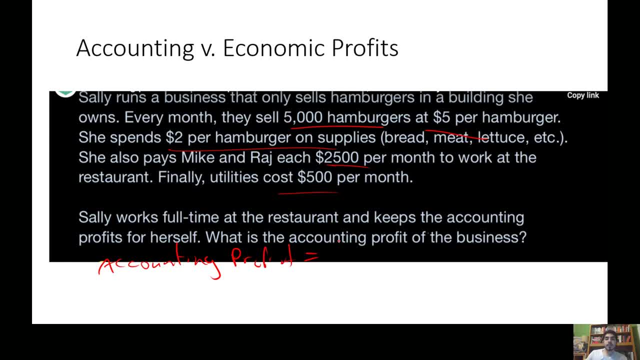 so this is again a inicial cost. Scotland has been working on funding Washington to mid Channel, so it's a normal business item like homebrewing food. all right, we know that many vision would be if we spent that much B's. we would still be good if we spent, you know, $People thought Mount Entre to the 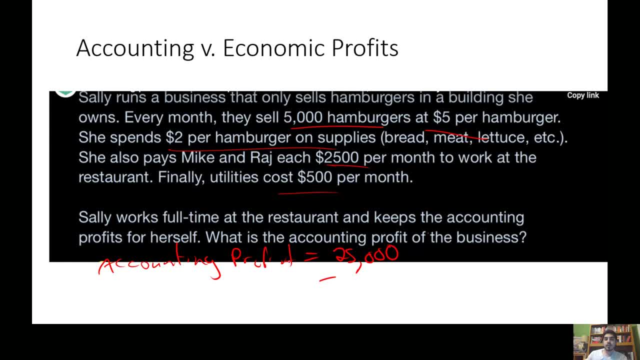 building. they would be bad. so we need to have a B's team, because it is pretty good to do a lot more finishing worker positions, and so you know what we're going, where we can use wider brands. so I think we're going to go ahead and 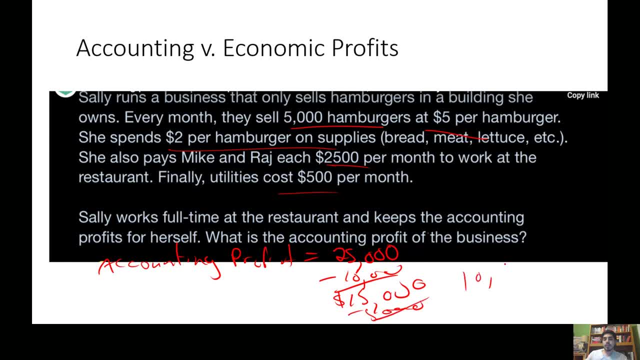 see if you want to invite, uh, some of our technical partners to join about something. what you would like to know more about it for sure 10 000, and then we have 500 in utilities, so we're left with 9 500 in accounting profit. 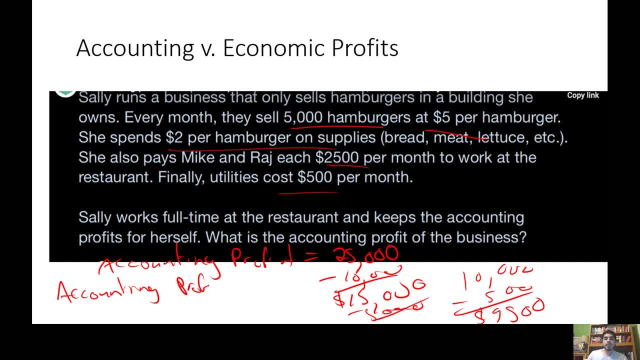 accounting profit's good, but we care about economic profit. this is intro to microeconomics. right, and let's say that sally could have worked, that she has a law degree and she could have been making ten thousand dollars a month. all right, that's the value of her best forgotten alternative at a law firm, then her economic profit. 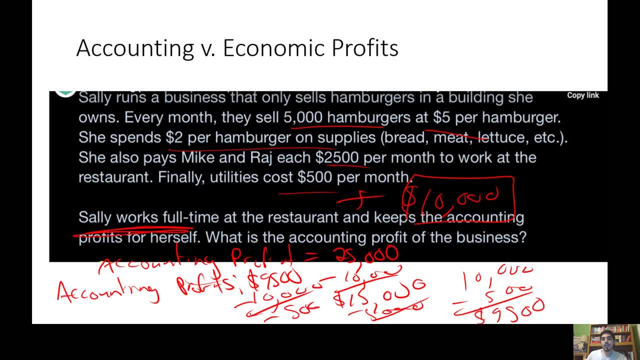 so minus ten thousand is actually negative five hundred, and so, um, assuming, uh, we don't know, maybe she has sort of benefits associated with this, but this wouldn't seem like a rational decision to make. um, assuming that she didn't really care or she didn't really have a 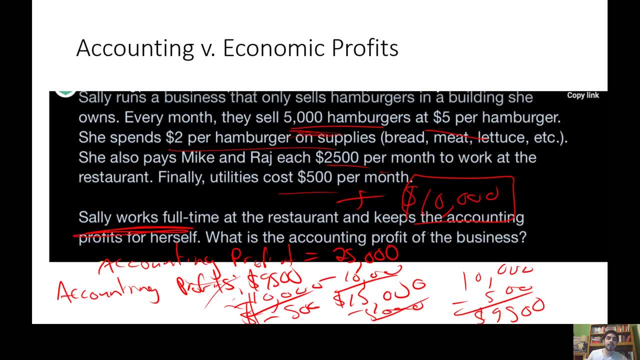 preference for work. she didn't really care for her job. she didn't really care for her job. she didn't care for her job. she didn't really care for her job. she didn't really care for her job. she didn't work in a hamburger shop, over a law firm, and she was just trying to maximize. 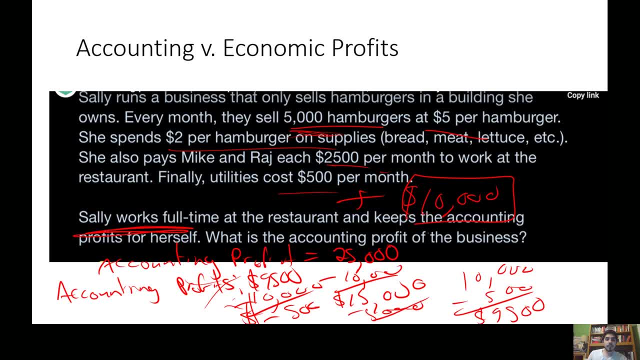 the economic profit right. this wouldn't be a rational decision because economic profit is counts for implicit costs. but if it was like she could have made 5 000 a month, then we would just subtract it from 9 500 and then her economic profit would be 4 500. 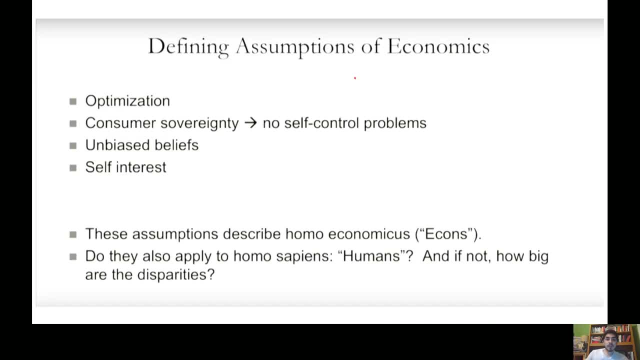 that's how we consider economic profit. so assumptions of microeconomics. this is what something i took from richard thaler- i'll include him in the video description, a lecture on richard thaler. he goes and models of economics kind of assume rationality like nobody does this cost. 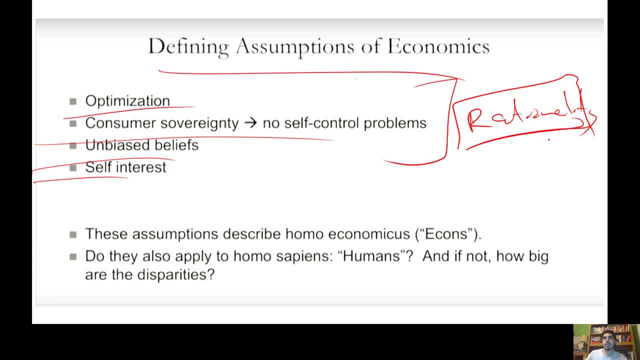 benefit analysis explicitly. nobody thinks like, oh, what are my costs, what's my opportunity to cost. but we do do it intuitively, we do kind of have a sense, we kind of have a rough back of the envelope type assumption. and so these assumptions about you know us, you know being rational agents, it's called homo. 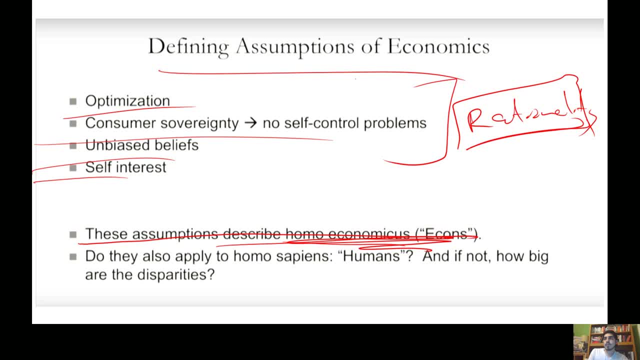 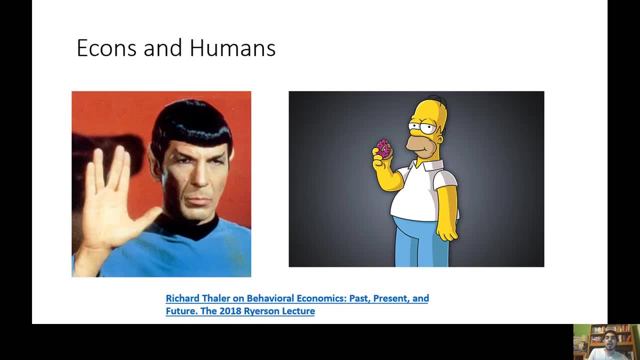 economicus, um, but i think it's really important to think about these assumptions and i think it's really important to ask ourselves tomorrow: um, are i really Pablo 150? think we do that this day? or do we only trust a computer? i don't know if it's like that, but it onto others. 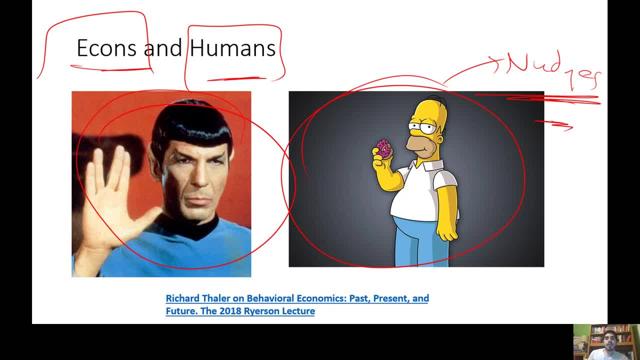 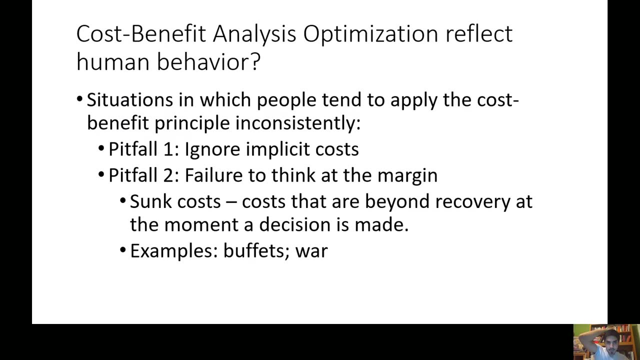 new research on nudges, which we'll talk about at the end of the year. But for right now we're just going to build a lot of models, assuming rational consumers and rational producers. Cost-benefit analysis optimizations reflects human behavior. There are certain pitfalls in 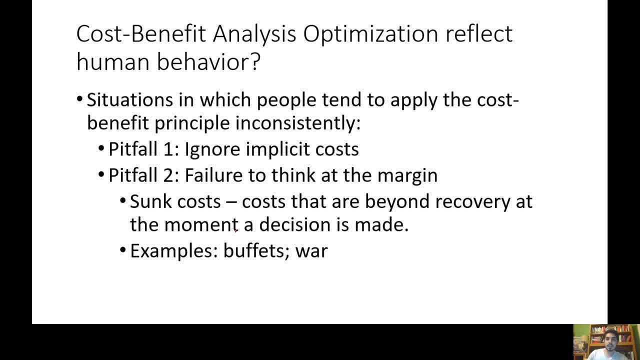 situations in which people tend to apply the cost-benefit principle consistently. We talked about this. They ignore implicit costs. They focus on accounting profits And then the failure to think at the margin. So sometimes a lot of them will consider sunk costs. So an example would be: 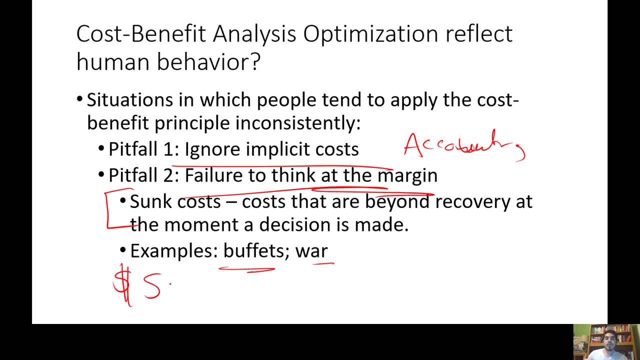 a buffet. So sometimes there's a $5 buffet fee And sometimes if that fee gets waived for like 20 customers, it shouldn't matter. You should still expect the same conduction for 2,000 customers And 2,000 customers have to pay. 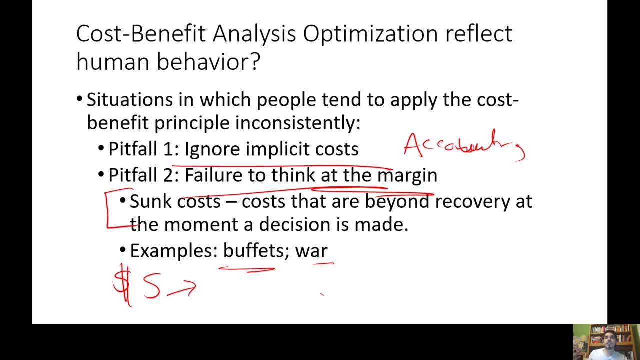 that $5 fee, You should still expect the same consumption patterns, because it's a sunk cost. It doesn't matter, right. What matters is decisions at the margin. What matters is decisions at the increment, in terms of determining the amount of utility you want to get out of something. 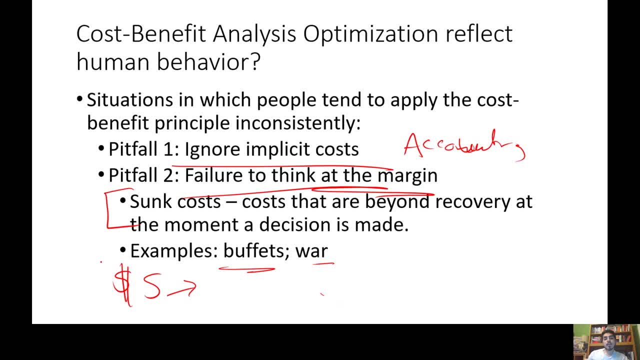 the amount of happiness you want to get out of something and stuff like that. But psychologists have shown- and behavioral psychologists in particular point to this- that that $5 actually matters a lot And that people that have to pay this fee actually tend to spend or try to eat as 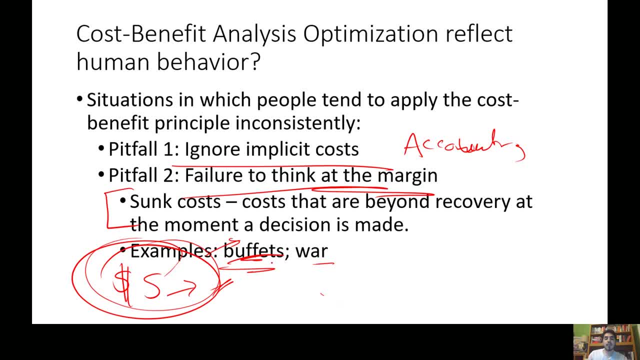 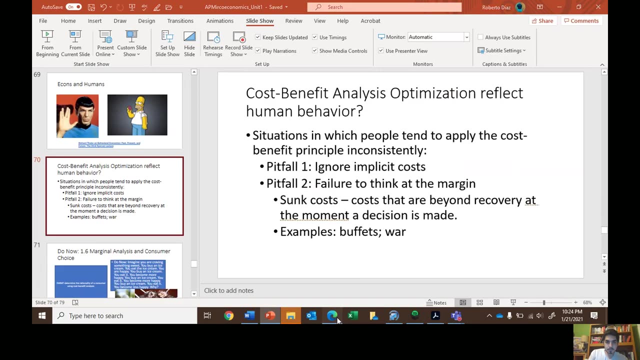 much as possible at buffets, And so that's one of the things that we're going to talk about today. Another example is war and conflicts, And so I'm going to go to this because there's a cool Justin Wolfers. he was quoting a Donald Trump tweet and he was talking about the sunk cost. 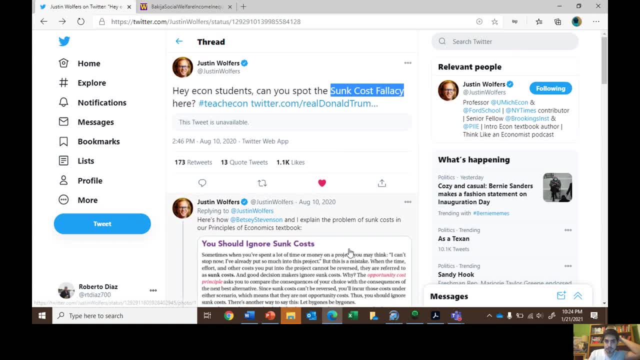 fallacy, And so I'm going to go to this because there's a cool Justin Wolfers. he was quoting a Donald Trump tweet and he was talking about the sunk cost fallacy. So sometimes politicians use the sunk cost fallacy. Obviously, Trump's Twitter account has gotten taken down, But there are other. 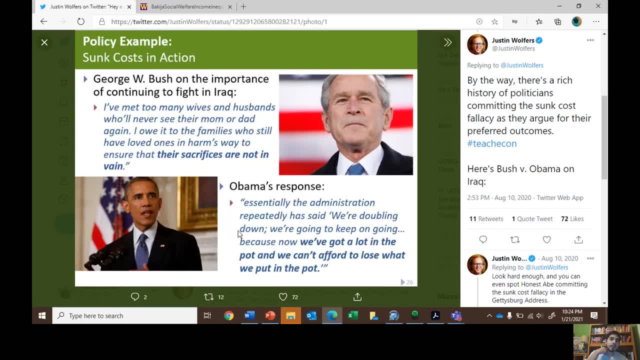 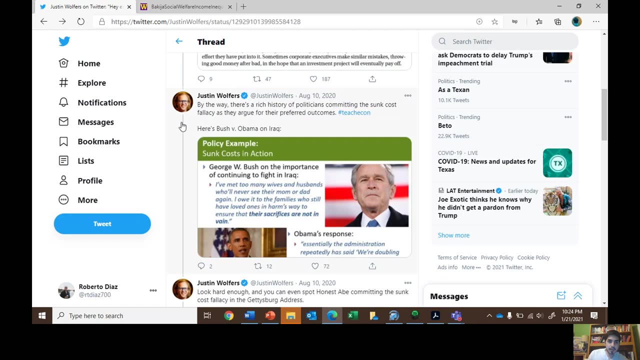 examples of sunk cost fallacies in like foreign policy. So these are examples from Justin Wolfers slides. He's a fellow at the Peterson Institute of International Economics, He's a professor at the University of Michigan. And so, George W Bush, you can see here I've met too many wives. 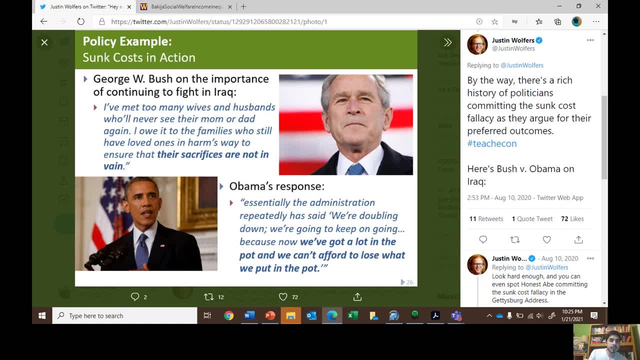 and husbands who will never see their mom or dad again. I owe it to their families, who still have loved ones in harm's way, to ensure that their sacrifices are not in vain. Obama kind of talks about the same sentiment, But that's not rational. 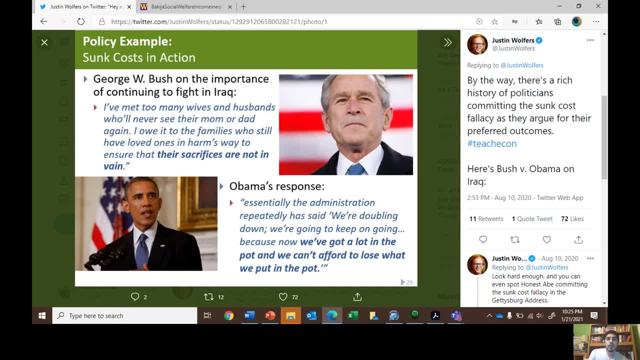 That's not maximizing. That's not considered rational according to economists. That's not making decisions at the margin. This is a sunk cost. The sacrifices of these people's lives and the resources are a sunk cost and you should make decisions at the margin. according to economists, 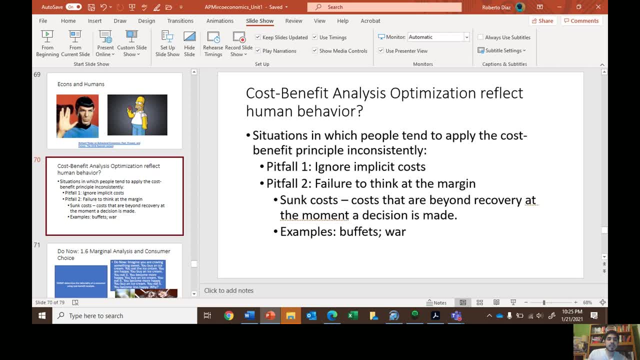 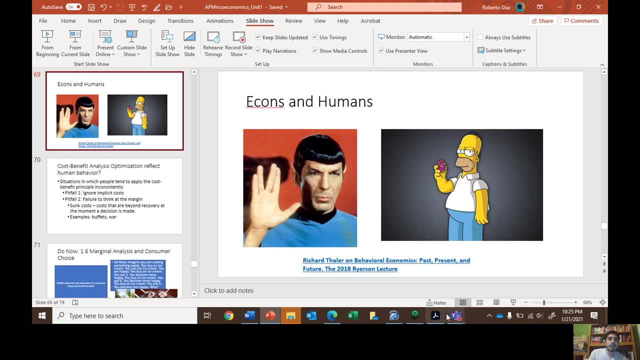 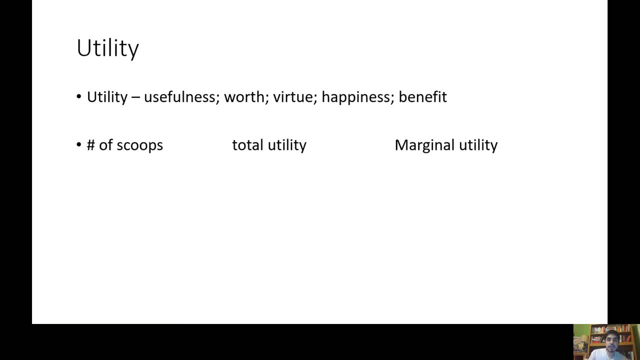 I mean, not all of us are like that, And so there's a sort of Spock-like- you know, character to the rationality models that economists build, But don't worry about that so much. Okay, then we talked about diminishing marginal utility. So we talked about this in class. 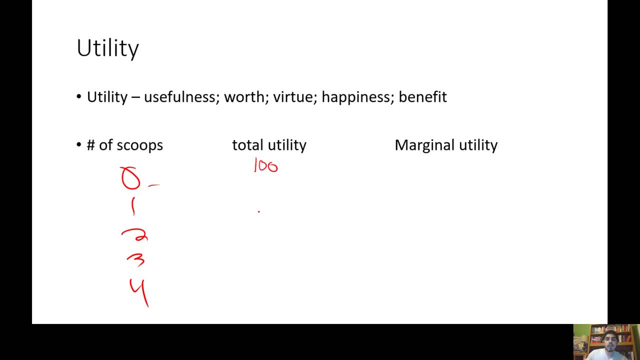 So we said, with each additional scoop of ice cream you might get a total utility of 60 points, 100 points, 100 points, points, 120 points, 140 points, 120 points, 110 points, And so total utility reflects. 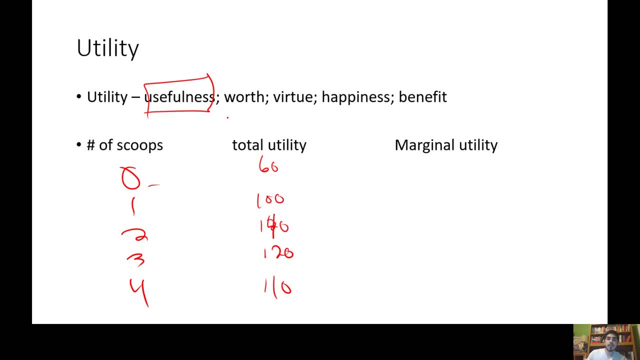 utility as a concept. So we talked about costs in the cost-benefit analysis. now we're going to talk about benefits in the cost-benefit analysis. Utility is a kind of amorphous concept. you mean happiness benefits worth. The previous economics teacher called them happiness points. 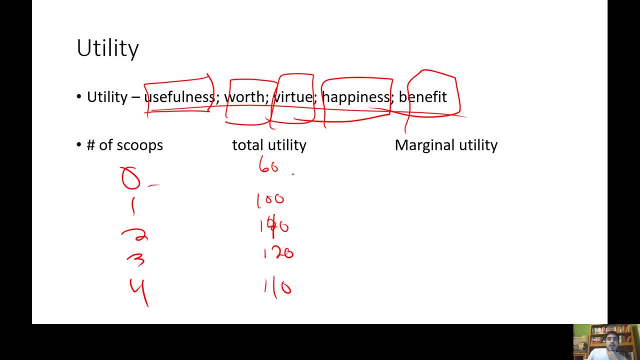 so if you want to call them happiness points, you do that. It's just a concept that is supposed to really kind of reveal that there is a lot of subjectivity in terms of what we value and the preferences we value. There's a whole economic literature or a lot of economic philosophers. 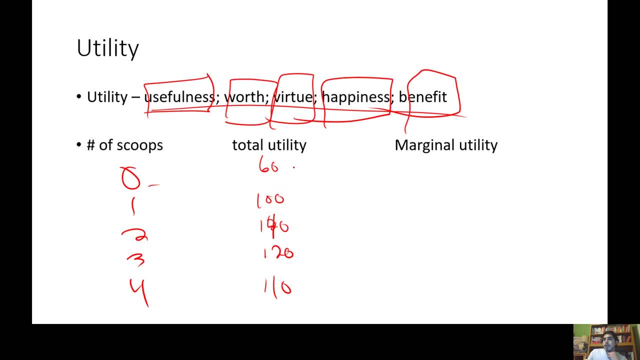 for a long time were trying to determine what went into the pricing of specific goods and services, and they thought it was labor. And, yes, labor is important, but what is probably also important is just like subjectivity and arbitrariness, right, Sometimes we value very like things that you know. 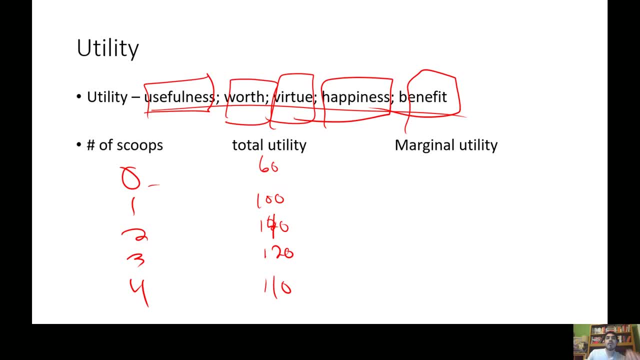 don't require maybe a lot of labor to produce or don't require a lot of inputs, but we value them nonetheless and we can have eclectic values and maybe even problematic values as well. So our utility functions look different for different things. We all value and gain happiness. 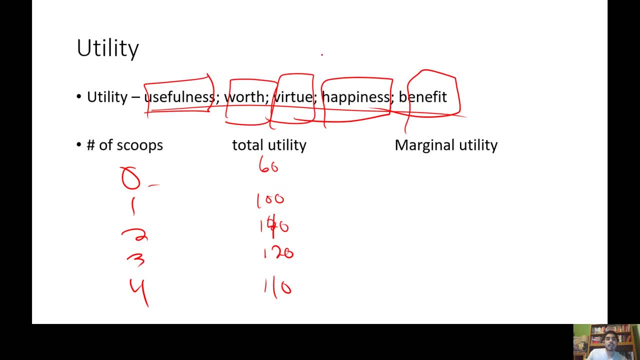 from different things, but we assume rational agents are trying to maximize utility. So utility is a term for usefulness, worth, virtue, happiness and benefit. So total utility from scoops of ice cream. you can see here it increases and then it goes downwards. So right here we said that. 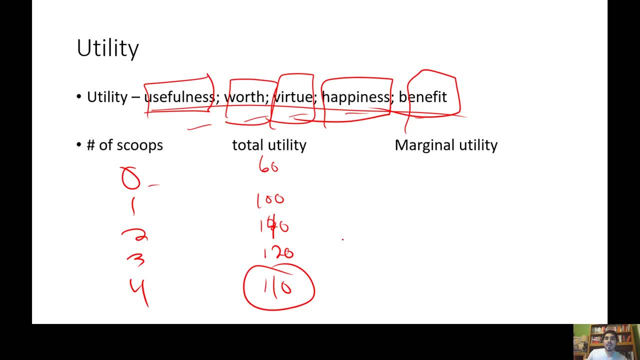 you're blowing up brownie chunks. You're just eating too many scoops of ice cream. You're not enjoying it anymore. You're becoming miserable. Marginal utility reflects the with each incremental. this should actually be 100, and then 60,, so with one scoop of ice cream. So you know, you're just. 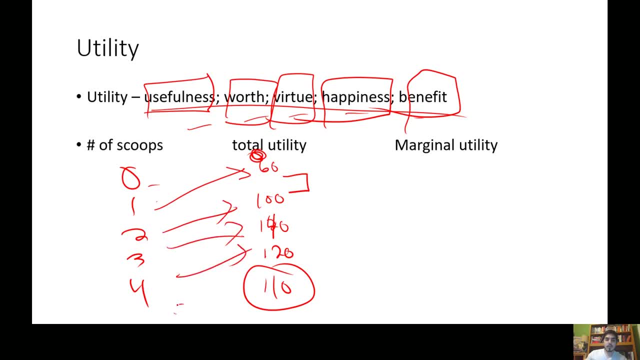 eating one scoop of ice cream, 60 utility points to 4, and then 5 is 110.. So with each increment, marginal utility reflects the utility gained at the margin or with each incremental unit. So from 0 to 60, the marginal utility is 60.. From 60 to 100, the marginal utility is 40.. 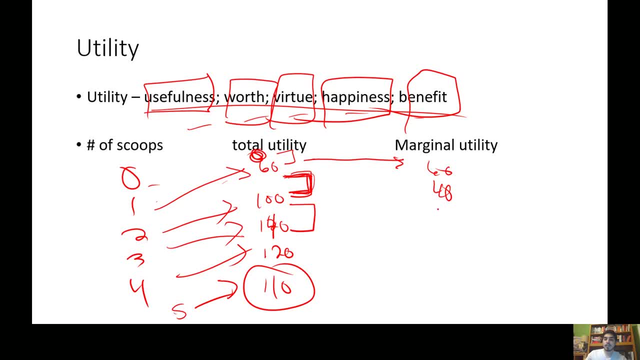 From 100 to 140,. the marginal utility is 140, or, I'm sorry, 40,. again, Let's say it's, let's 130, so I can get get the point 130. to what the heck did I do? 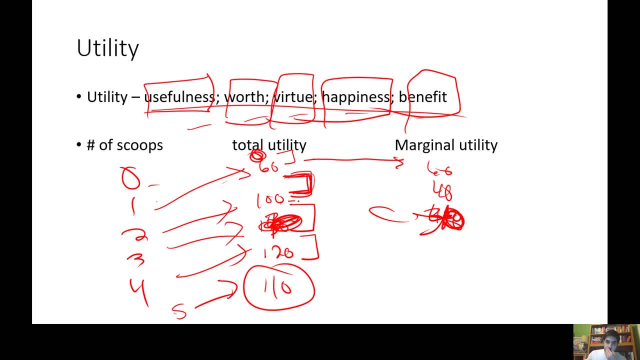 Okay, forget this. So from 100 to 120,, the marginal utility is 20, and then from 120 to 110,, the marginal utility is negative, 10, right, So with each incremental unit- And this demonstrates the principle of what is called the law of diminishing marginal utility- It represents. 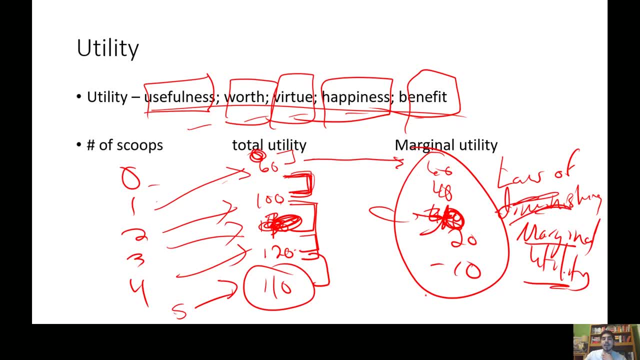 the law of diminishing marginal utility. Laws in social sciences are not exactly like the laws of, you know, physics, like the law of gravity and all that good stuff, but they are still nonetheless very important, And so the idea of 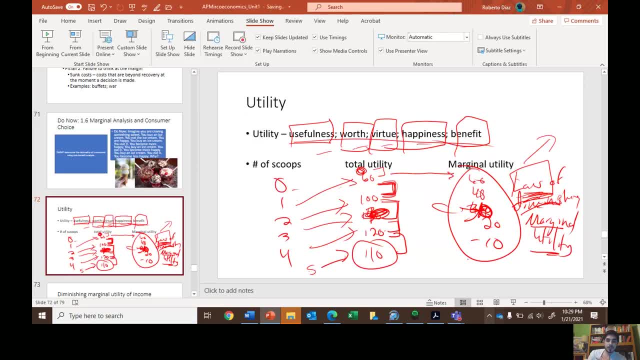 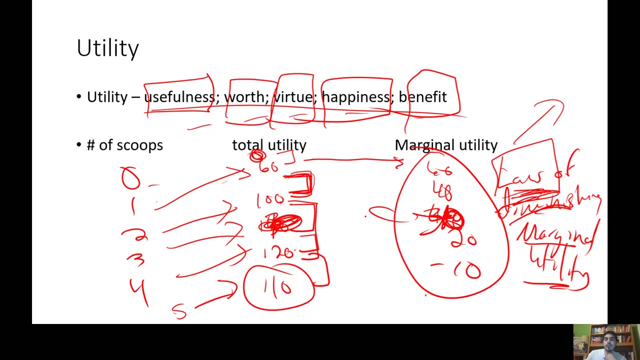 law, the law of diminishing marginal utility, is going to become very important because it's one of the reasons why our demand curves are downward sloping. that means nothing to you right now. it's going to become very important to you later. but it's this idea that with each incremental unit, 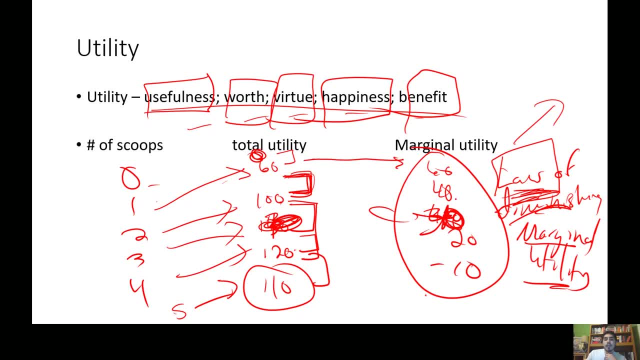 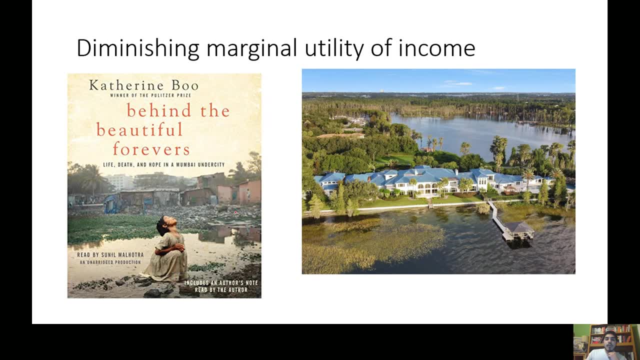 we may still gain happiness from it, but we become, we gain, our marginal utility decreases, and we should expect this um. so, for example two, we can see marginal utility. oftentimes we'll use extreme examples in economics to demonstrate a lot of laws and principles, and so we can see the 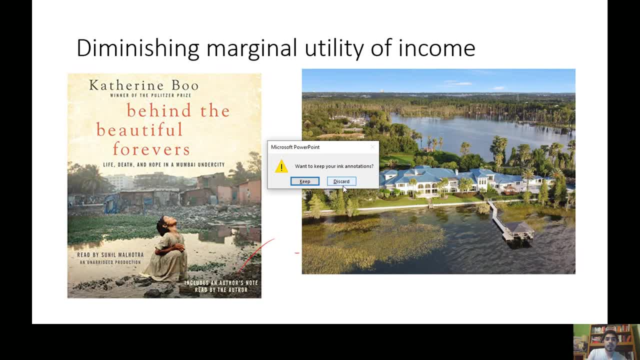 law of diminishing marginal utility in income and so, specifically, i want to show you so: in extreme poverty, the marginal utility of a dollar is probably extreme. you're probably going to be very, very happy for an extra, extra dollar. this is a beautiful book by catherine boo. on behind the beautiful 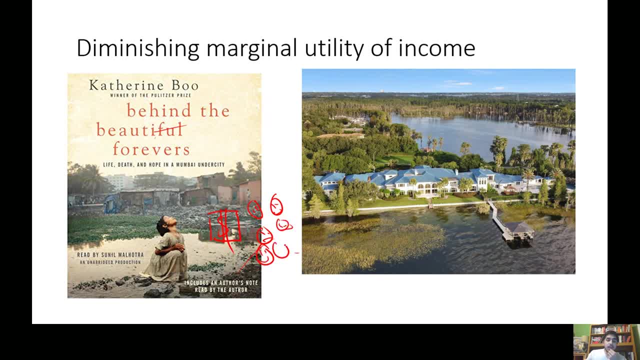 forevers about living in islam and mumbai. you're going to be really, really happy with an extra dollar- just one dollar, because a lot of these people that are the subject of catherine boo's book live on less than a dollar a day. there are about a billion people in the world that live on. 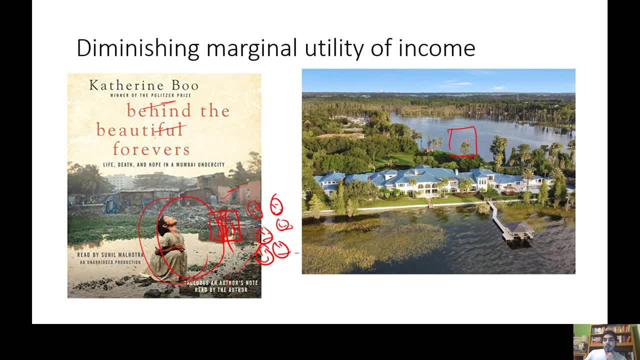 less than a dollar a day, however, shaquille o'neal- for him, a dollar is. this is shaquille o'neal's house. a dollar is not going to bring him nearly as much happiness, if anything, as as, as you know, the people that live in this slum in in india. 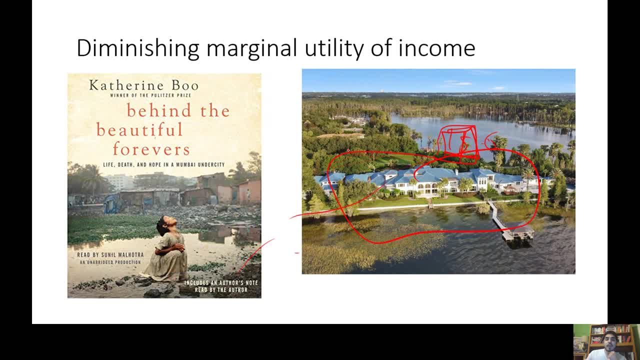 so that's the principle of diminishing marginal utility of income. there's a lot of things, for the most part, that have diminishing marginal utility and we'll we'll explore this further when we get into demand later. i also just wanted to raise your awareness, and i'm 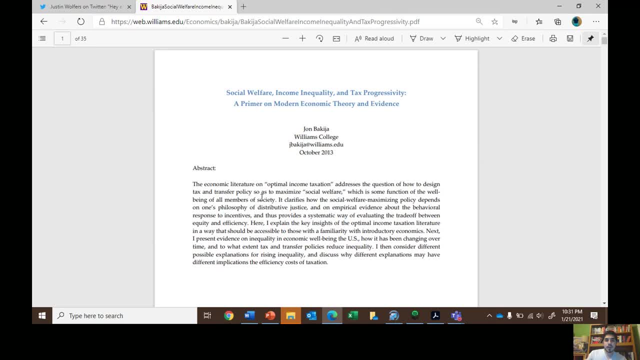 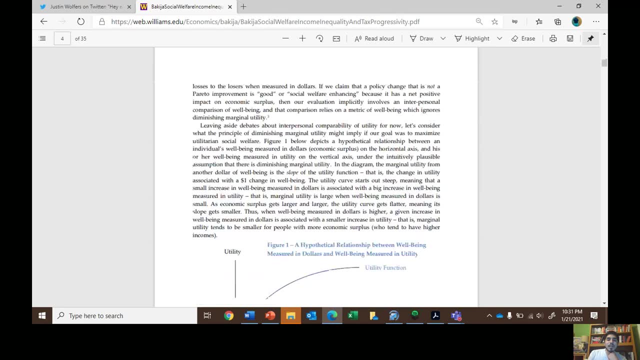 going to go ahead and share a little bit of a description. um, this is what i'm going to have my ap cohort you're going to have to read a large excerpt from this if you're in my ap cohort, depending, and this is going to cover so many cool topics. this is a really cool paper. that is really 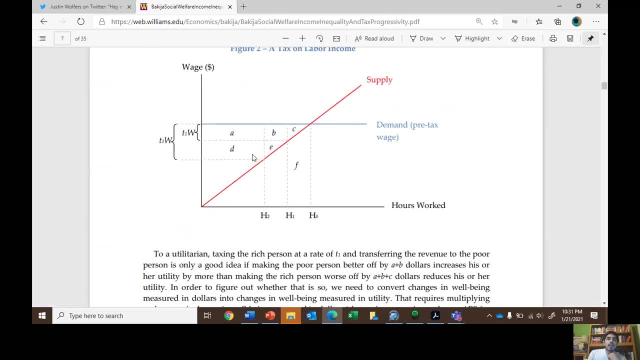 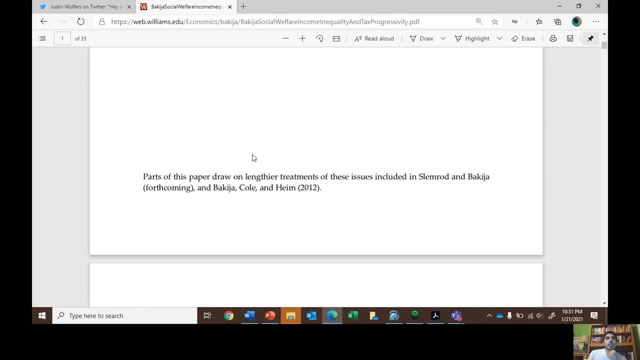 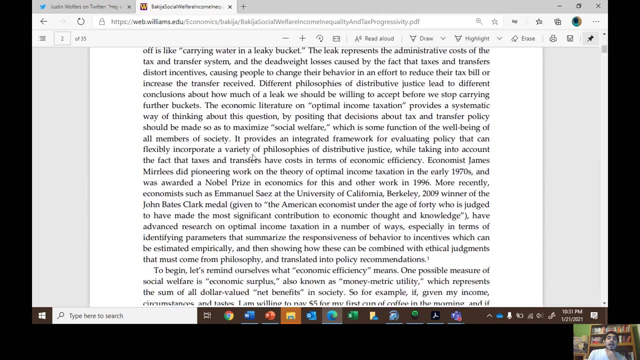 geared towards introductory economics courses in college. so, undergraduate students, that talks about the fact or talks about, you know, not our economic ideologies, but more so, um, maybe our conceptions of how to adjust economic distribution of resources. um, and i want us to kind of think about that, using 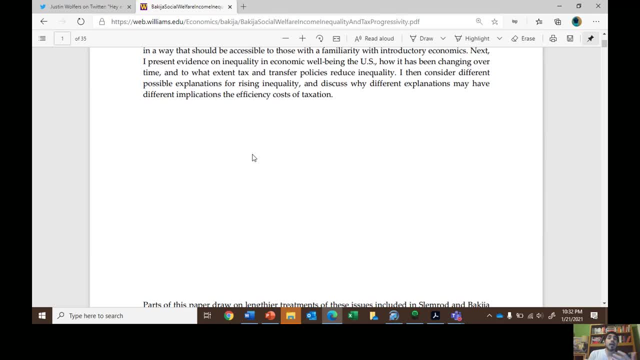 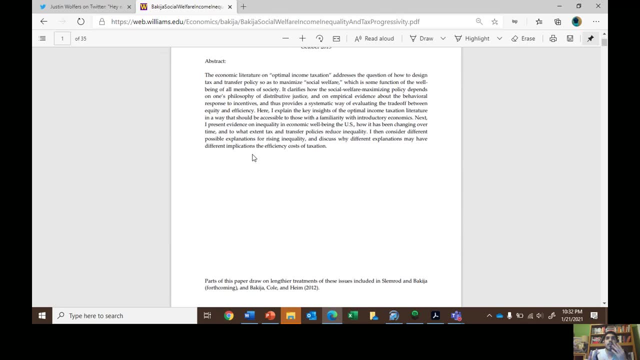 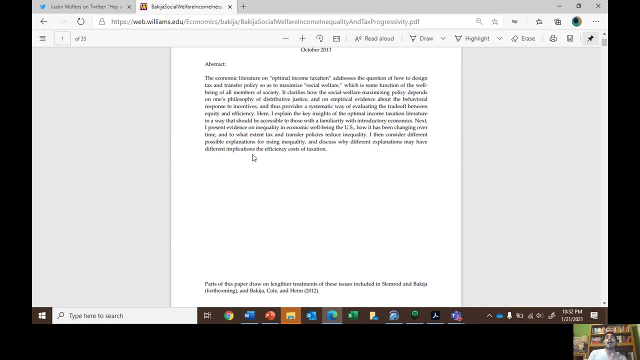 you know different frameworks for thinking about adjust allocation of economic resources, and so the law of diminishing marginal utility really suggests, um, that you know to. if you're a utilitarian in the sense that you want to increase and maximize the amount of happiness in society, um, then there seems to be a lot of room for just redistributing economic distribution of resources. 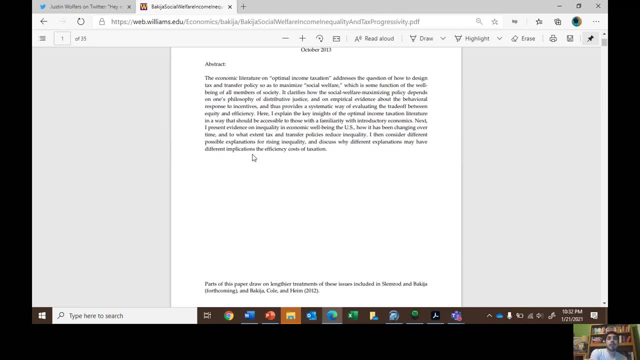 from the top end of the spectrum to the bottom end of the spectrum, where the marginal utility of a dollar is higher than at the top end of the spectrum. right, if you're looking to maximize the amount of happiness in the society, and we'll talk about this, but of course this comes with 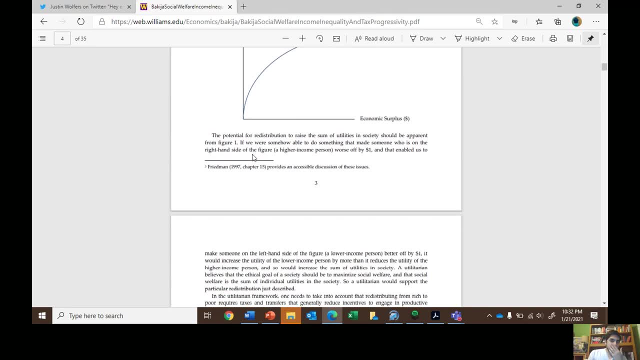 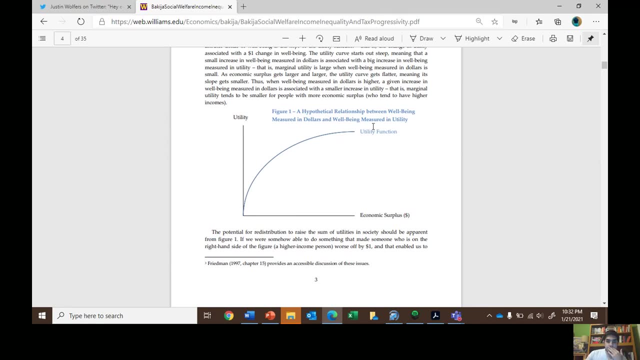 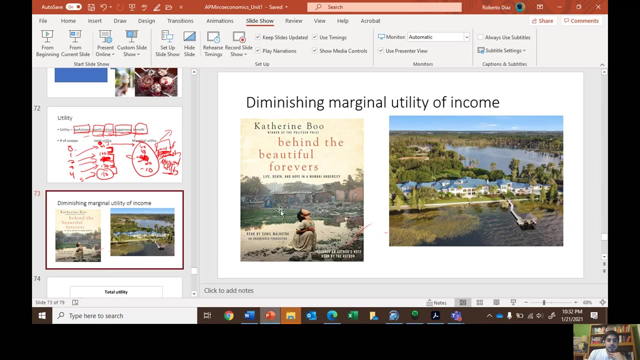 efficiency costs and there are things that we have to consider. here you can see the utility function of hyper between measuring dollars and opening measure given utility, the law of diminishing market utility. but we'll talk about this later. i just thought it was really cool to introduce and i'm very excited to talk about it. so right here you can see total utility. 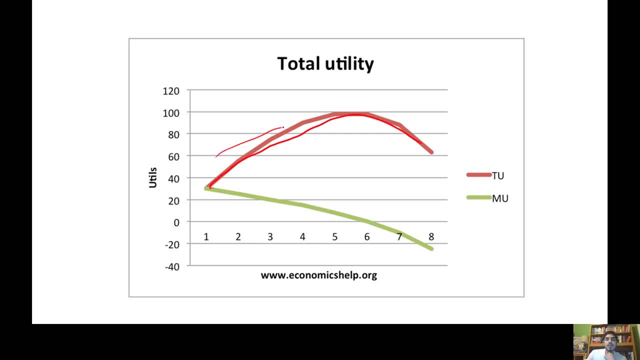 graft. we can just imagine this could be the total utility of ice cream. maybe you have at one ice cream cone, here you're blowing up trunks, or here you're you're blowing up chunks, but i don't know why you're still eating it. and then the marginal utility. so the marginal utility is actually the. 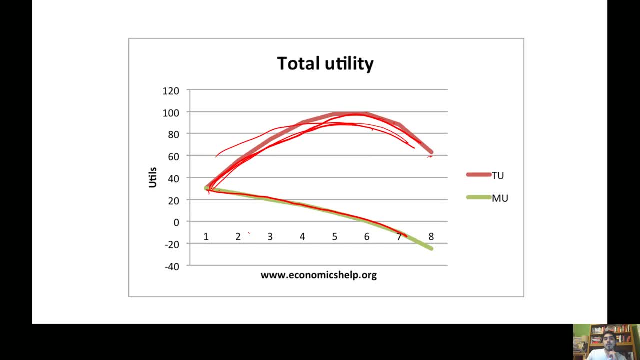 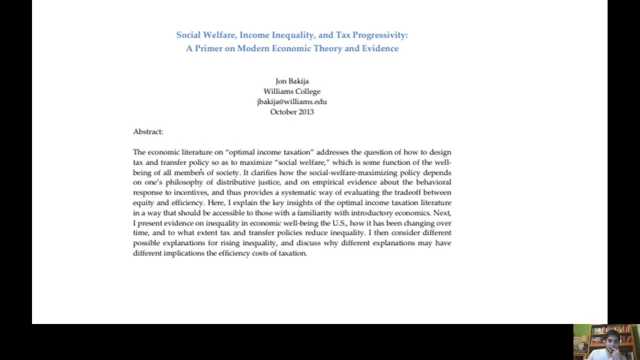 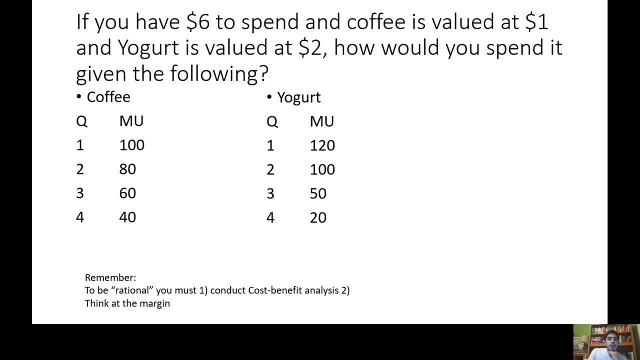 of the total utility and marginal utility, you can see, is downward sloping. this is going to be so cool because in unit two we're in a diminishing marginal utility is one of the mechanisms for a downward sloping demand curve. but i live in right now, okay, so i'm going to do this word. 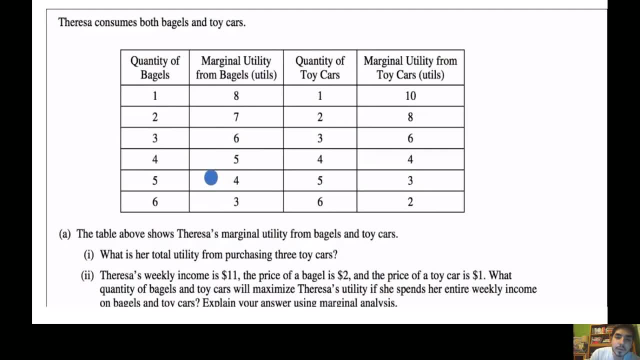 problem. the table above shows to rich teresa's marginal utility from vehicles and toy cars. so we can see the marginal utility. what is their total utility from choosing three toy cars? so we go to the amount of toy cars and we know that marginal utility is reflects incremental utility gained. so at 10 a 10, marginal utility reflects the gap between 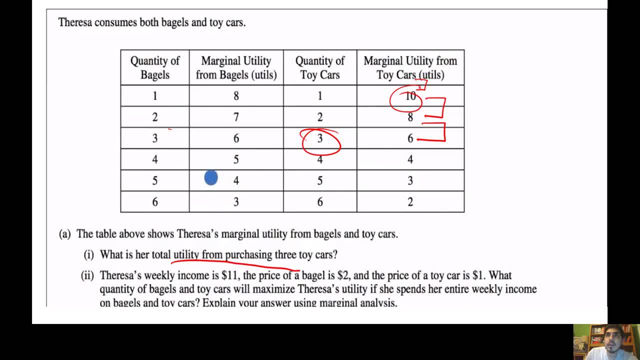 uh, quantity of cars being zero and ten, and the marginal utility or the, the, yeah, the marginal utility or the incremental utility gained from zero to one, and that's ten. um, so all we have to do is add up marginal utility to find the total utility, and so we add these numbers up, 10, 8 and 6, and we get 24.. so easy, 24.. 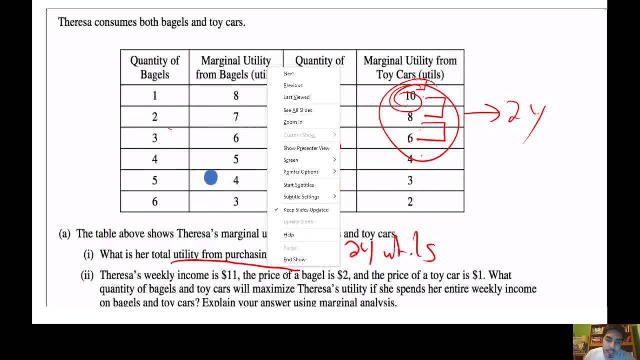 this is a little bit harder and this is where i kind of messed up in class, and my apologies. i was, i haven't been sleeping very properly and, as you can probably tell, um, you know, teaching, i've been teaching. you have to consider it from my view. now i'm feeling sorry for 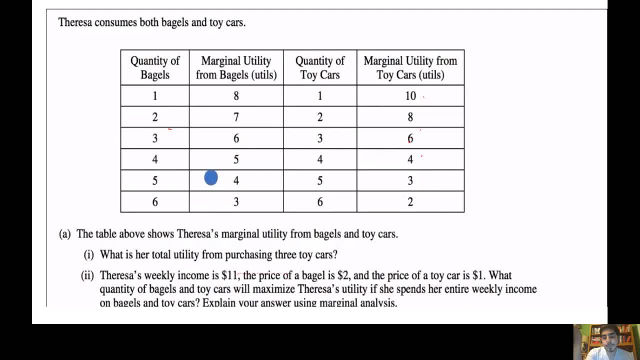 myself in this youtube video, but i have been a teacher for two years now and both years um, i decided to move to ap microeconomics. that was my decision, for sure, because i love ap micro, i love ap government and i wanted to teach it. after i taught ap world history, i wanted to teach ap world. but 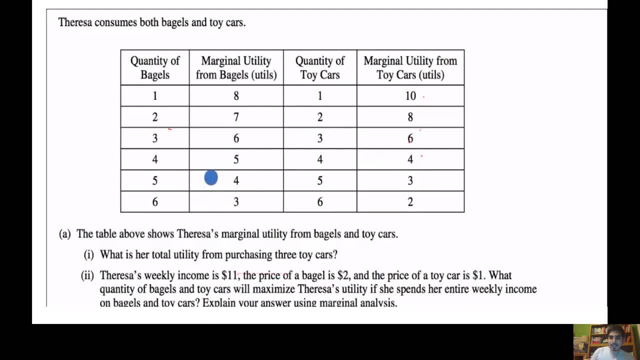 i've only ever taught a new content. does that make sense, like i've taught ap world history and then ap government and then ap microeconomics? i think i really want to stay one more year. um, because i just want to be able to like relax a bit. 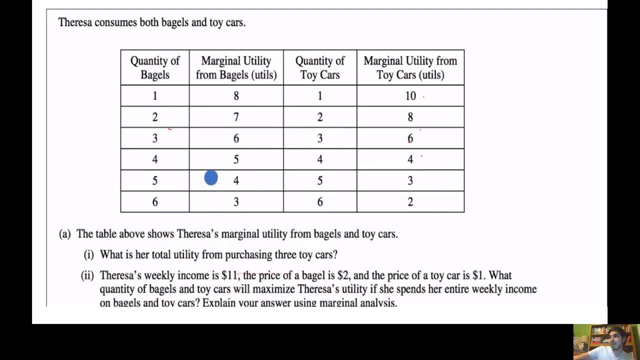 and having taught you know, or having all these resources accumulated that i've made um to be able to implement. okay, that's besides the point. so the table above shows tourist's margin utility from from bagels and toy cars. um so marginal utility from toy cars and utils. we just had a muck. 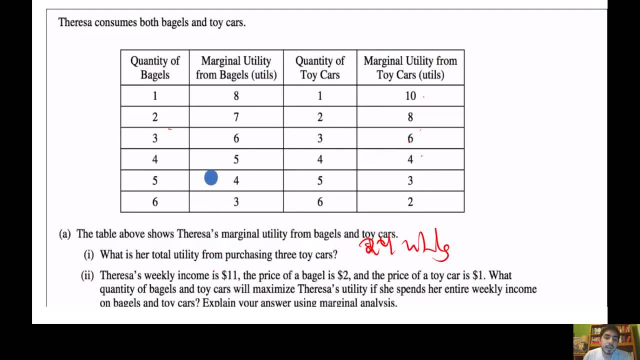 up 24.. 24 utils: Teresa's weekly income is $11,, the price of bagels is $2, and the price of a toy car is $1.. What quantity of bagels and toy cars will maximize Teresa's utility if she spends her? 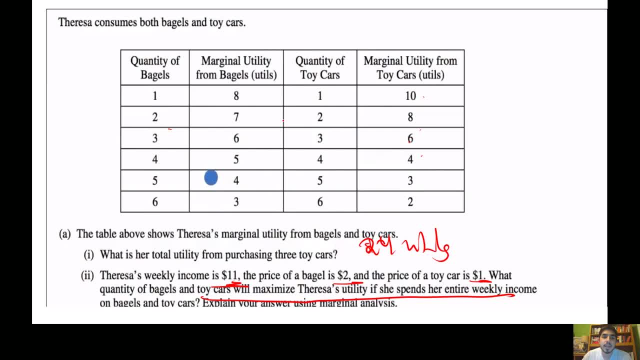 entirely weekly income on bagels and toy cars. Explain your answer using marginal analysis. Okay, so I'm not going to get to the explain this part. We're going to do that in AP microeconomics tomorrow- but we have to find to be able to compare these. 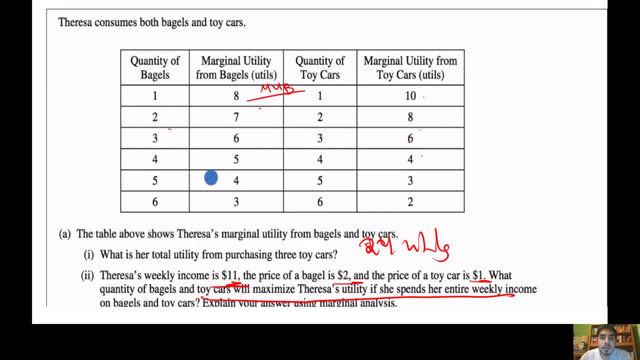 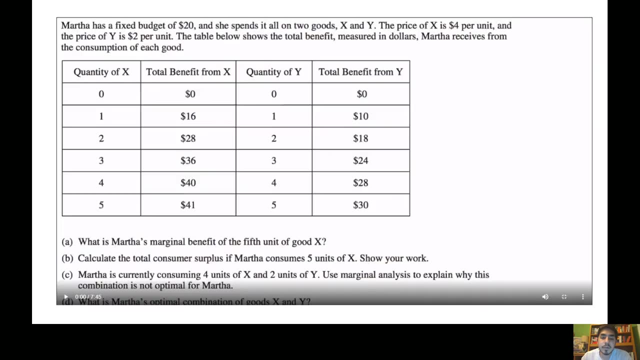 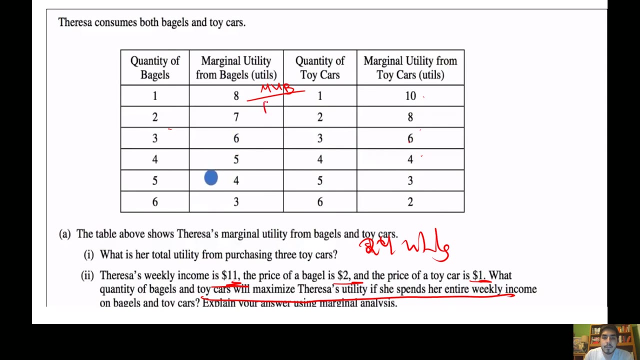 and make sure that we're allocating these $11 properly is we have to find the marginal utility per price, So marginal utility of bagels per the price of bagels, And then we have to do the same: marginal utility of cars per the price of cars. 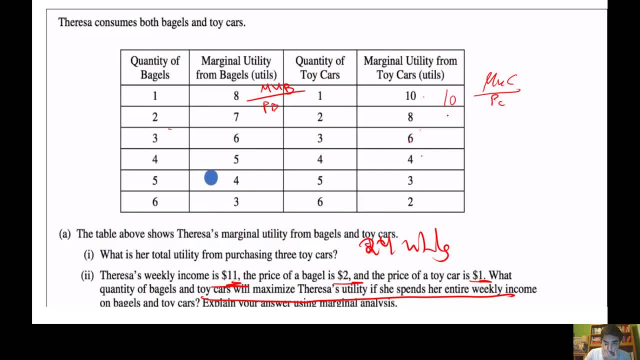 And so price of cars is only $1, so it's 10,, 8,, 6,, 4,, 3,, 2.. The marginal utility per price of bagel is divided by 2, so you divide everything by 2.. 8 divided by 2 is 4.. 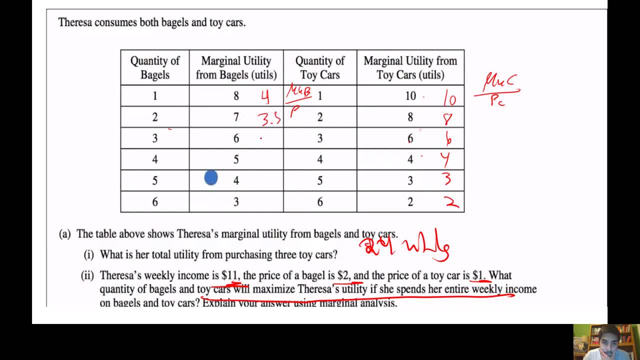 7 divided by 2 is 3.. 3.5.. 6 divided by 2 is 3.. 5 divided by 2 is 2.5.. 4 divided by 2 is 2.. 3 is 1.5.. Okay, so if we're maximizing utility, we're trying to get the most utils for our bucks. 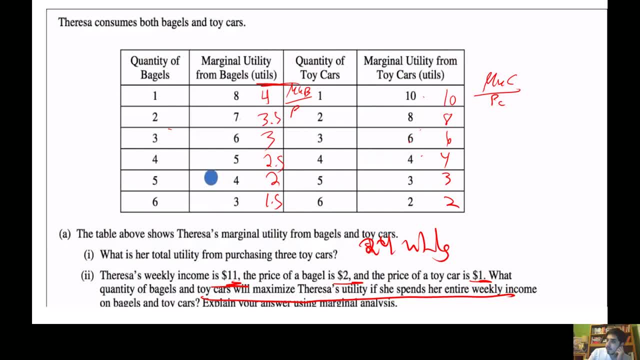 And so what we have to do- and what I forgot to do- is we have to determine: okay, for each dollar, how much are we going? So, for our first dollar, we're going to allocate it to one toy car, Right? 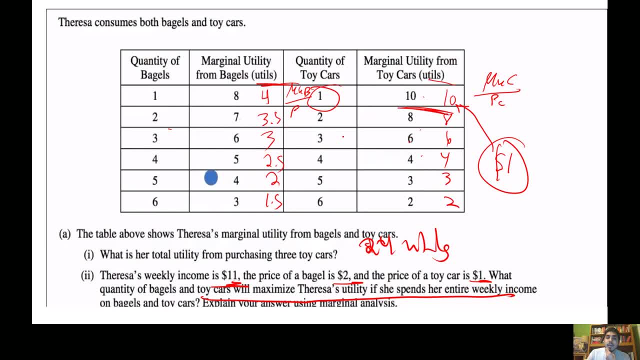 Because one toy car will give us 10 utils For our second dollar. we're going to allocate it to two toy cars, or the second toy car, because it'll give us 8 utils For our third dollar. we're going to allocate it to the third toy car because it'll give us 6 utils. 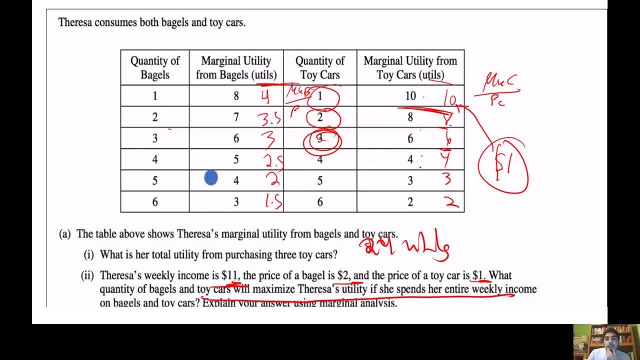 For the fourth dollar. we can allocate it to bagels or we can allocate it to toy cars, which is allocated to toy cars. to keep it simple, For the fifth and sixth dollar, and this is what I forgot to say, because the fifth and sixth dollar 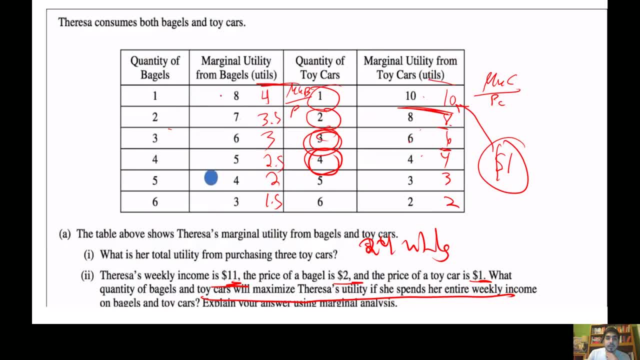 because remember that one bagel costs, you know, $2. So for the fifth and sixth dollar, I'll just put two circles or something, whatever you want to notate. we're going to allocate it to one bagel Because we know.